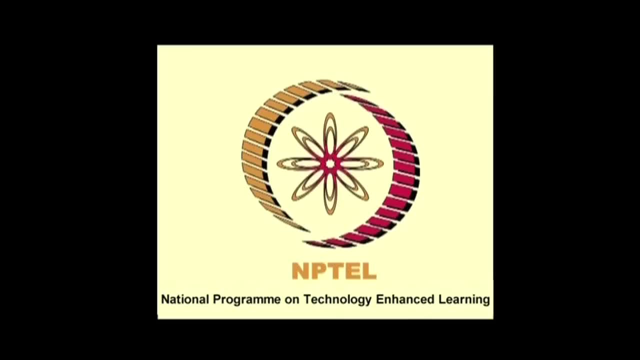 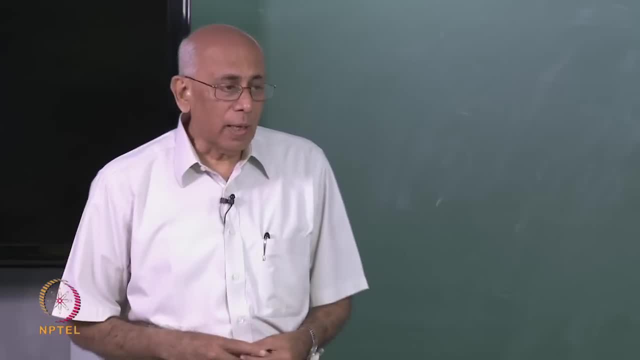 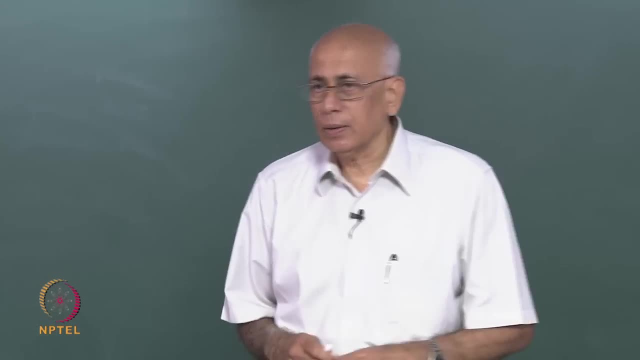 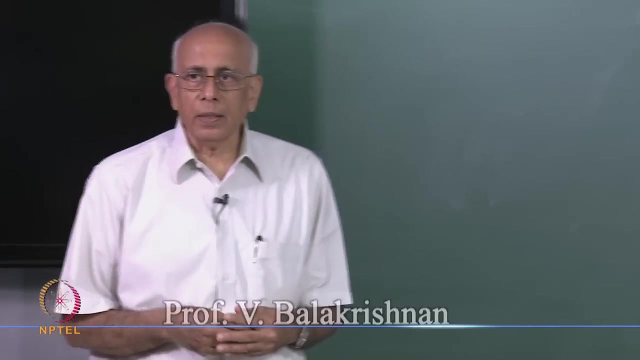 So we will start today with a slightly new topic, which is the first of the partial differential equations of physics, the famous partial differential equations of traditional physics, And this is Laplace's equation and, of course, if you have a term on the right hand side, it 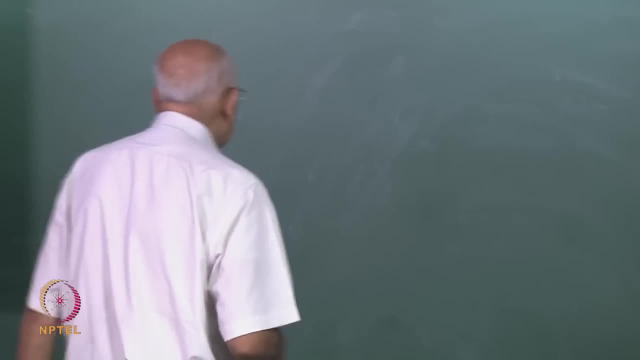 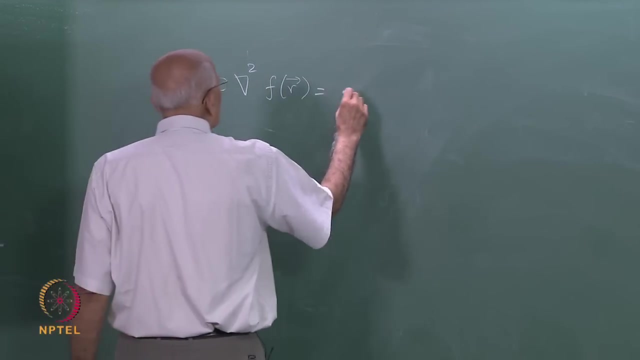 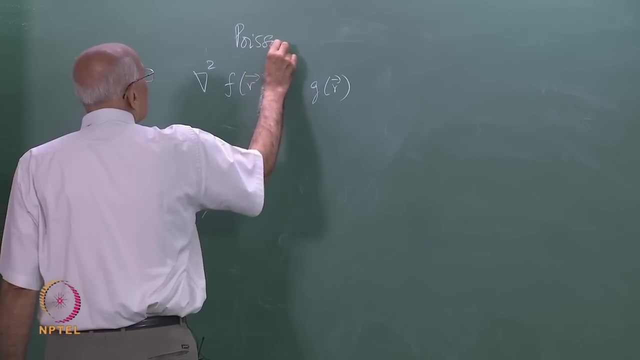 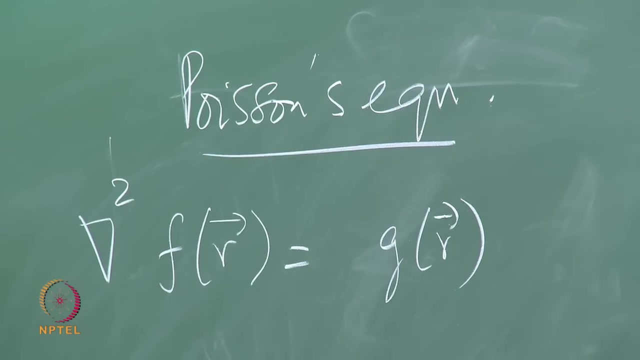 is Poisson's equation. So the equation we have in mind is of the form del square, some function of r equal to some other given function of r. This is Poisson's equation. By the way, the operator del square itself appears in all these equations. 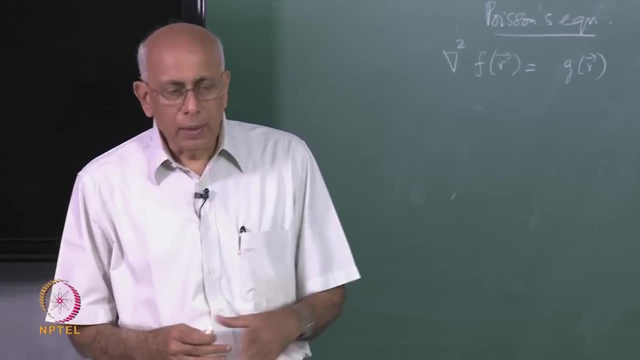 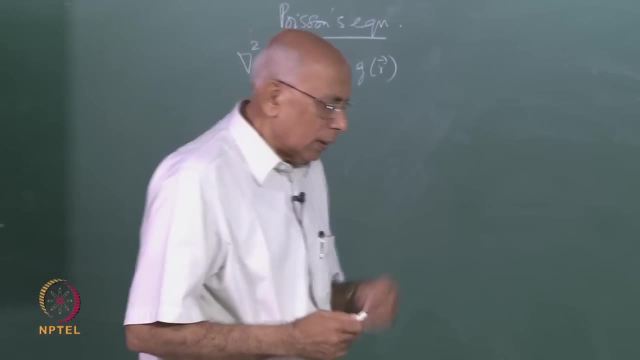 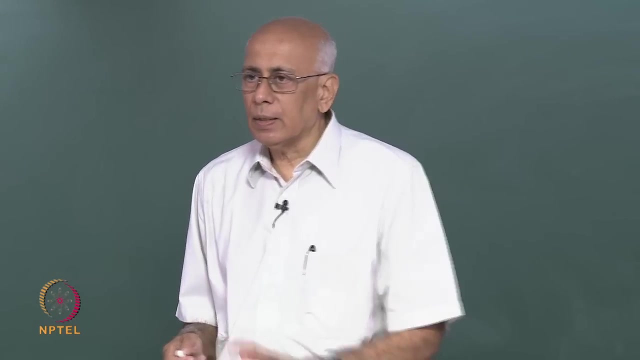 All the standard equations we are going to discuss, namely Poisson's equation, the wave equation, the diffusion equation, the equation, and so on. And there is a reason for it, of course, because del square is a scalar operator. It is invariant under rotations. 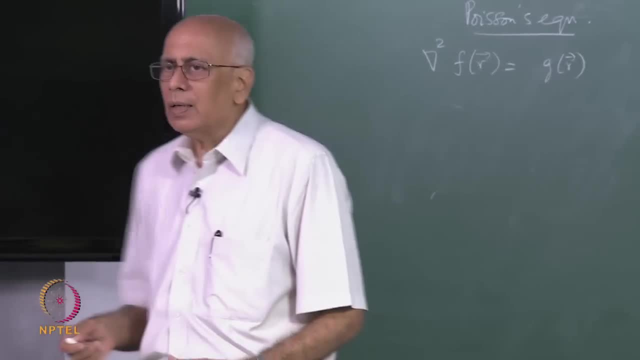 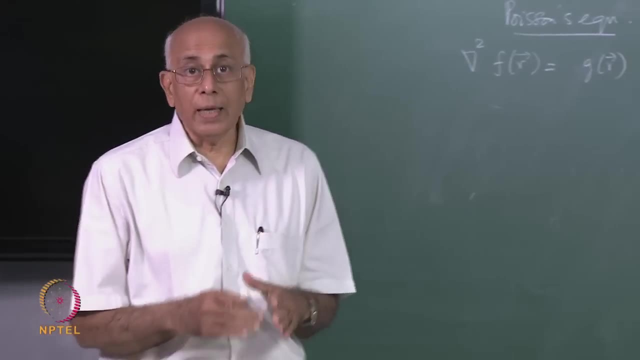 And these physical systems or situations that we are going to describe would generally have rotational invariants of some kind. So you have a second order differential operator del square, which is a scalar operator. It has a lot of fantastic properties. It is called an elliptic partial differential. 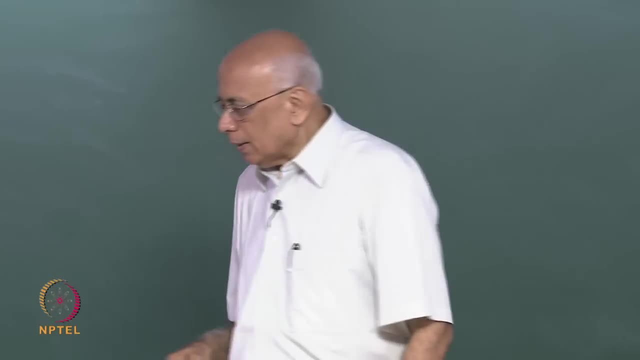 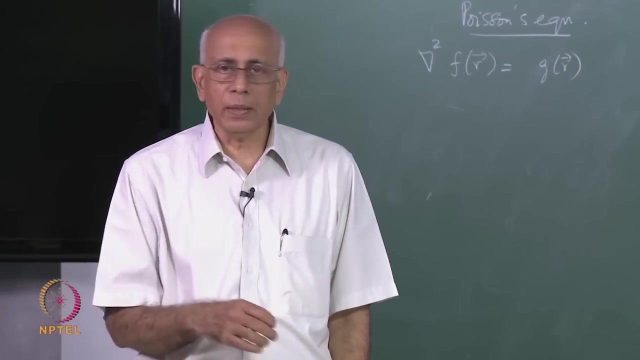 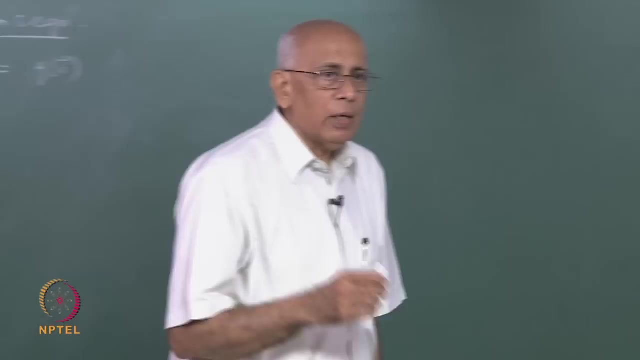 operator in the classification of such operators. And it is absolutely fundamental. When you generalize this del square to higher dimensional spaces, curve spaces, other manifolds and so on, it turns out that if you know a certain eigen value problem based on the del square, 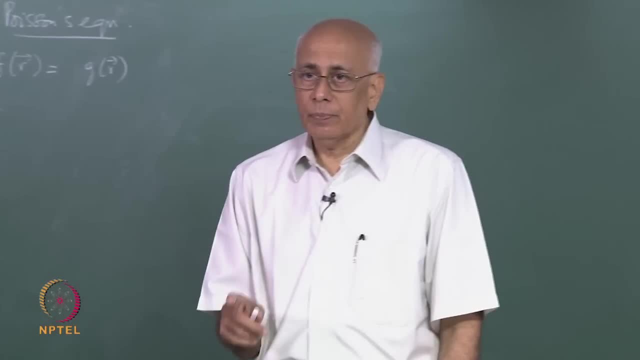 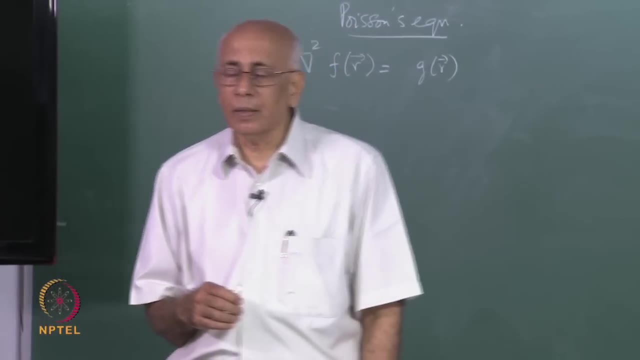 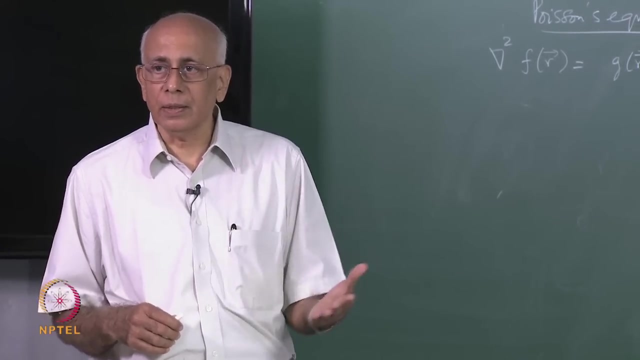 namely, very roughly speaking, if you know its eigen functions and its eigen values, then you can say a great deal about the underlying space itself. So it is a very interesting fact that knowledge of the eigen value spectrum of the Laplacian operator and its generalizations gives you a great deal of information about the underlying 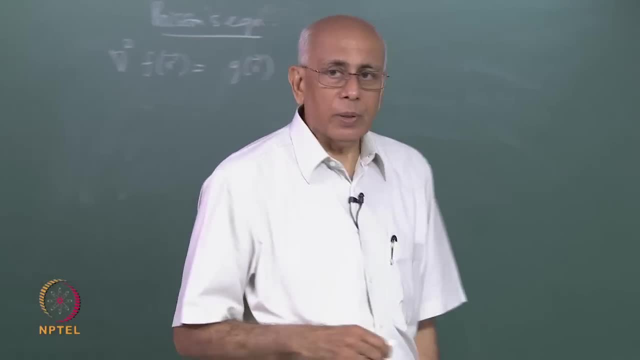 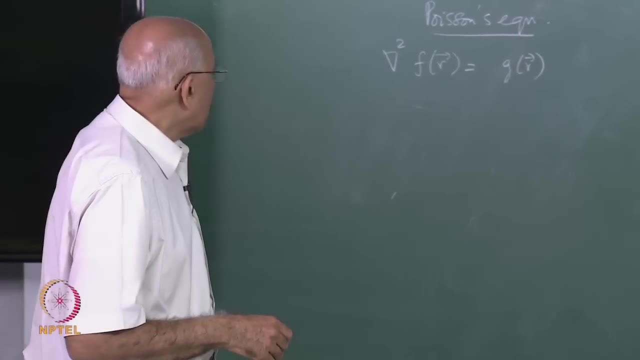 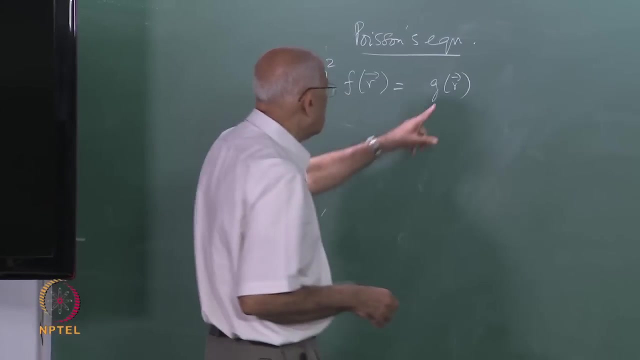 space itself. I will come back to this point later on. For the moment, we will focus on Poisson's equation, the first of these equations, And the question is: how do we solve such a, such a linear, partial differential equation where you, given some function g of r? 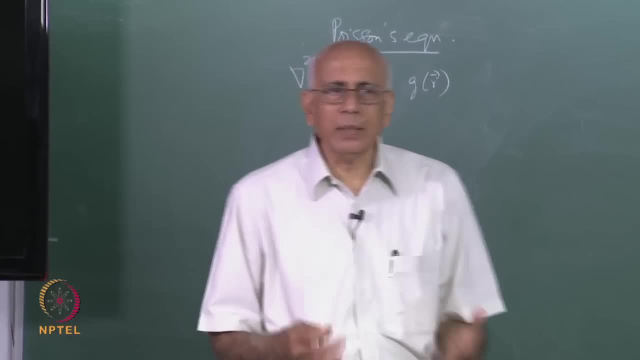 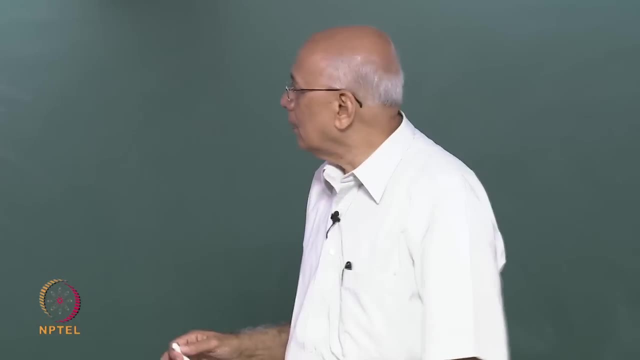 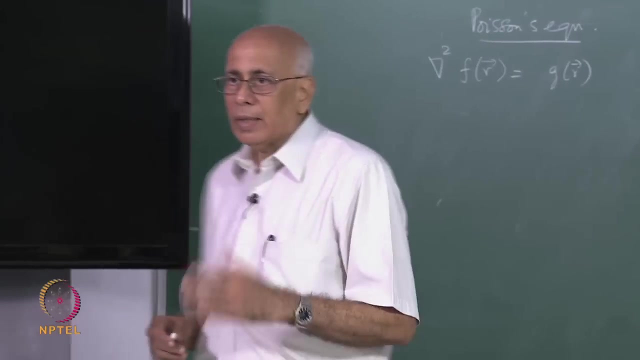 Now we will do this by a sort of combination of physical arguments and mathematics in a very simple way. All of you are familiar with this equation from the most classic example of all, namely electrostatics. where you have del square, acting on the electrostatic potential is equal to the charge density on the right. 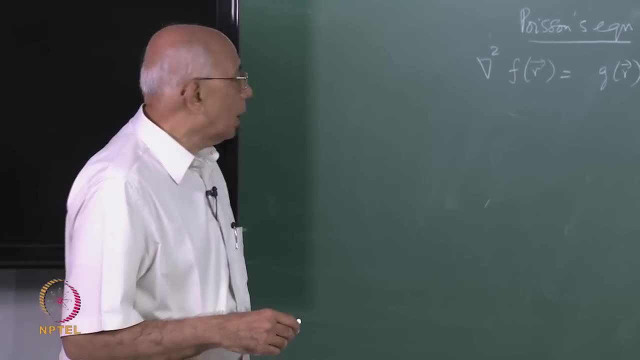 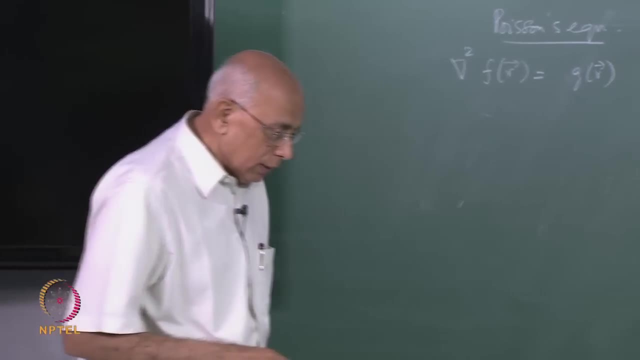 hand side, apart from a constant factor- And we know what- the solution to that is essentially Coulomb's law plus the superposition principle. that is the general solution. So we are going to exploit that fact and I will give a physical argument to see how you can extend the 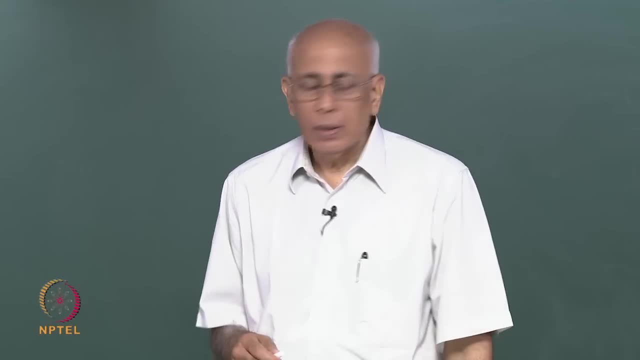 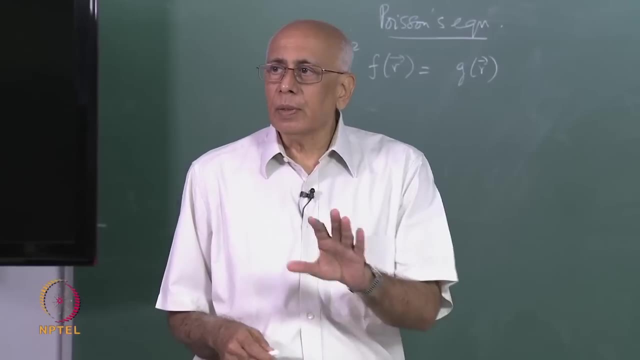 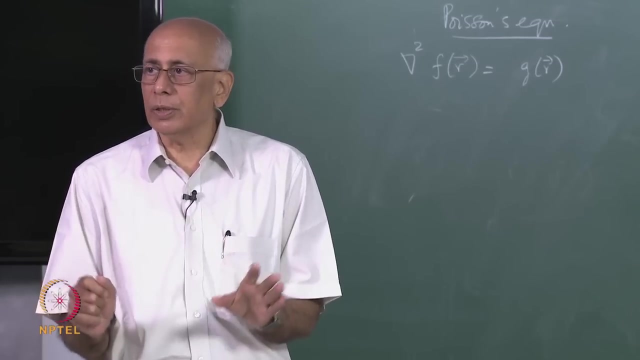 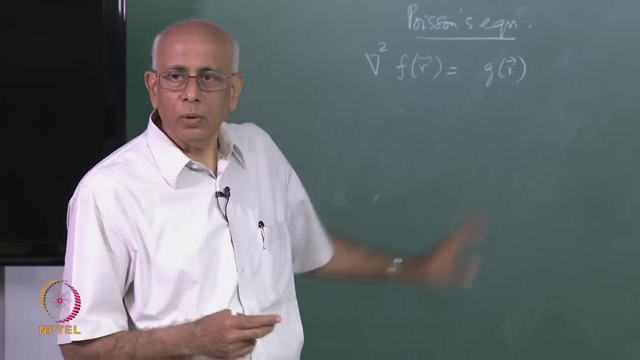 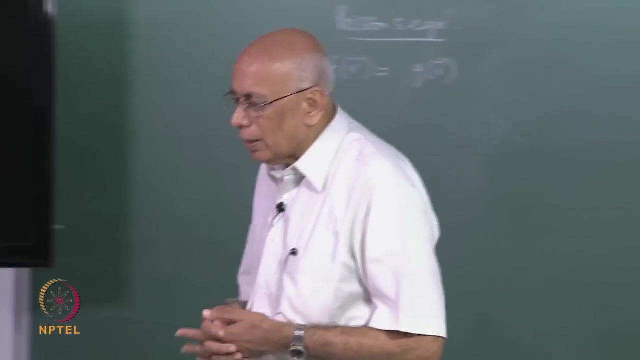 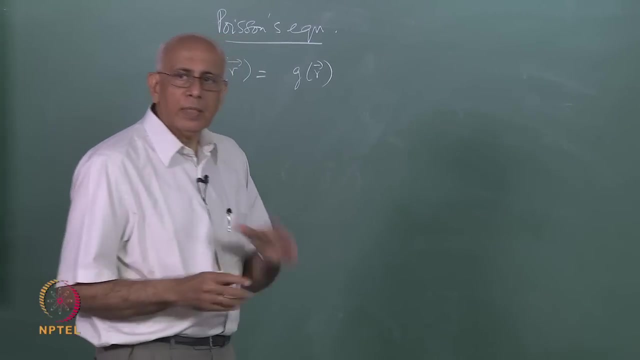 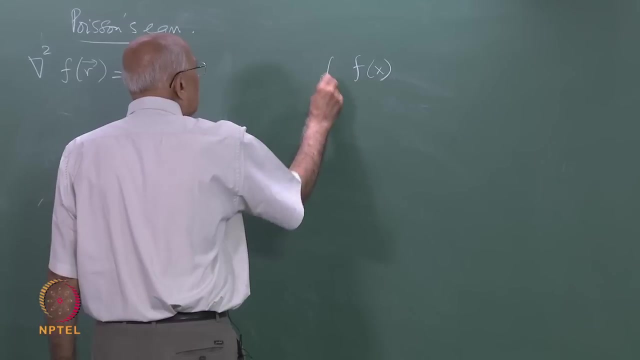 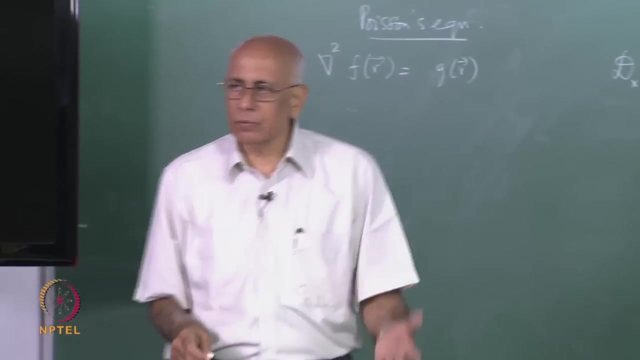 solutions of this equation to higher dimensions and so on. But the purpose here is restricted for all these partial differential equations. My primary aim is to find the so called fundamental solution to this equation, namely the fundamental green function for such operators. So this is called x functions of x, derivatives with respect to x, and so on and so forth. 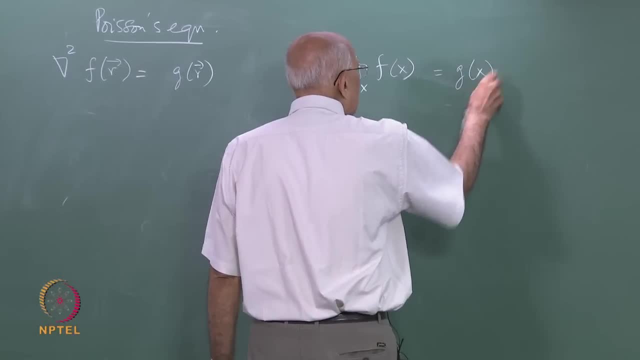 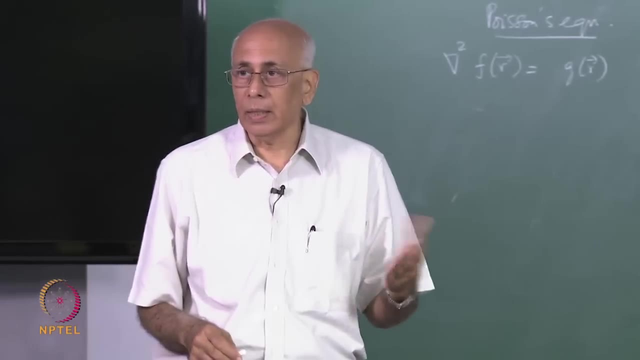 Acting on this, f of x is equal to some other function. g of x on the right hand side, a given function here. And the question asked is: what is the solution to such an equation and inhomogeneous equation? The answer is, of course, that you need to formally invert. 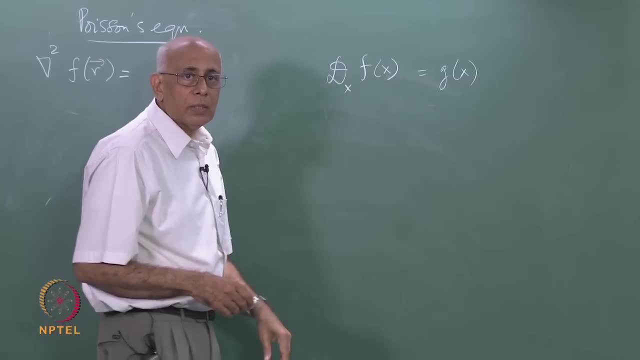 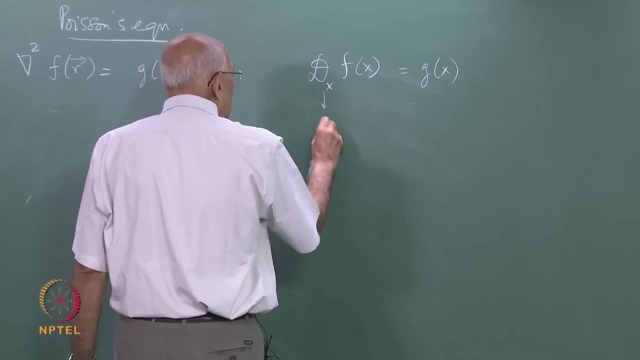 this operator and somehow get it to act on this g here. So let us do this in abstract notation and see what it looks like. So in abstract notation, if this d is a representative of some operated d in some space, some, 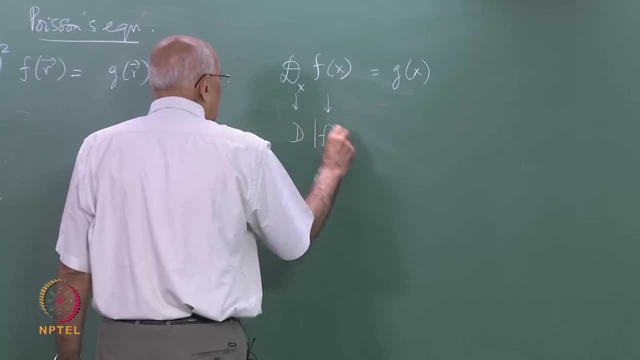 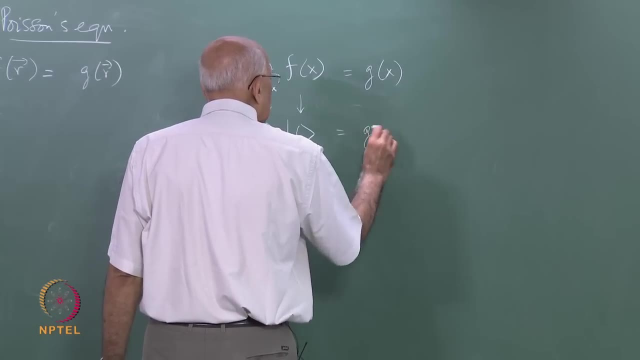 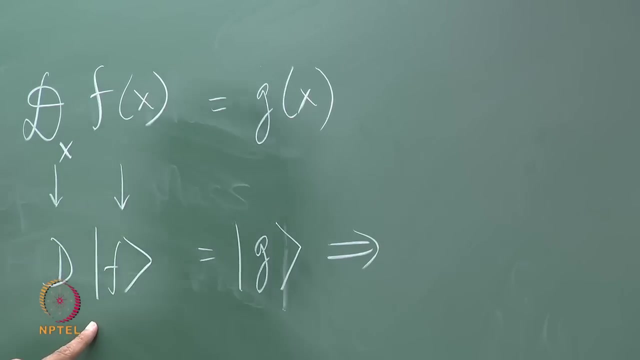 linear space and this f is represented by this ket vector on this space. I will use Dirac notation here. This is equal to g on the right hand side. This will imply formally that the solution f is equal to d in this space and this love is equal to g on the 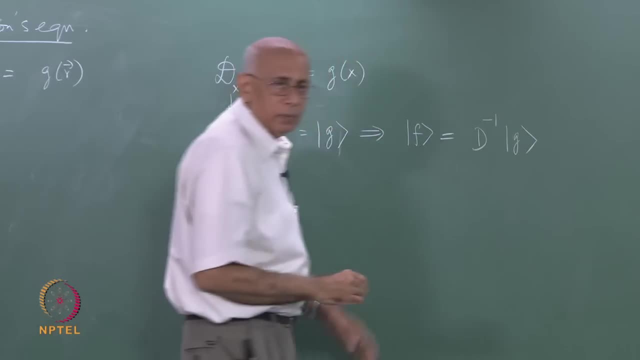 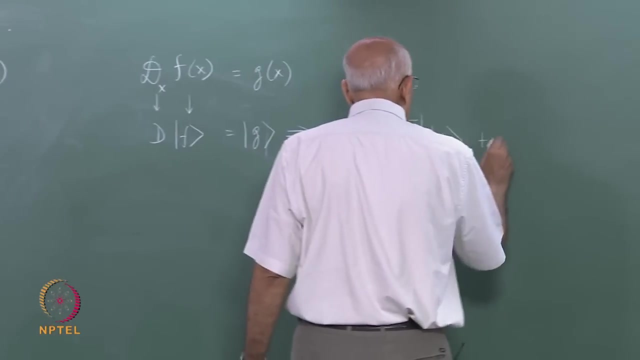 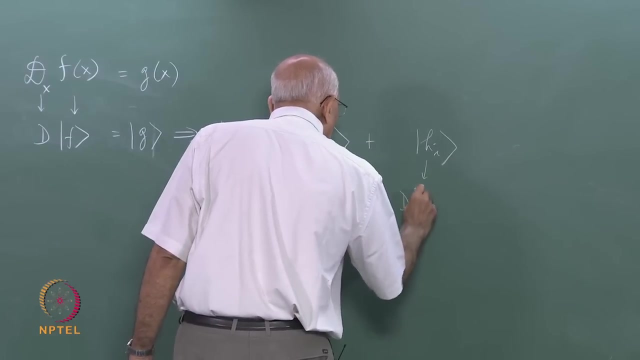 inverse, if it exist, acting on g, formally of course. but that is not all, because you could also have a piece plus a piece, which is some vector h i where d acting on this h i equal to 0, and in fact you must sum over linear combinations. 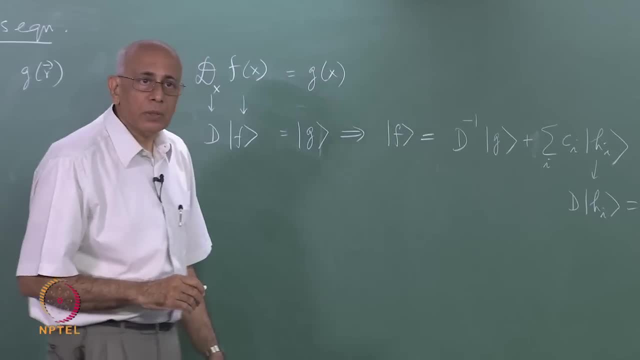 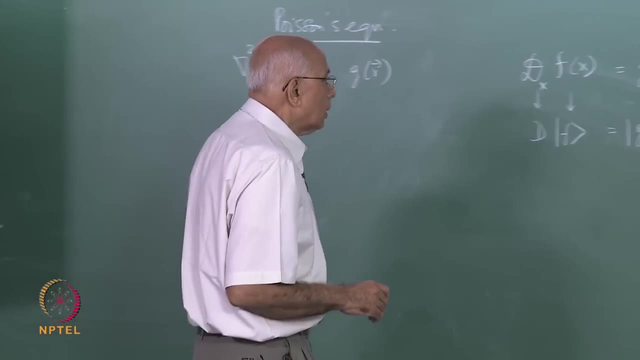 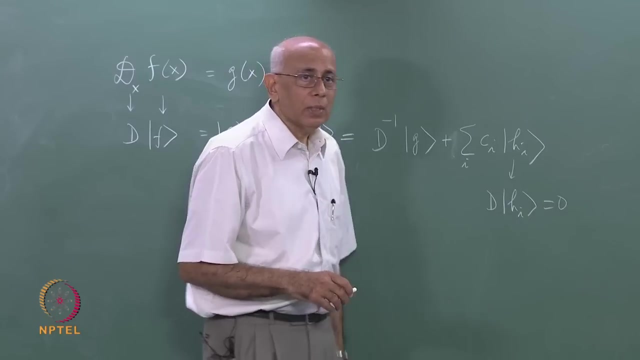 of all such Eigen functions or Eigen states such that if this operator acts on it, it annihilates it. you get 0 here. So, as you can see, this is the solution of the homogenous equation d of x acting on some. h of x is 0, and this is the part that comes from the 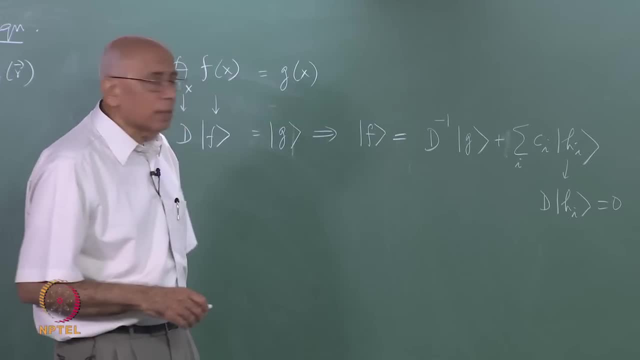 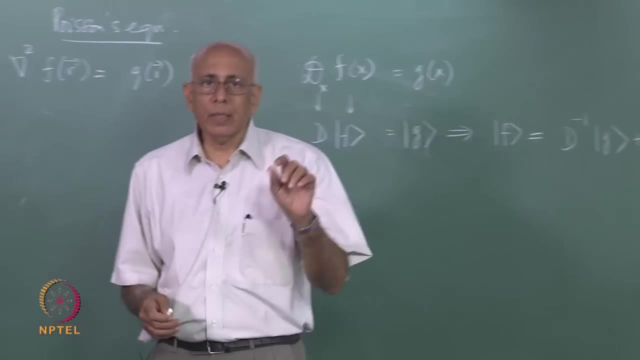 inhomogeneous equation here And in the language of differential equations, this portion, when you write it back in function space, this portion is what you would call the particular Integral and the rest of it you would call the complementary function. Now, of course, 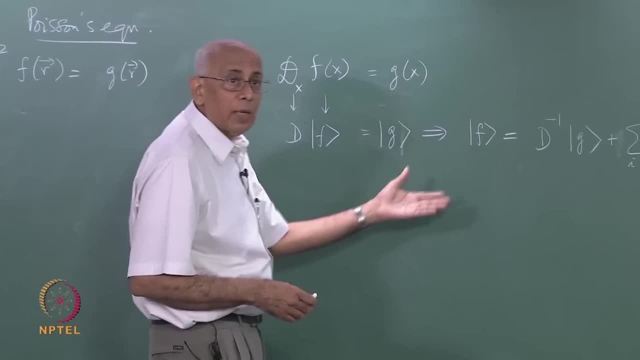 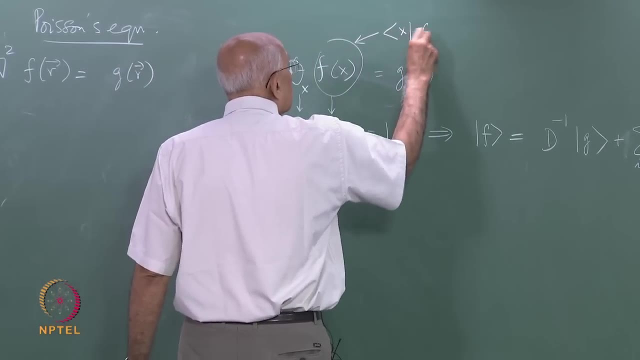 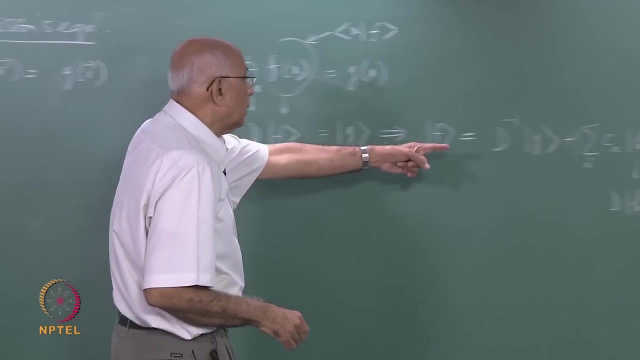 we can write this back in the position space and see what happens here. but remember that this so called f of x is nothing but the representative of this ket vector in the x basis. if you like it stands for that, Then what is this equation really look like? it says f of x equal to, and thus some operator. 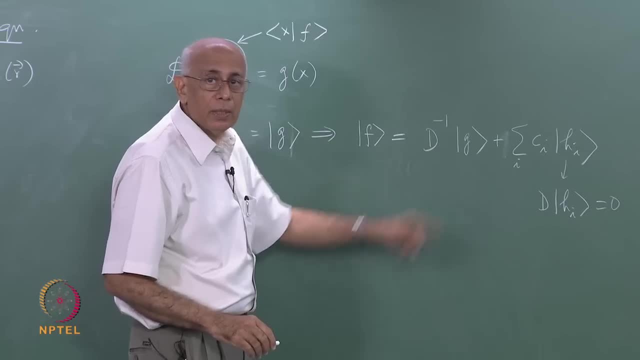 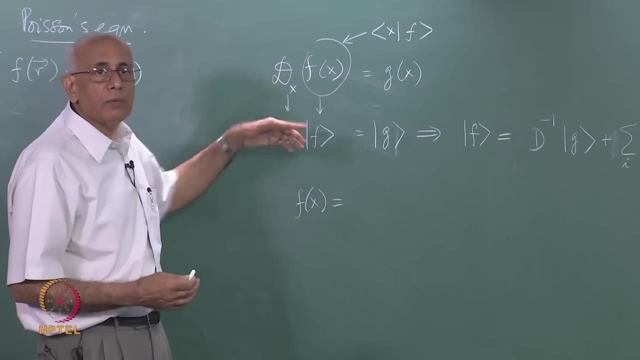 g acting on a, d inverse acting on this g. And now we can ask very naive terms. we can see what is going to be. this is a differential operator of some kind, So the inverse of it in general will be an integral operator in general. So this in would be of the form: 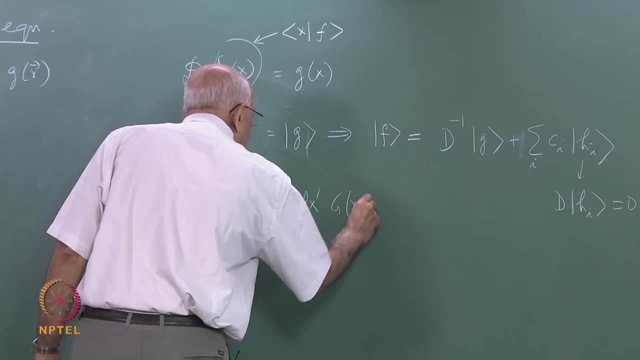 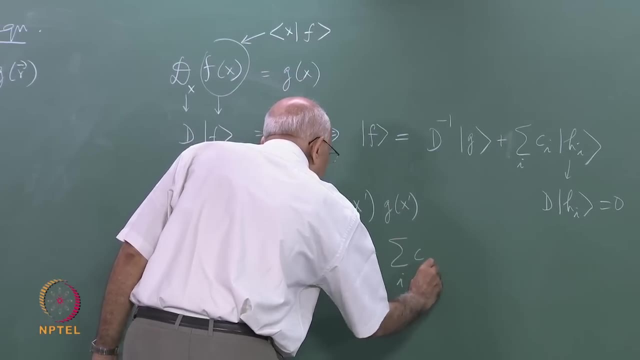 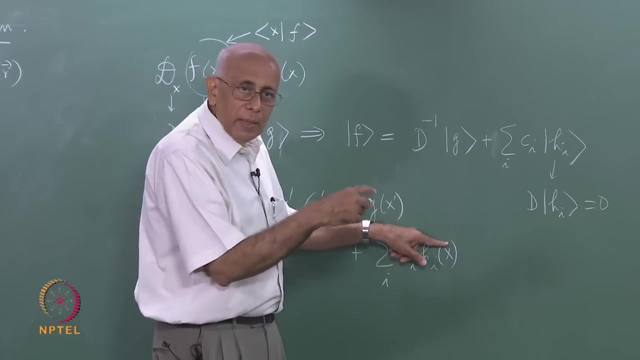 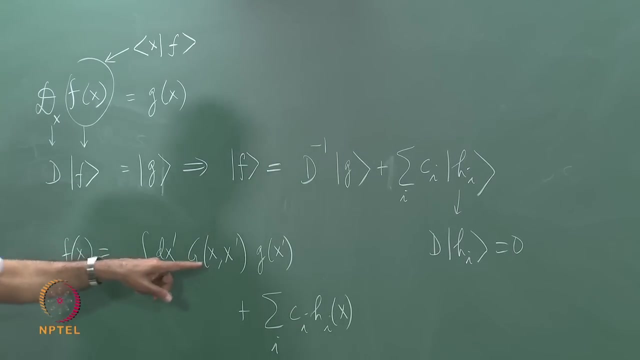 and integral over d, x prime, some g of x comma, x prime, little g of x prime, plus of course summation c, i, h, i of x, Where these are the representatives in this basis, x basis of this abstract vectors in function space. So this g here represents this d inverse. in fact we can make it even 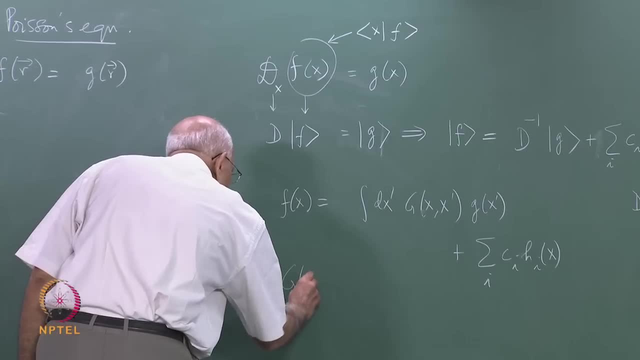 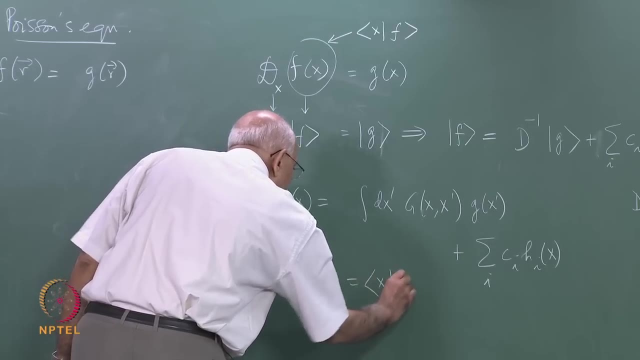 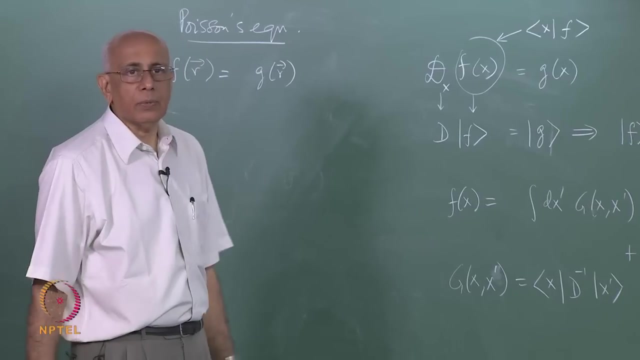 more precise, what is this g of x comma, x prime, the so called green function for this differential operator? this thing here is nothing but x d, inverse, x prime. It is obvious from this notation that that is precisely what it is. I leave you to figure. 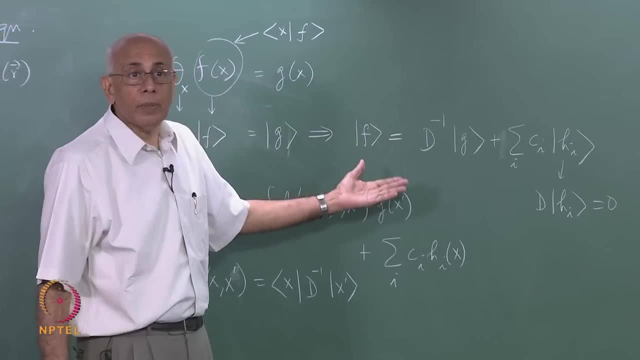 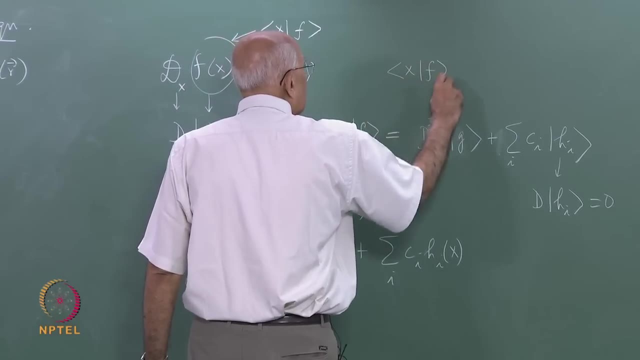 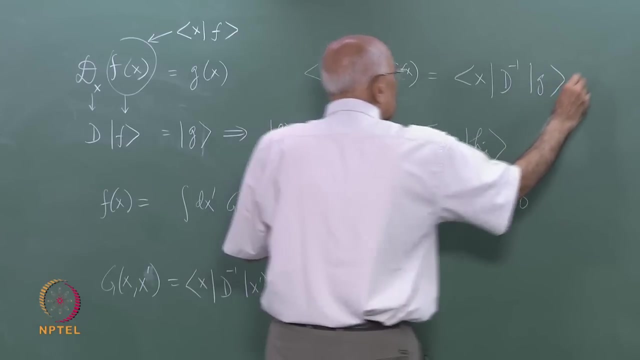 this out. I mean, it is very trivial. do you want me to do this? see how it is done. put an x on either side, So you get x, f that is equal to f of x that is equal to x. and then there is a, d inverse g plus summation over i, c, i, x, h of y. This is: 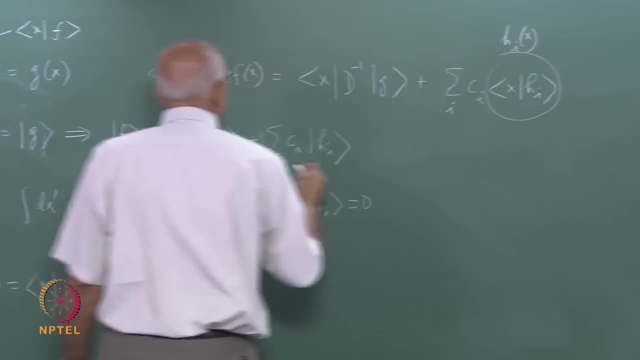 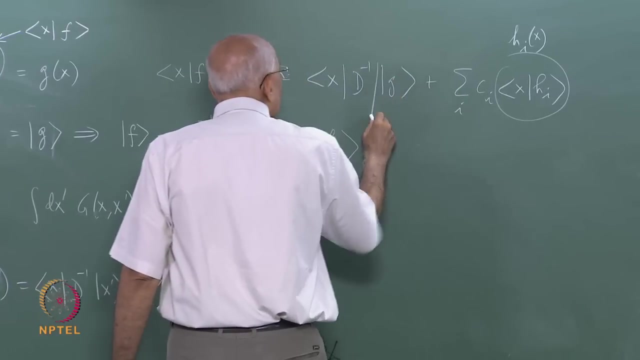 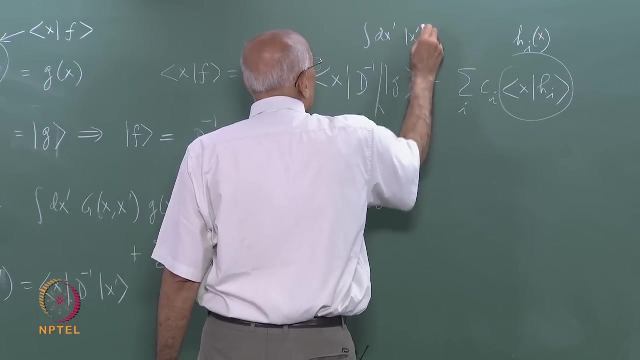 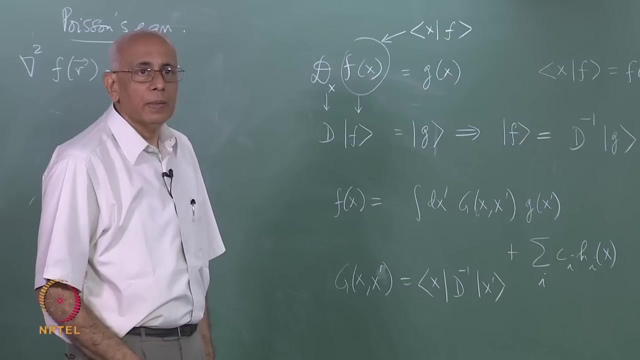 is what we called h i of x. So that is what this thing is. and here now insert a complete set of states. and a complete set of states is integral: d x prime, x prime, x prime. that is the identity operator. I insert it in between. 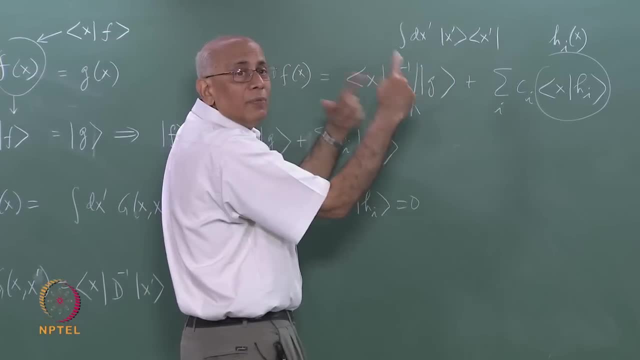 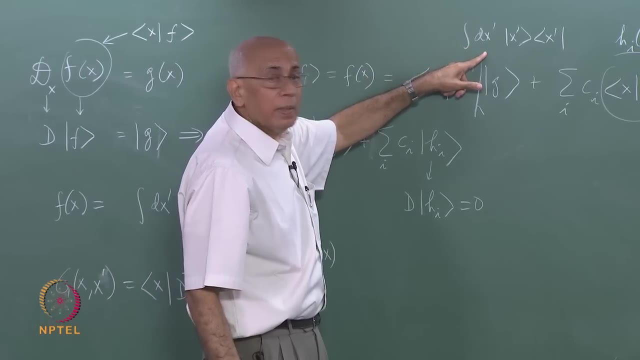 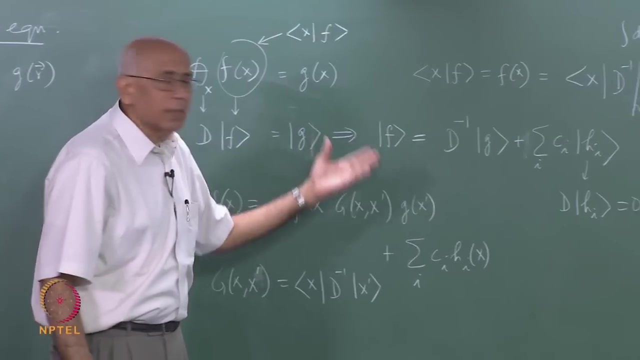 and then, of course, I get x, d, inverse x prime, that is a function of x and x prime, which we call g, the green function, integrated over d, x prime, and then x prime acting on g, that is g of x prime. So this is all it is writing. 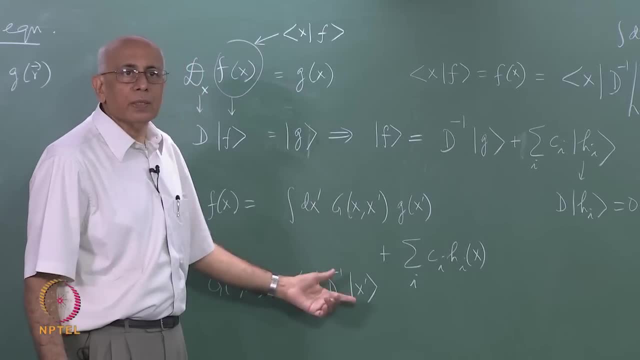 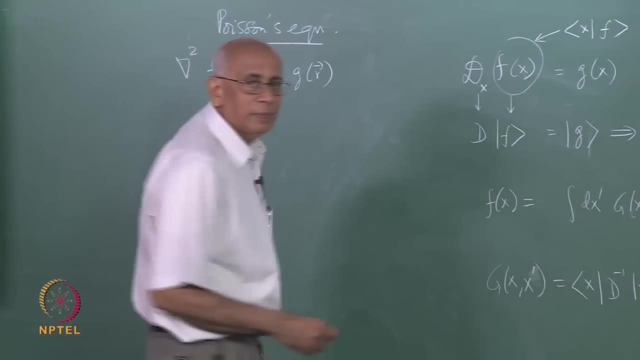 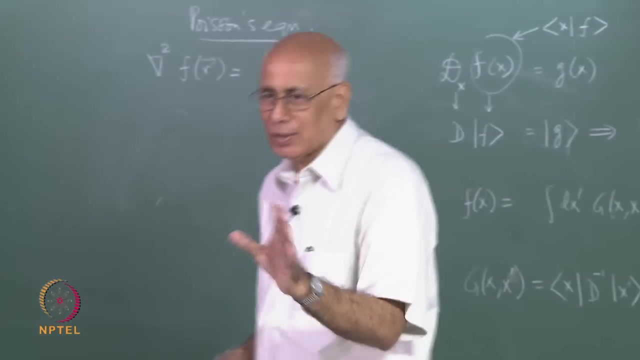 it down. this abstract notation is trivial, writing it down. here is just one more step. take the matrix element between x and x prime and that is it. Yeah, we have to certainly worry about d inverse exist. So if it exist, then this is: 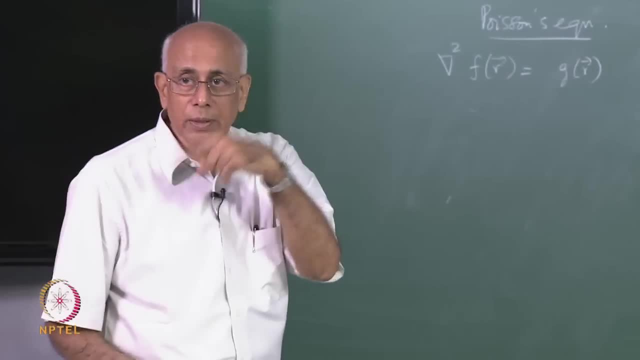 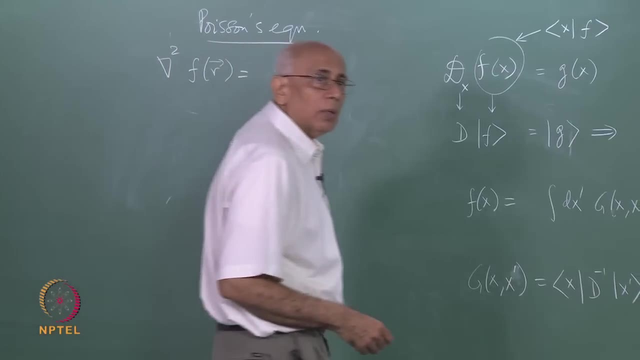 true. So we will have to ask: what are the conditions under which this d inverse exist, etcetera? and what I am going to do a little later, when we talk about integral equations, is to show you under what conditions you would have this inverse exist for this operator for the moment. 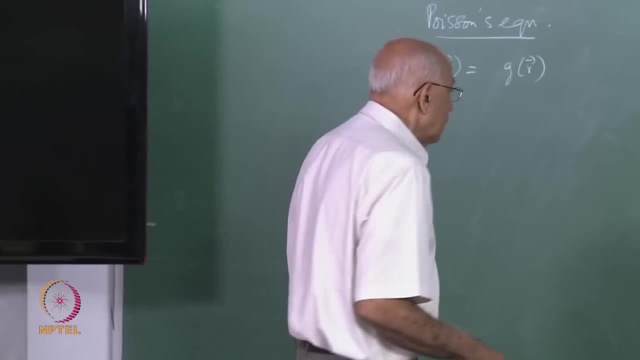 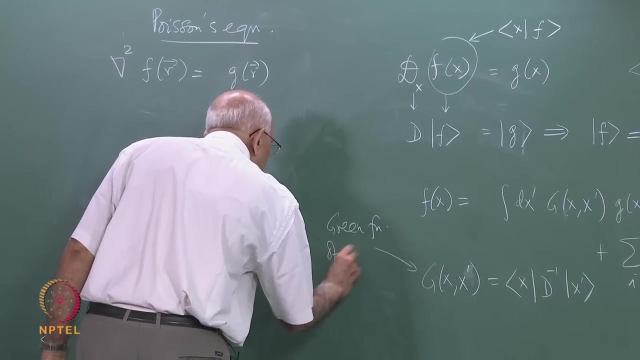 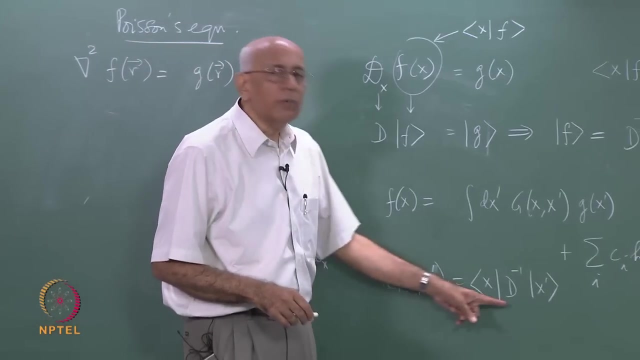 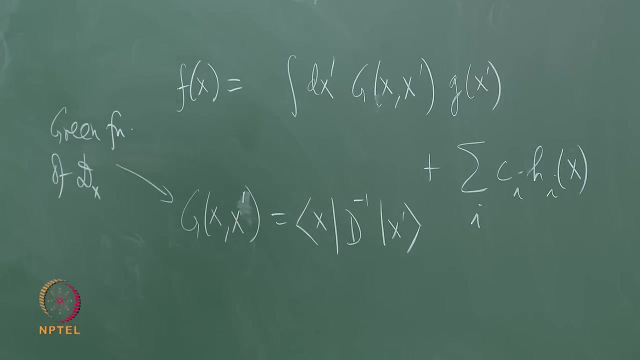 we assume it exist. So this thing here is called the green function. So this is the differential of the differential operator d x. it is nothing but the inverse of the operator expressed in this basis. nothing more than that. and we need now. 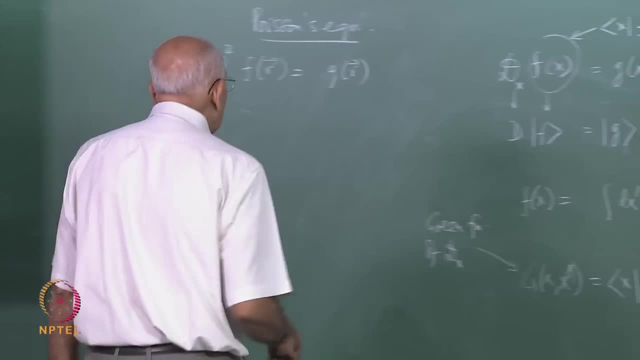 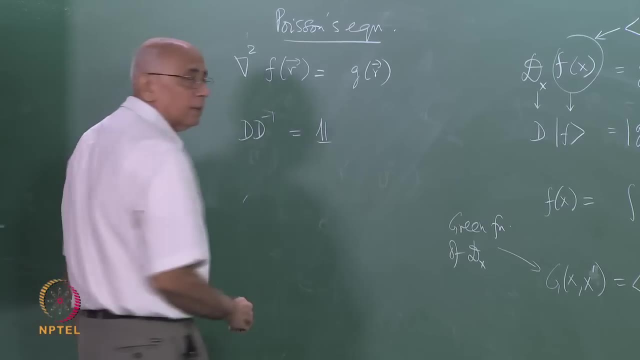 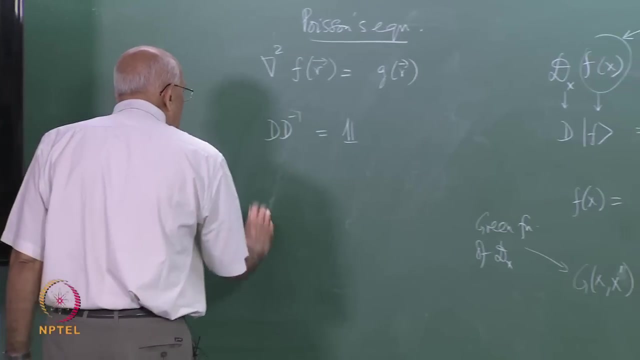 to find out what this d is. but that is very simple. we need an equation for this g. that is not hard to find, because notice that d- d inverse- must be equal to the identity operator. And if I express this in the position basis, what is going to happen? this thing here is: 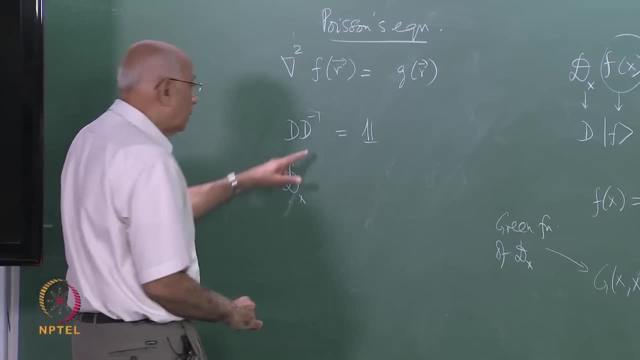 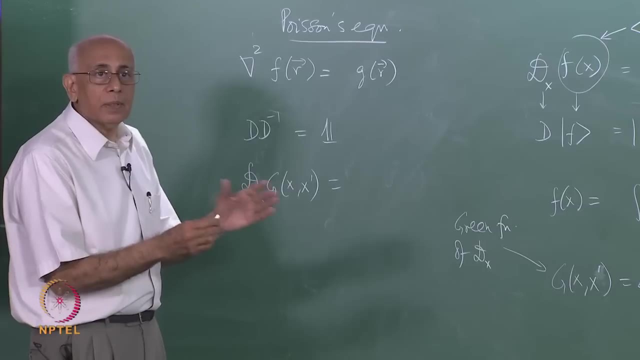 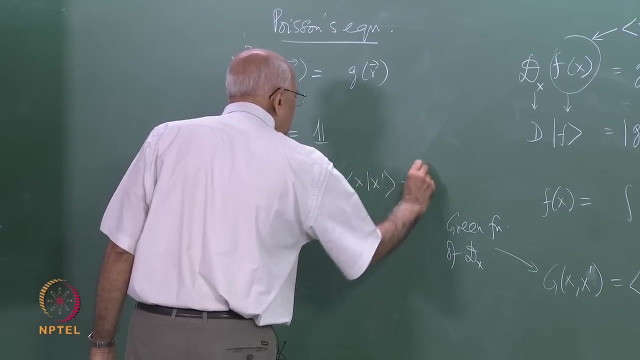 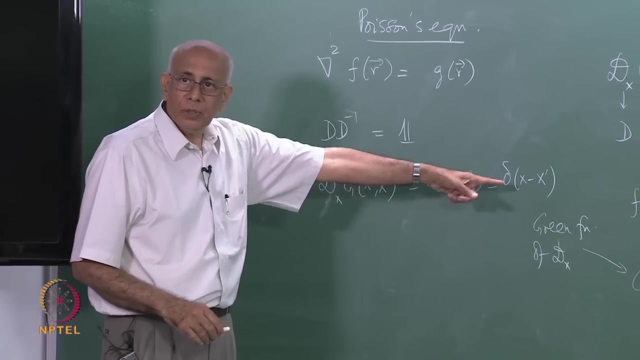 represented by d x, and this guy here is g of x comma, x prime, and that is equal to the bra of x with the cat of x prime, which is nothing but delta of x minus x prime. So solve this equation. 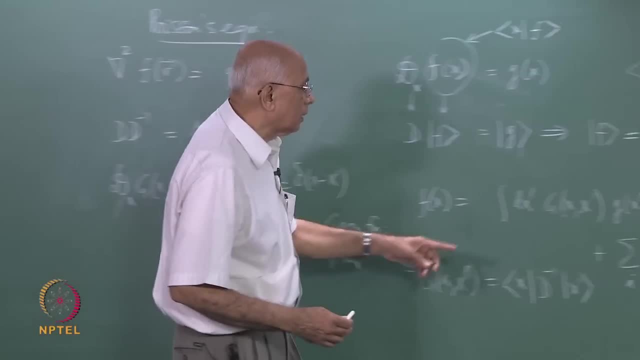 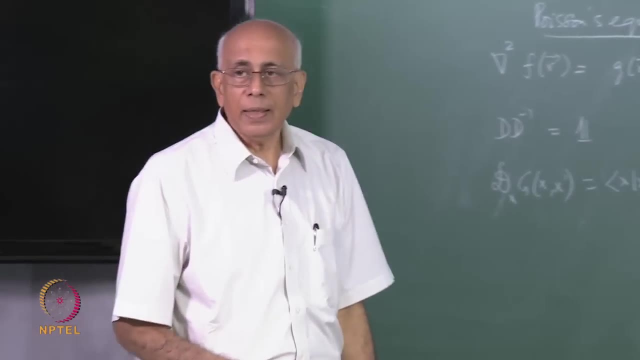 So if you have a function with a delta function on the right hand side and then you can solve this general equation by plugging that in here and then doing this integral, it gives you the particular integral. So this in a sense is the green function method. 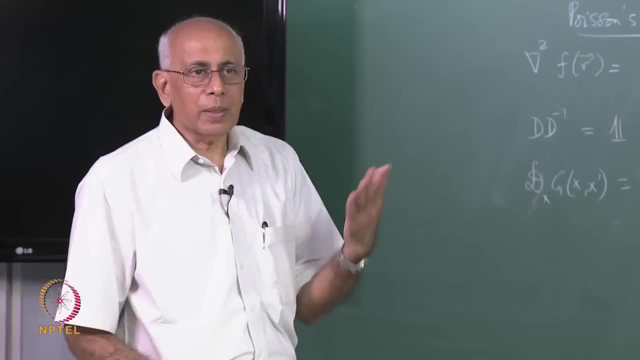 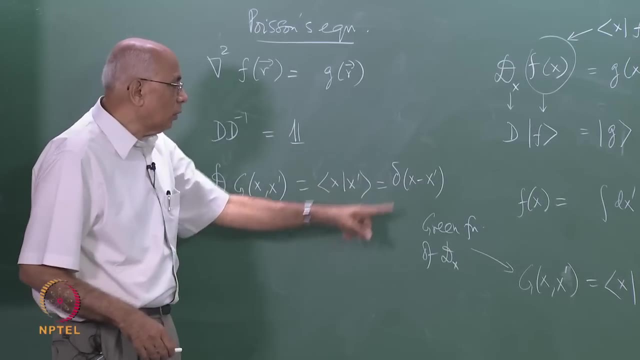 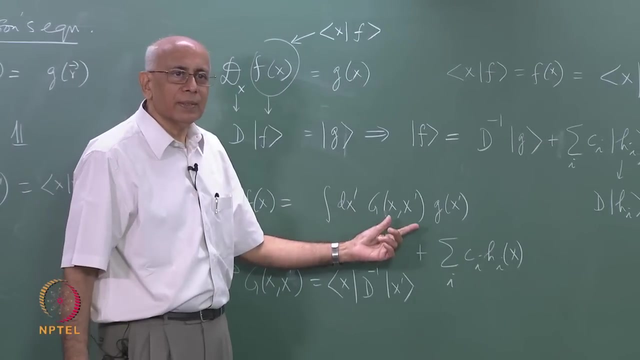 all you are doing is to invert some operator, writing it in some particular representation, and it satisfies this differential equation, And engineers are used to calling this the unit impulse function, or whatever it is, solve it and then you superpose. So this is all, such responses to the unit impulse function multiplied by whatever you. 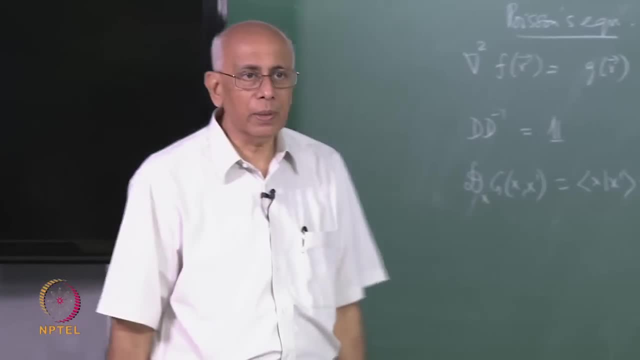 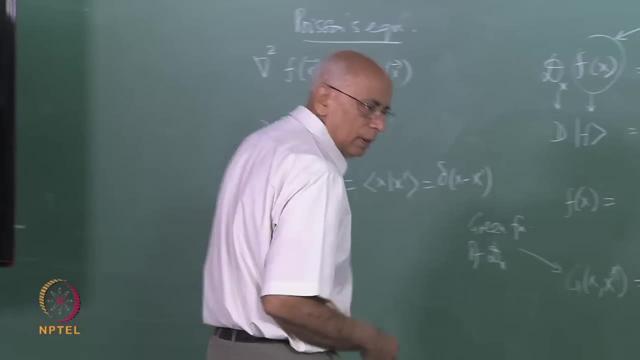 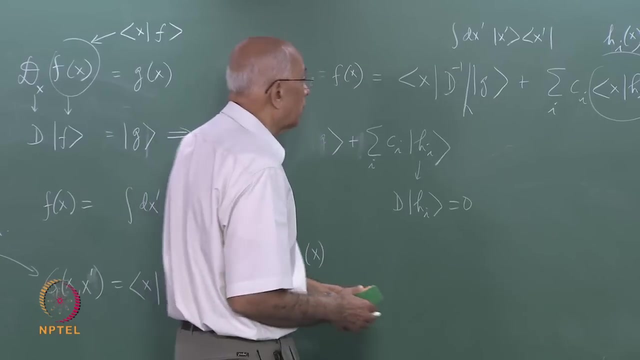 have there the given function and you have your solution. Now, how does this work in practice? well, if you look at the very simple example let us look at, just for to refresh a memory, let us look at an extremely simple example. First one question: I should ask how 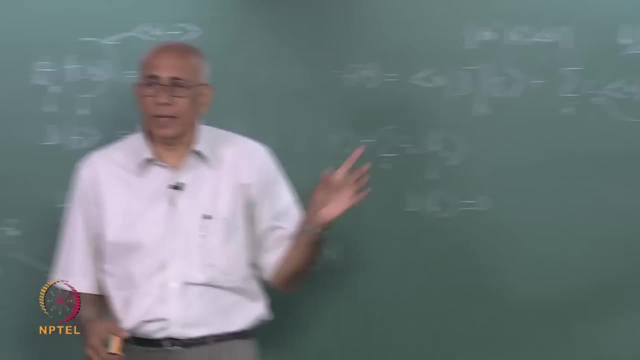 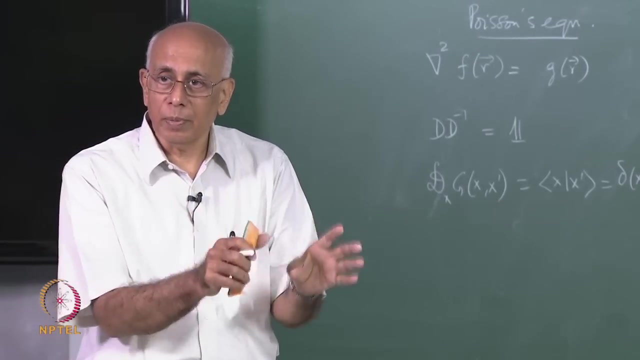 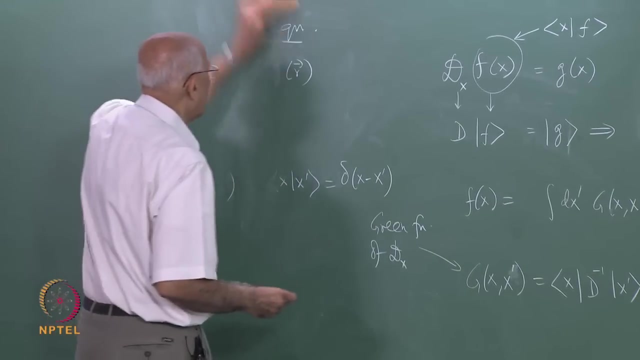 much of this. should you put this? put in: what decides that? So the conditions will decide what these coefficients are and what the admixture of the complementary function is to the particular integral, as we will see now from a simple example. So let us do this example first and then come back to Poisson's equation. 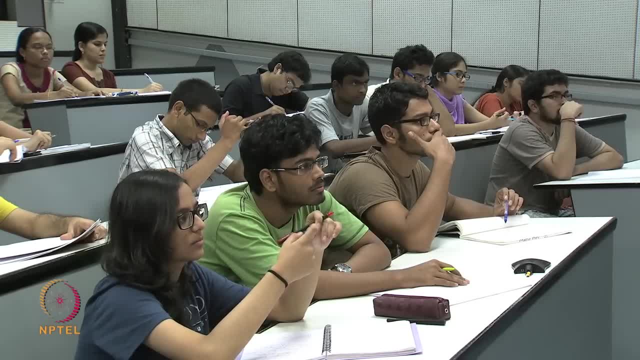 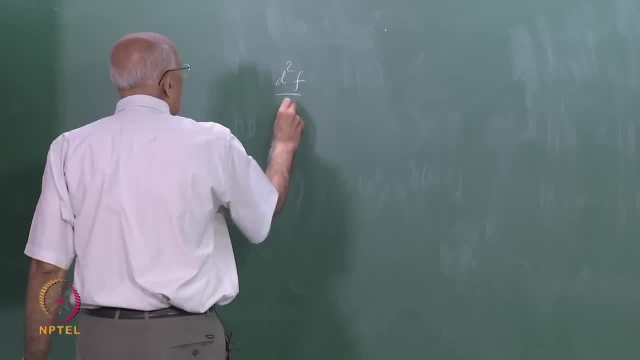 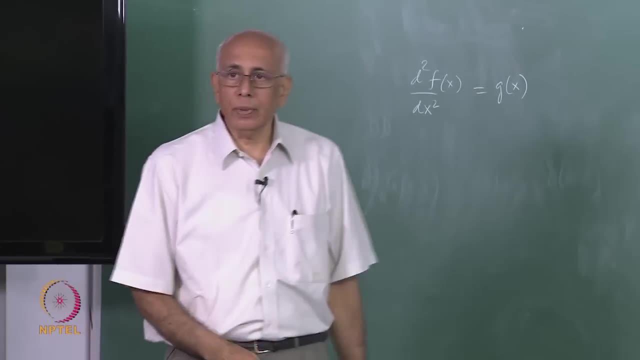 So the example is a standard one. it starts with a self adjoint differential operator, So it is of the form d 2 f over d x 2. this is f of x equal to some given function g of x. I would like to solve this. equation is the simplest of examples. we need some boundary. 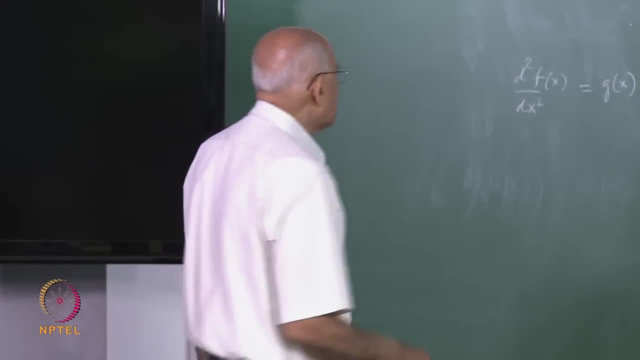 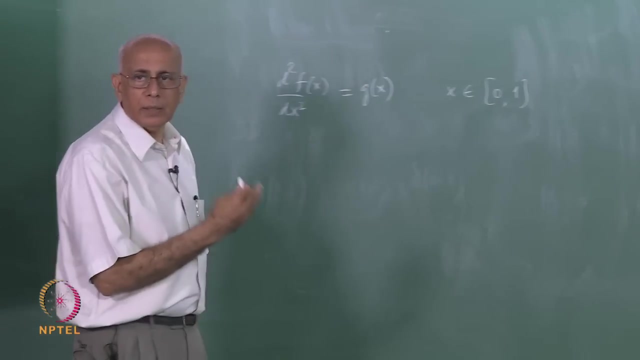 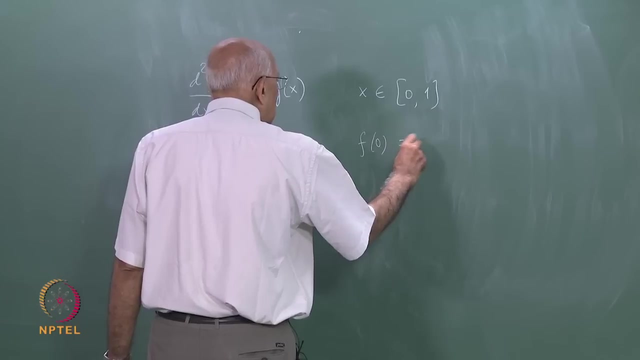 conditions and we need to say what is the range of x, etcetera. So let us take the unit interval. let us say x is an element of 0 comma 1 and I need to put some boundary conditions on this f. So typically you would say f of 0 equal to something or the other f of 1 equal. 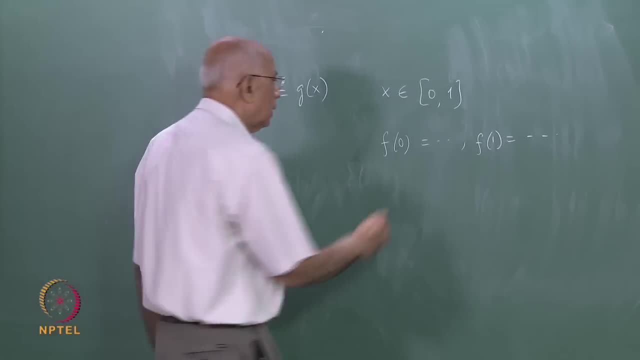 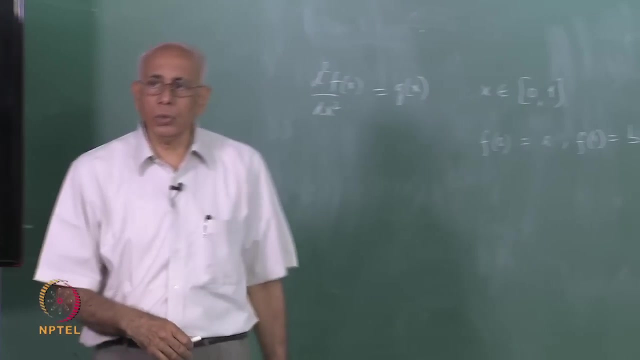 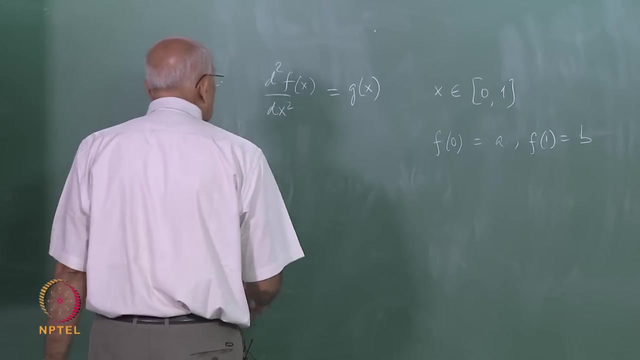 to something or the other, some constant, some other constant. call this f. So, subject to these boundary conditions, the question is: what is the solution to this differential equation? what is the particular integral here? So let us try to find out what the green function of this operator is. and the green function satisfies d 2 g over. 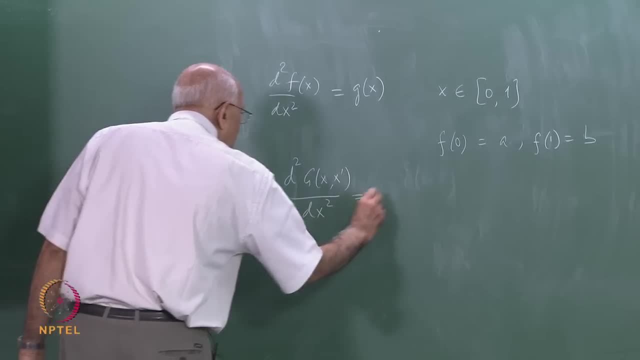 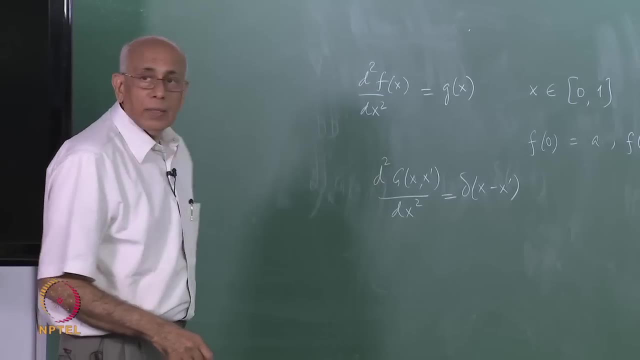 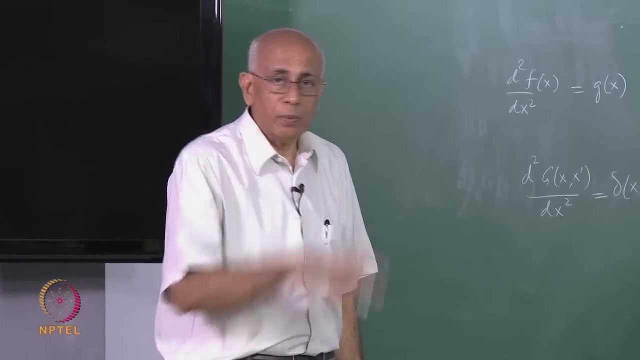 d, x, g, d x 2, equal to delta of x minus x point in this form. So what it says is that the second derivative of this with respect to x is essentially 0 except 1 x equal to x prime. So the big jump delta function of jump at x equal to 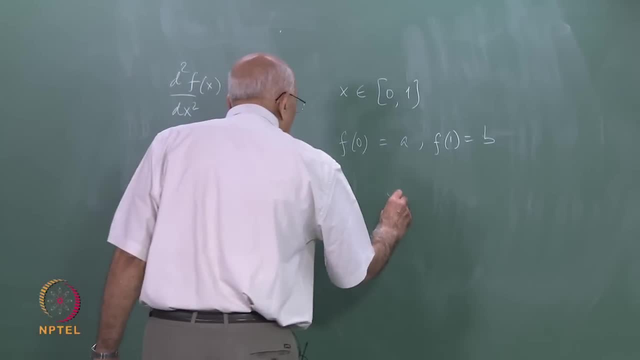 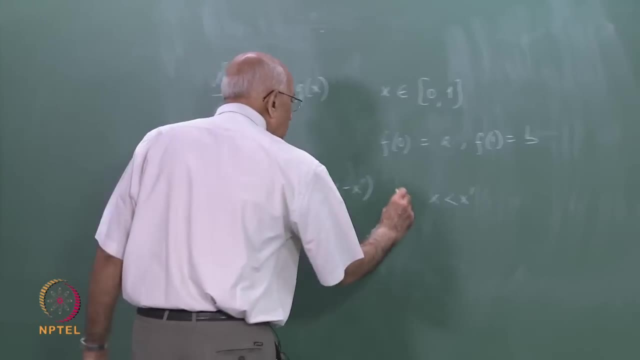 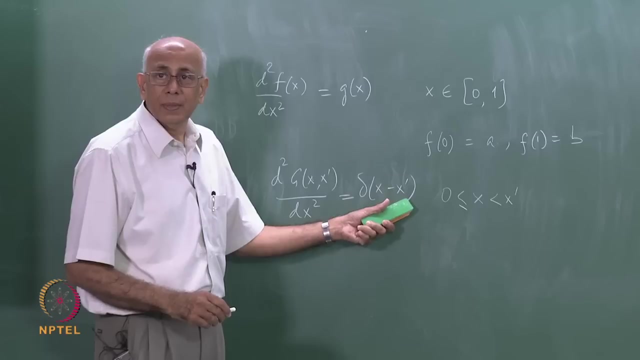 x prime. So let us for solve it in the region x less than x prime, then we solved it in the region x greater than x prime. So 0 less than equal to x less than x prime. what is the solution to this equation? well, this is 0 here, So it says the second. 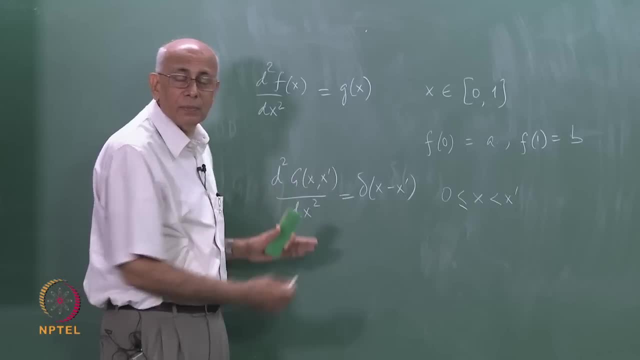 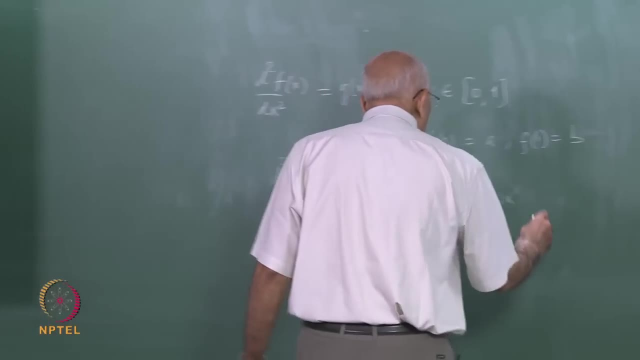 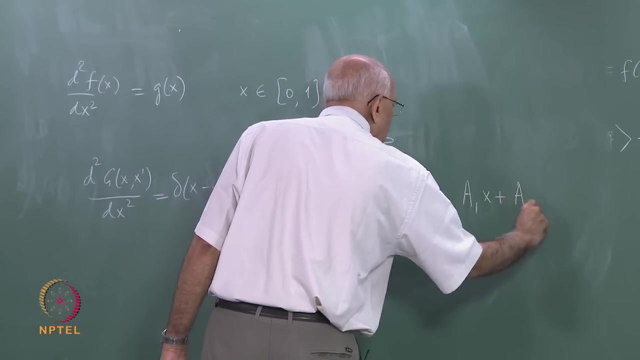 derivative of this g as a function of x with respect to x is 0, which means that g is just a linear function, right? So this is equal to. this implies that g of x comma, x prime, equal to some a 1, x plus a 2, a 1 and a 2 could. 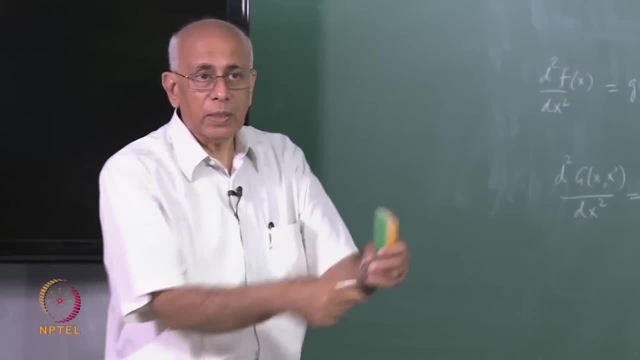 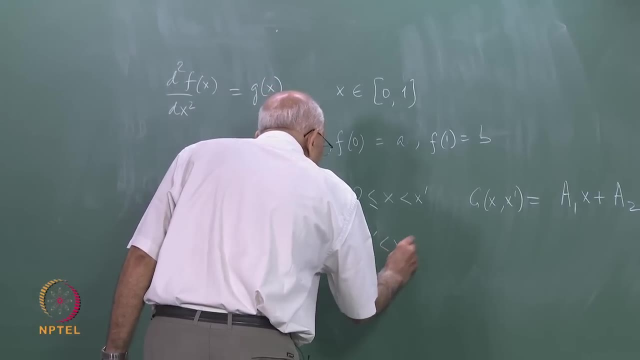 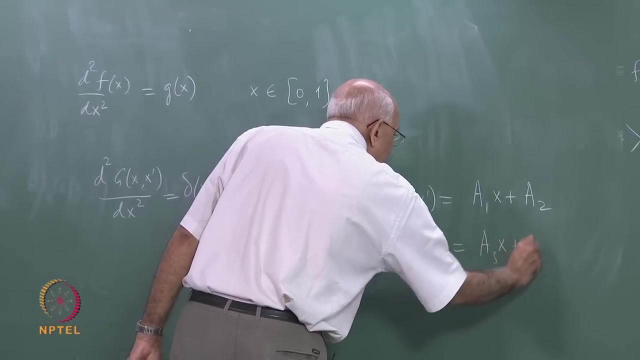 depend on x prime. in fact they would in general depend on x prime because we just integrated with respect to x alone And in the other region, x prime less than x, less than equal to 1 g of x comma, x prime equal to some of the constant a, 3, x plus a 4, and 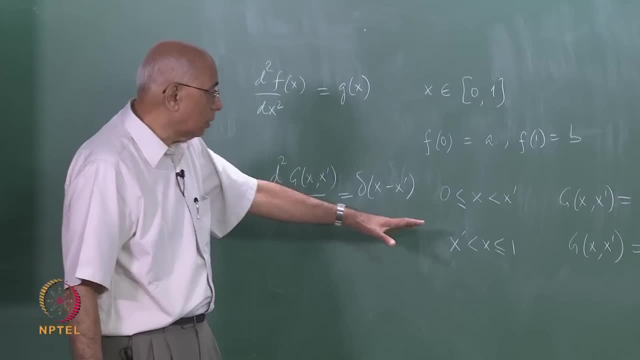 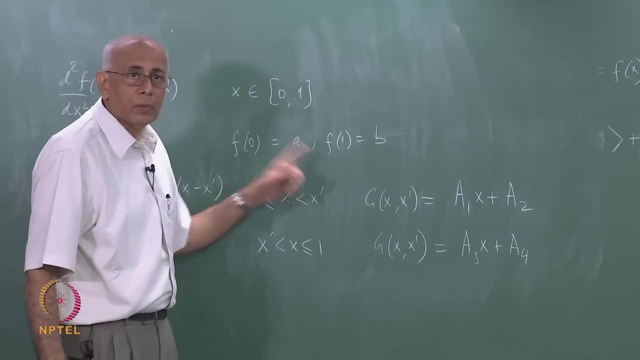 now we have 4 constants to be determined to give us the full g. and what are the pieces of information we have? Well, the first piece is this out here: So we put in the boundary conditions. I need to put in this boundary condition here. 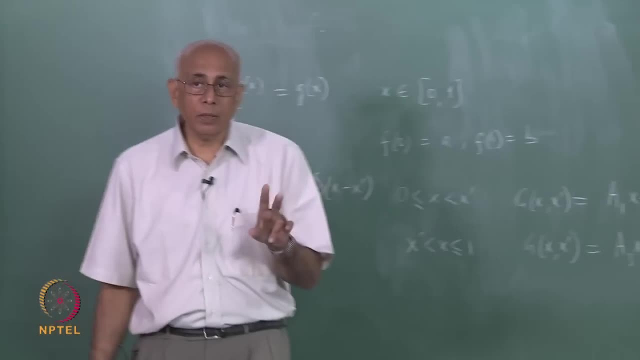 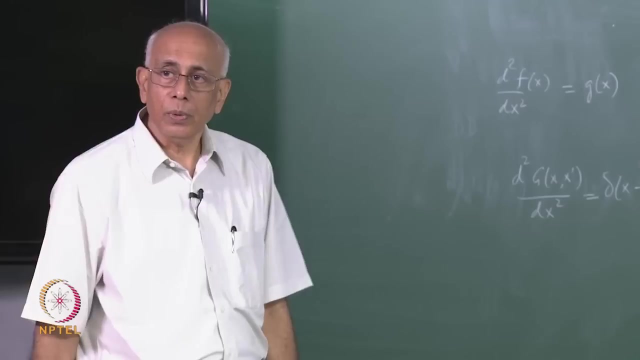 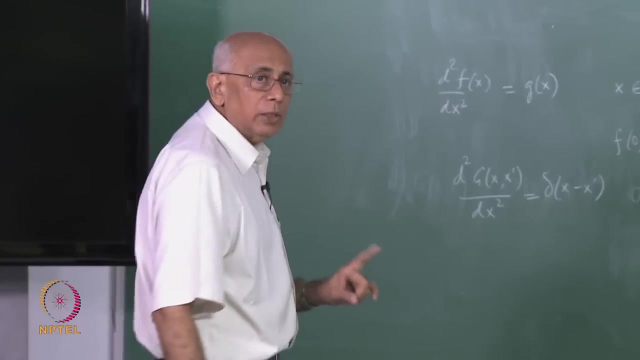 too. and then there are two other pieces of information needed to determine what the constants are. and what are those pieces of information? what would be well, the first one is the continuity of g. the reason I assert that g is continuous is because its second derivative has a delta function: jump. 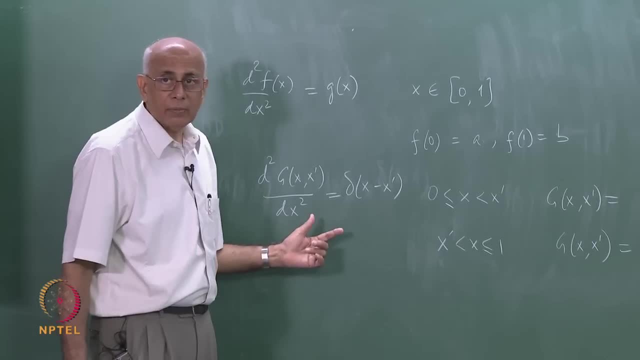 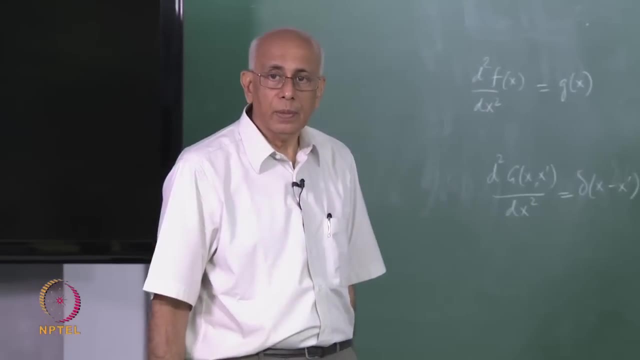 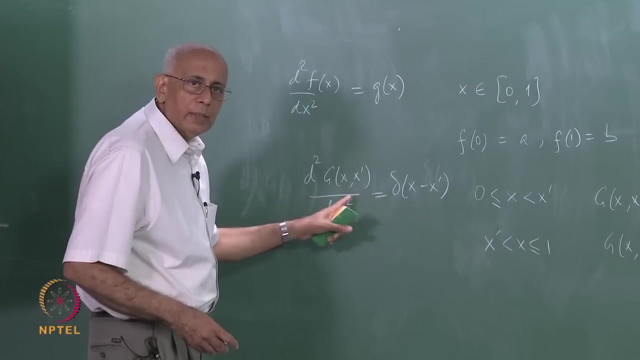 So what does it mean for the first derivative? this is got an infinite jump out here. So what does it mean for the first derivative? it means the first derivative has a finite jump of some kind. right, because if you integrate this equation, if you integrate this, 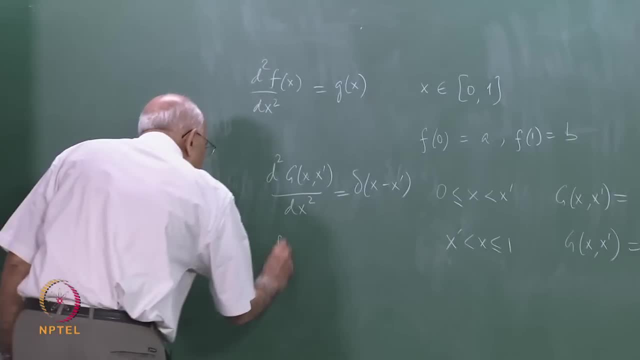 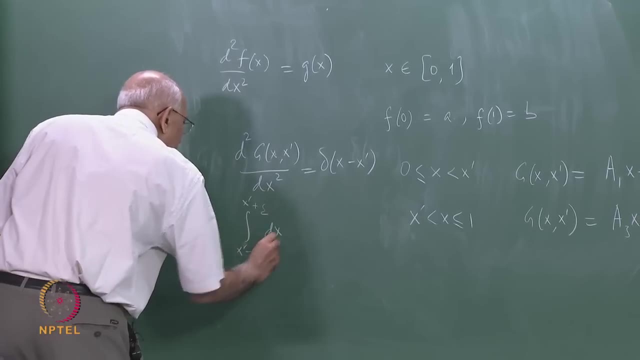 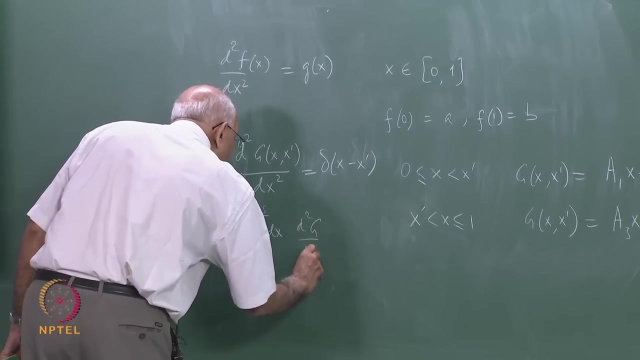 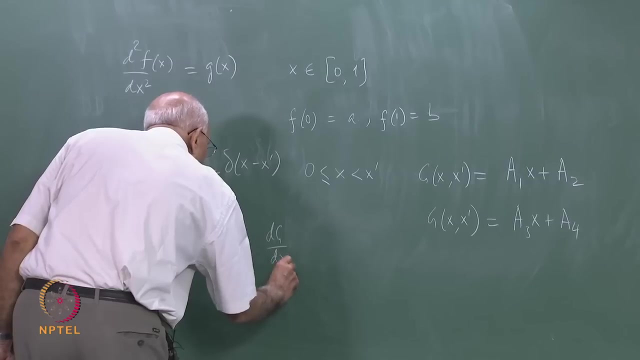 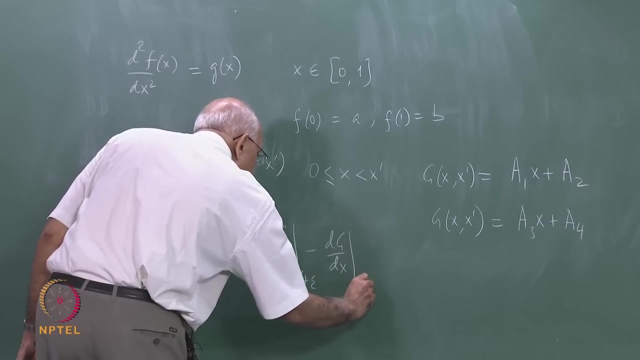 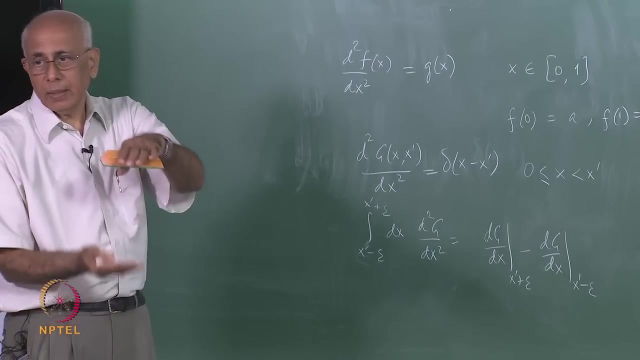 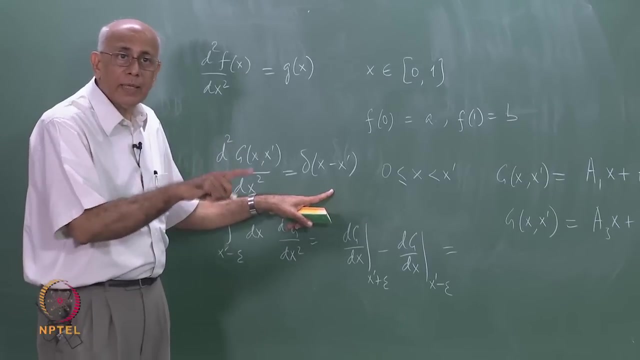 equation with respect to x. from some for a fixed x prime, say x prime minus epsilon, to x prime plus epsilon, you integrate d x and you integrate this. I integrate this across the point: x prime in x. So what is the answer? what happens? 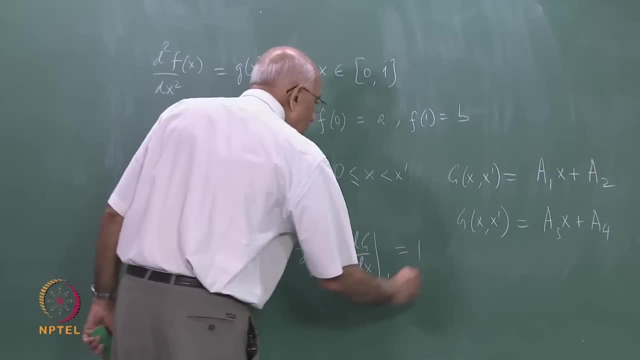 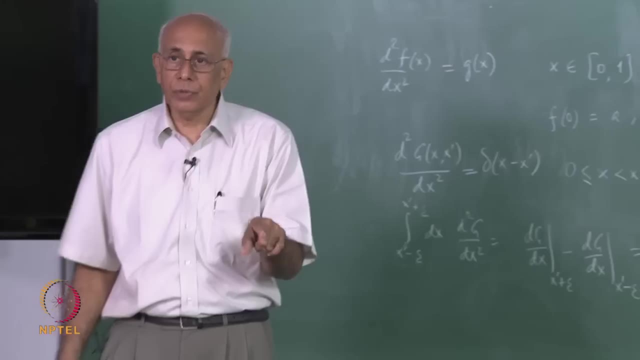 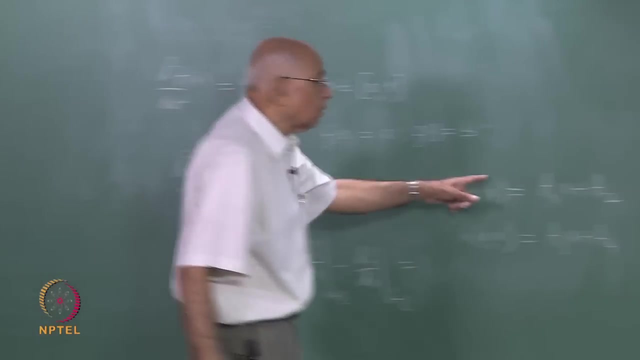 if you integrate delta function you get one. So this is equal to one. So in a sense it says that the discontinuity of the first derivative of g at the point x prime is given to you. So you need to use that information here. I differentiate both. 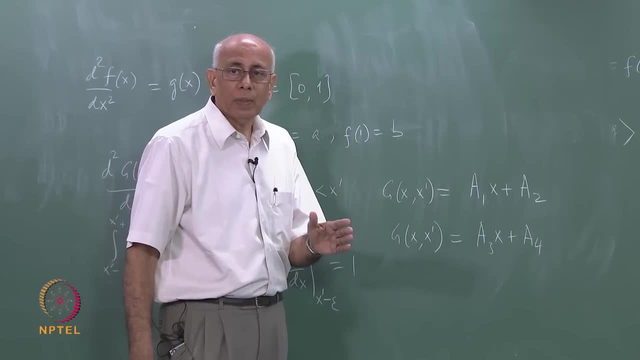 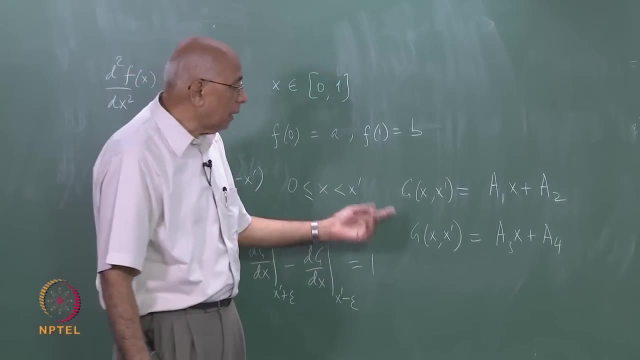 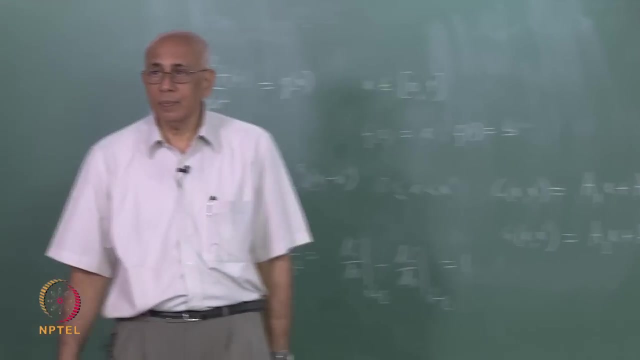 sides with respect to x and put x prime, x equal to x prime minus epsilon on the one hand plus epsilon on the other, and take the difference between the two. for the minus I take this and for the plus I take that and I equate the two at x prime, So that gives. 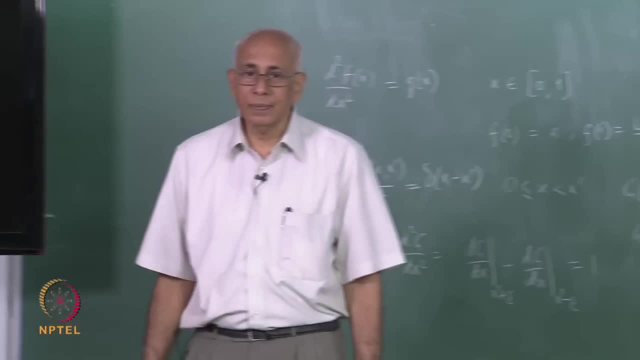 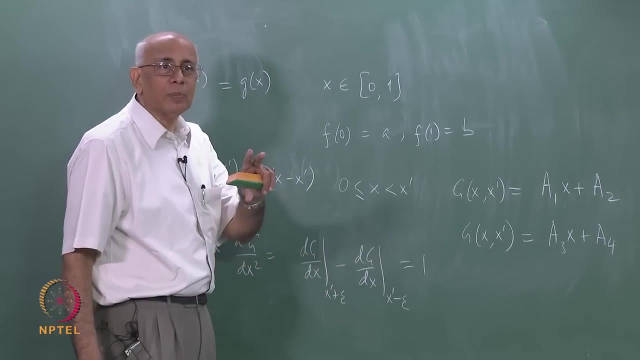 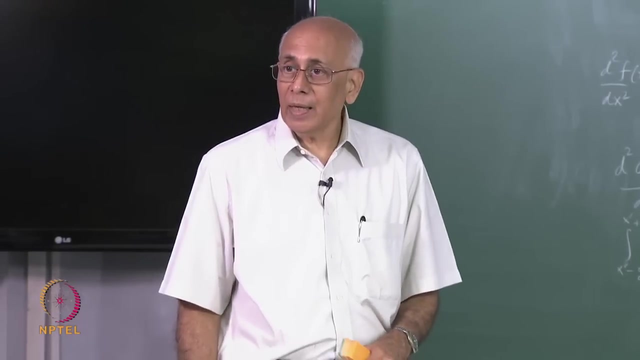 you one more condition, and what is the last condition of all this says that the derivative of g has a finite jump. So what is g itself have to have? It has to be a cusp. because it has to be something like this, because the 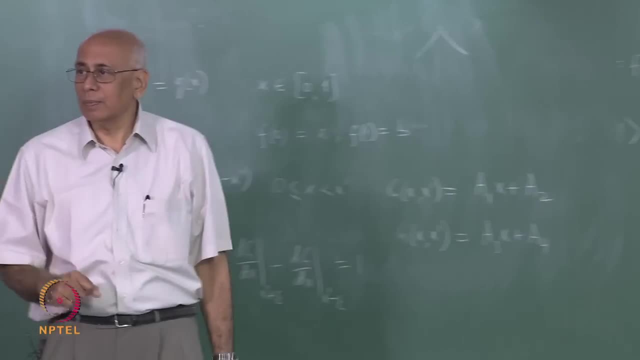 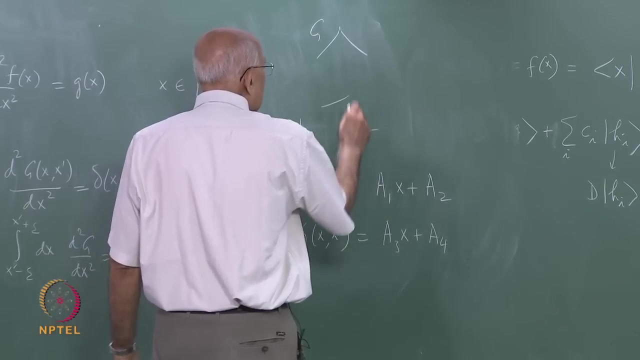 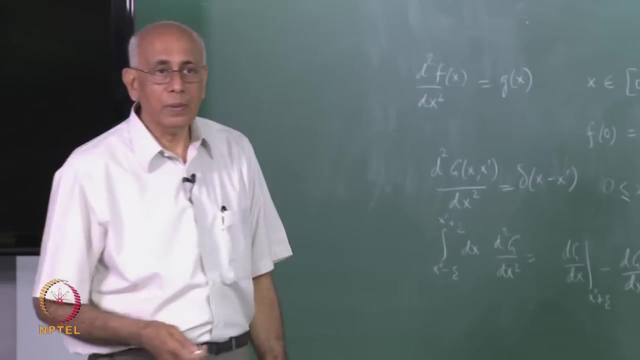 slopes are different and there is a finite difference between the two slopes. So the function g itself will look like this, g prime will look like this and g double prime will have a delta function. jump at that point. So whenever you have a delta function here. 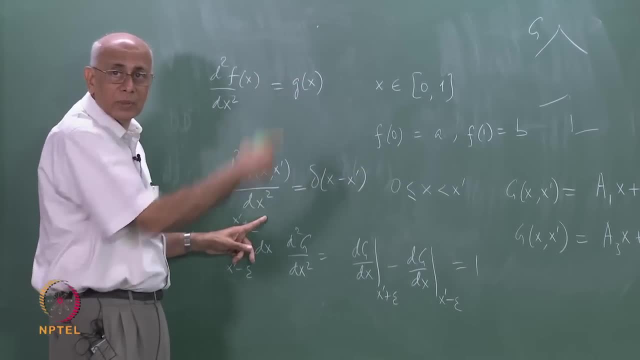 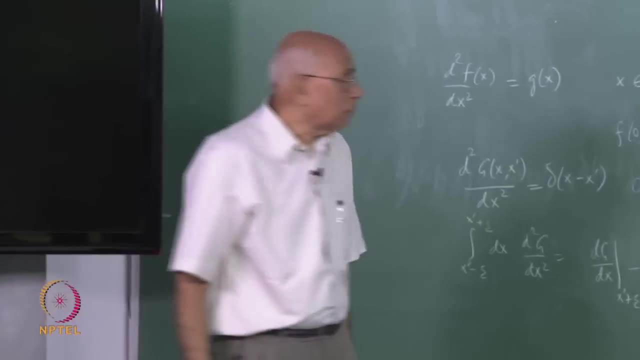 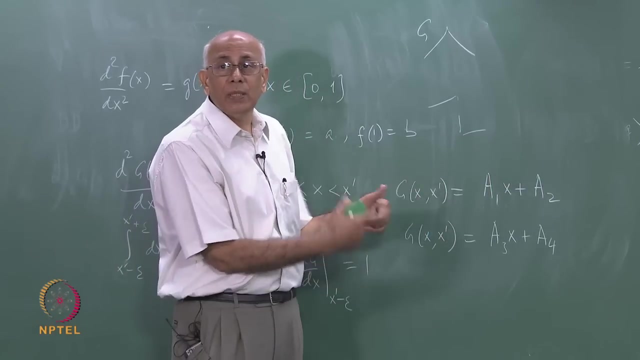 in the second derivative, you know immediately that the function itself would be continuous. but the first derivative has a known jump. So that fixes all the conditions. the first one is fixed by f at 0, then f at the other end at 1, then the continuity of g at the point x prime will give you one more condition. 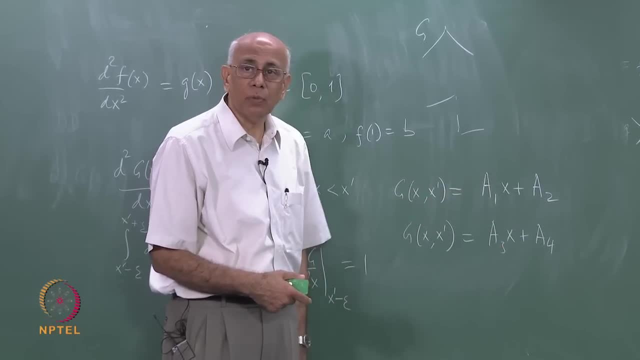 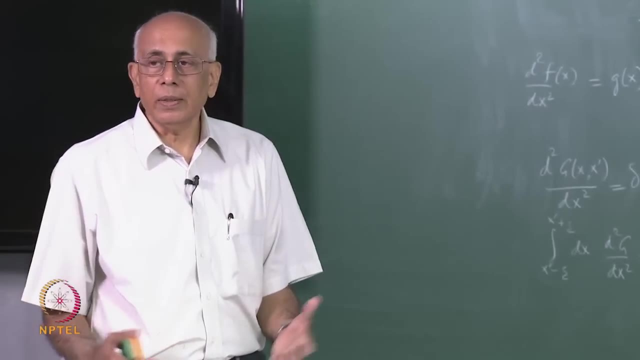 between the four constants, four quantities: a 1, a 2, a 3, a 4.. And the finite jump here gives you one more condition, So you can put those in and work out what a 1, a 2, a 3 and a 4 are, and that is your green function. You can do this for. 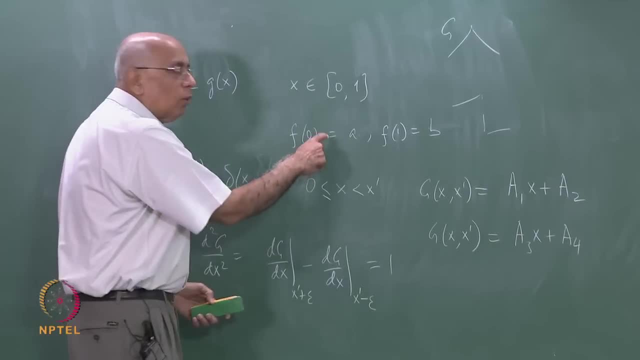 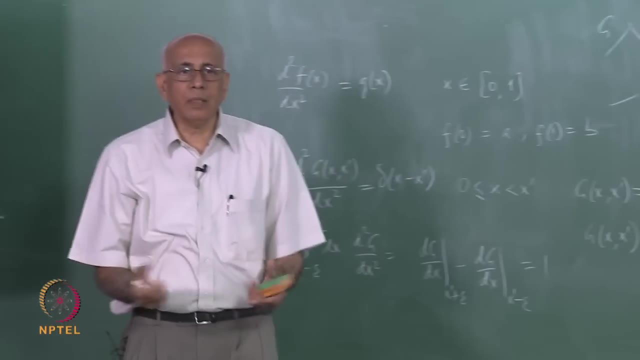 more general boundary conditions. the most general condition would be f of 0 plus some multiple of f- prime of 0 is something else- and similarly for 1.. These would be mixed boundary conditions, both sides, and you can write down the green function in the general. 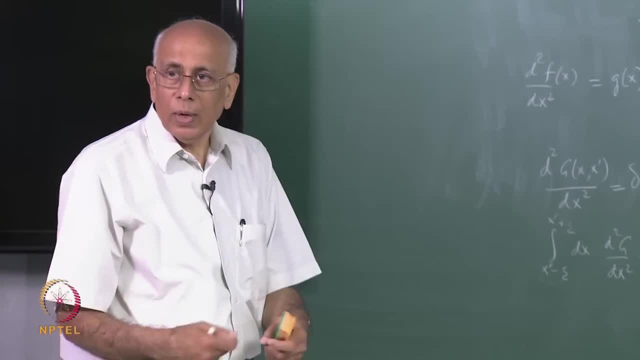 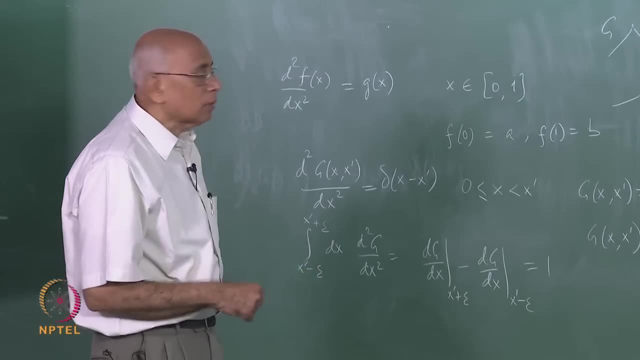 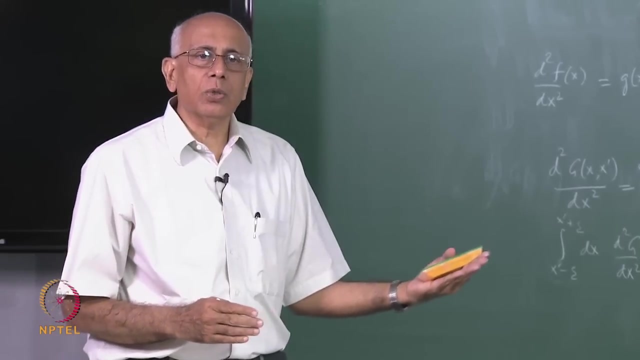 case. So this gives you some idea of how you handle the green function method. What we would like to do is a slightly simpler problem. in some sense we would like to do it for higher dimensions, certainly looking at partial differential operators, but we would like to use get the fundamental solution. So in 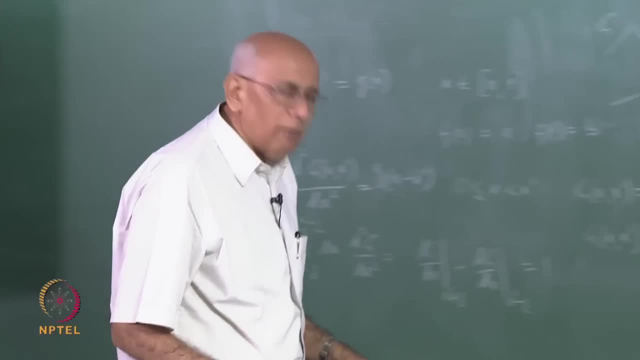 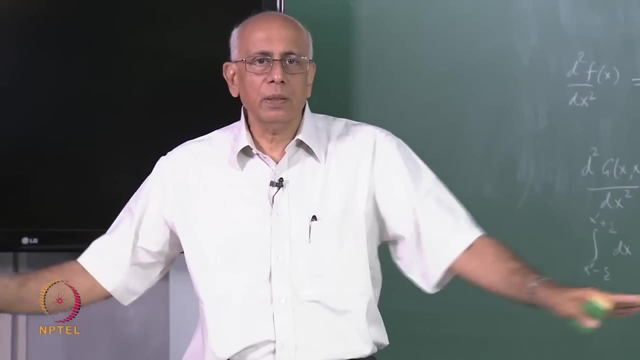 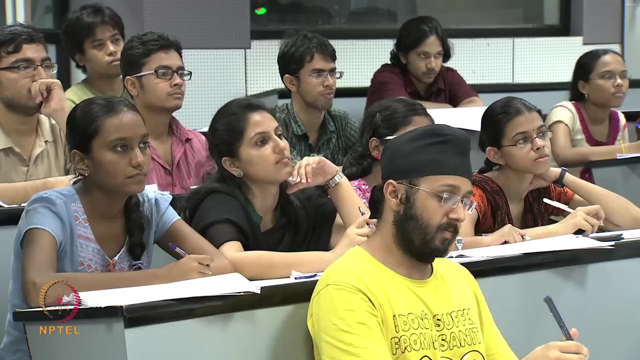 general, the boundary condition I am going to take is going to be the green function simply vanishing at infinity, or something like that. So we will take all of space and ask what happens. the green function vanishes at infinity. So now let us go back and look at Poisson's equation. will write the solution down by: 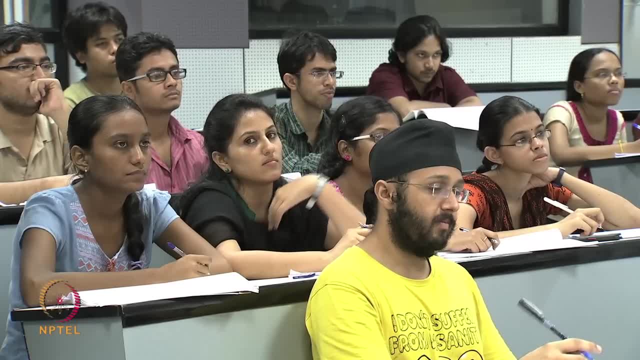 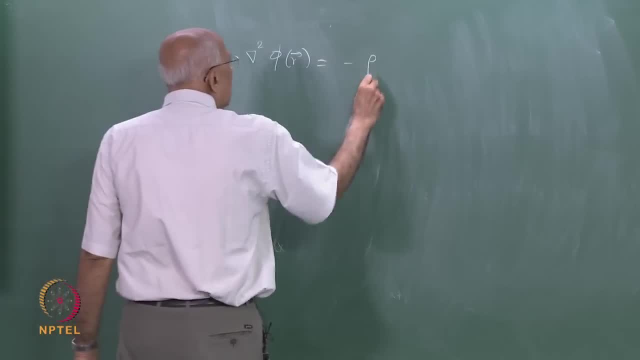 guesswork and then we try to derive it in more sensible considerations. So if recall this equation, pi of r is minus rho of r over epsilon naught. if you recall what solution to this equation is, Poisson's equation is electrostatic, is what is the solution to it is a essentially to решил this monster. 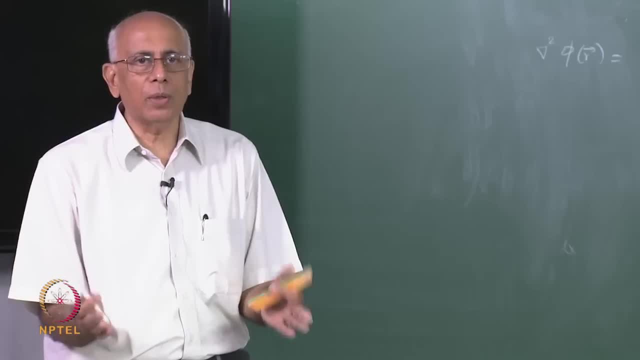 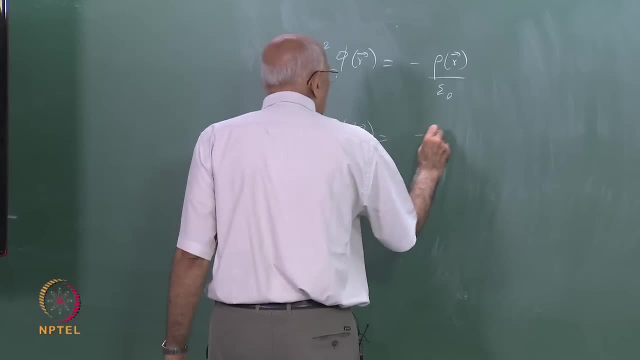 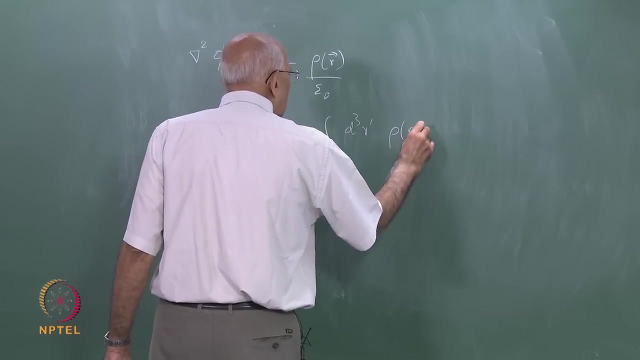 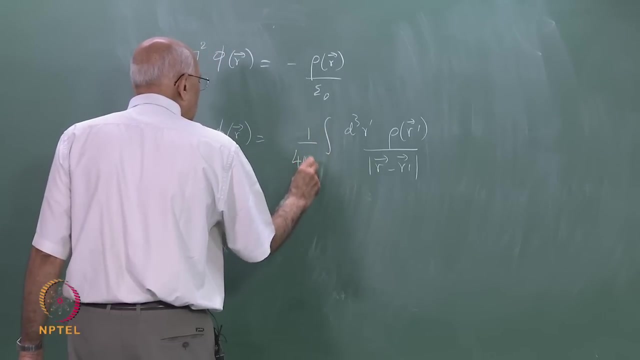 pulmes law. and if we look at the sociedad, what is? it is essentially column's law. right, right. The solution is: phi of r equal to minus, an integral, sorry integral. d 3 r prime. rho of r prime over modulus r minus r prime. 1 over 4 pi epsilon right. That is the 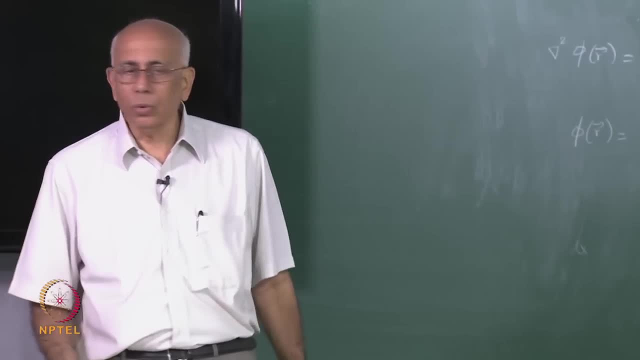 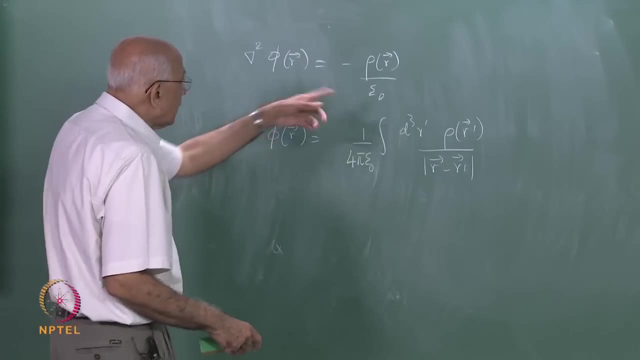 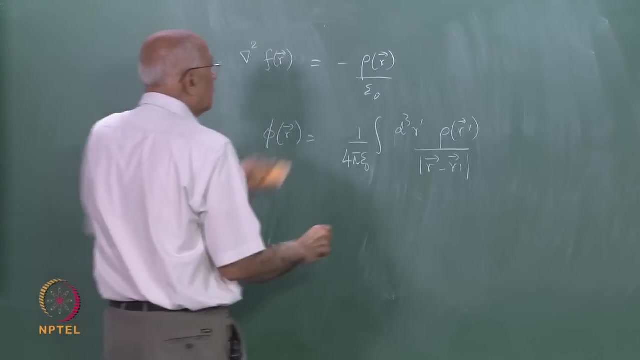 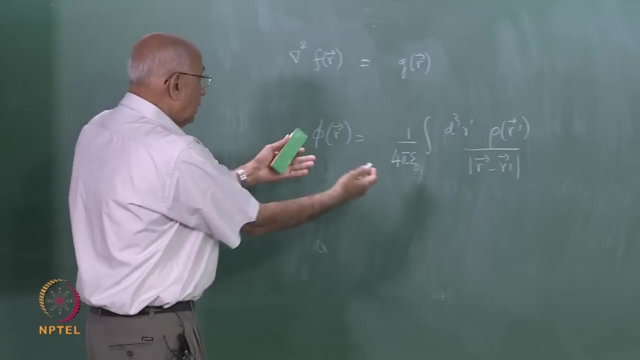 Kolom's law, and then the superposition principle is used to add up the potentials due to all the charges, all points where the charges. Now, what does that imply for the general equation? Well, the general equation was of the form f of r. this was equal to some g of r on this side. By analogy with this, it is clear. 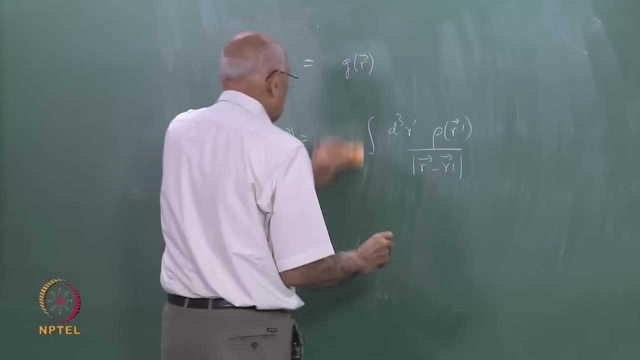 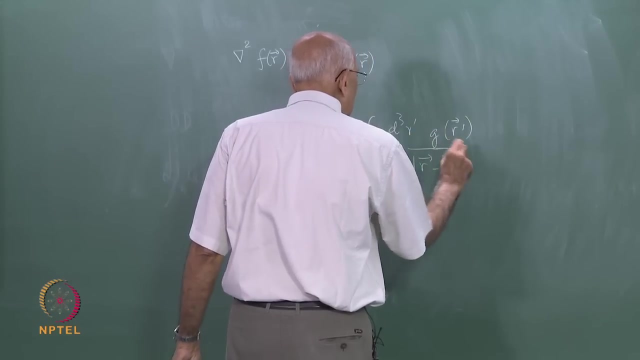 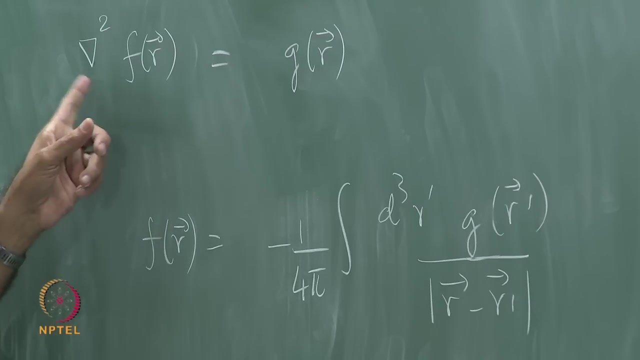 that the solution we are looking at is f of r is equal to minus 1 over 4 pi, g of r prime over this. So the green function in this problem for the del square operator is nothing but minus 1 over 4 pi mod r minus r prime. That. 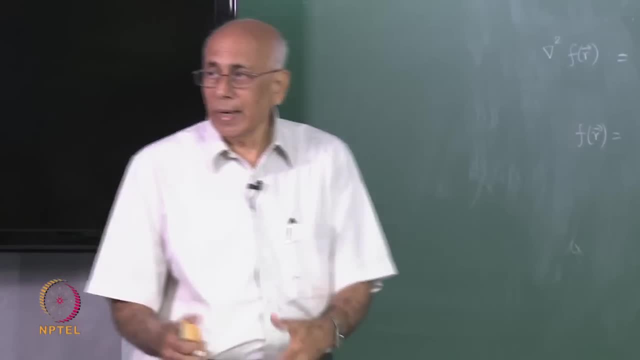 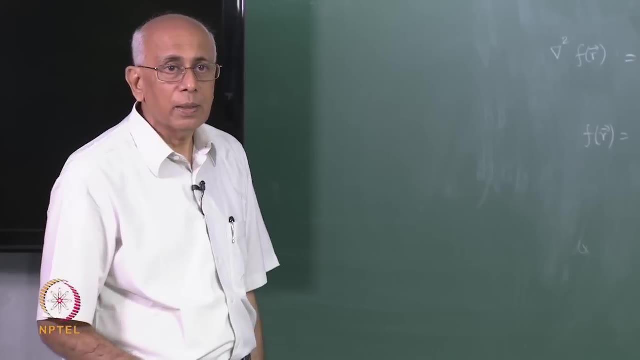 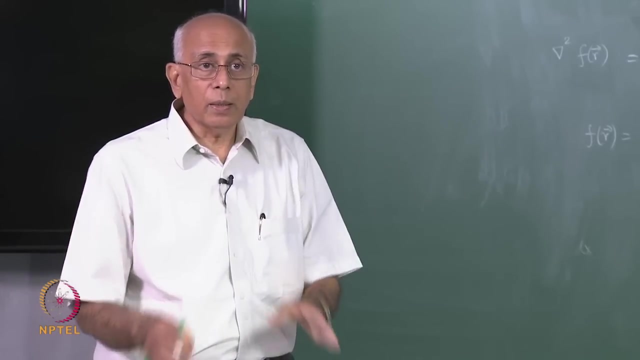 is the green function and we should get this, We should be able to derive this rigorously, that this is indeed the green function for the three dimensional del square operator, satisfying the boundary condition that this solution, by the way, for Poisson's equation, is written down, assuming that the potential vanishes at infinity. So the boundary 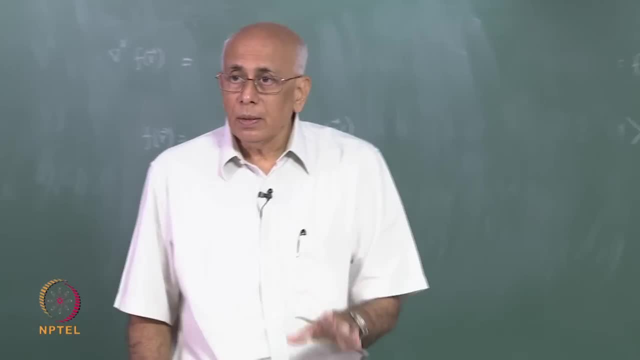 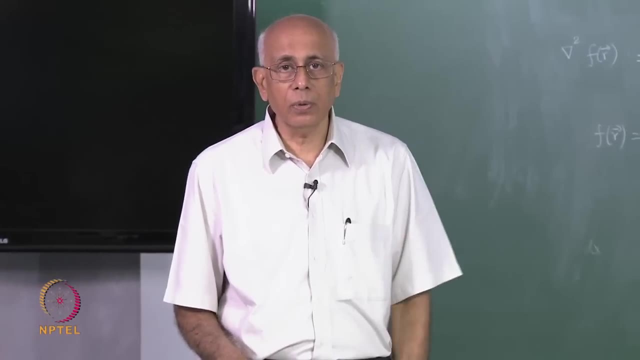 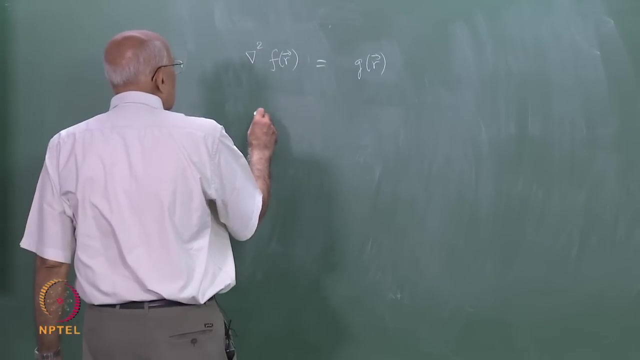 condition on this g is that as r goes to infinity, this g vanishes this whole thing. So this is the free green function with natural boundary conditions. and now let us see how to derive this. So we will start with this equation and write the particular integral. 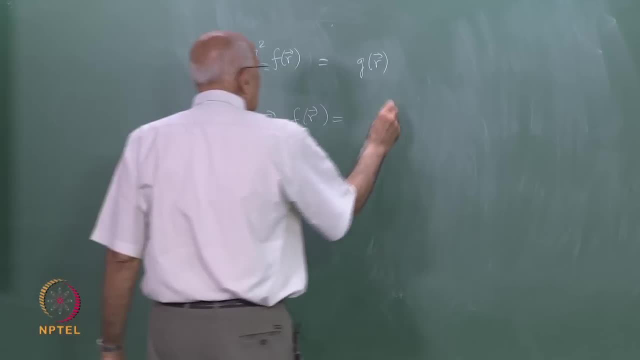 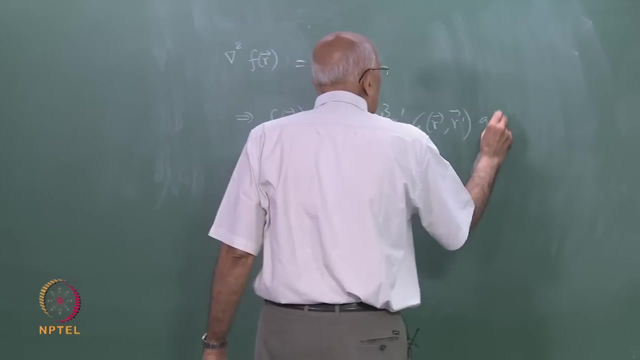 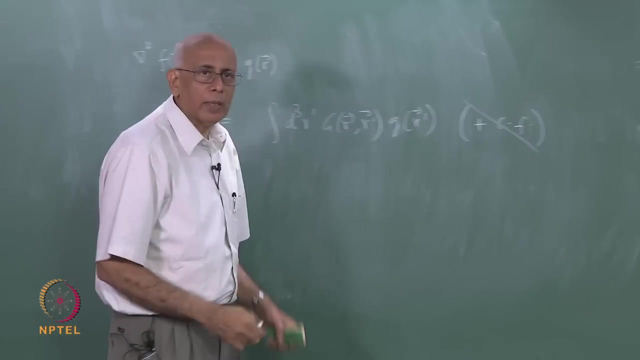 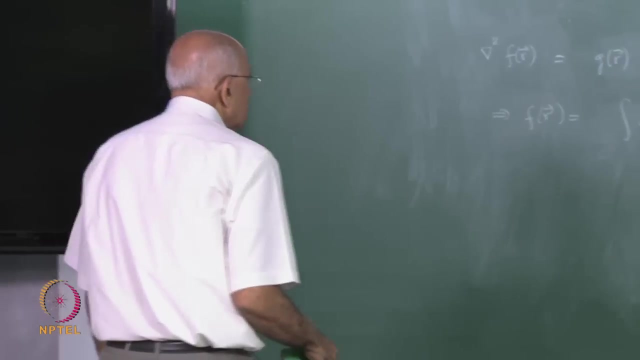 So we have the following equation: that f of r is equal to an integral d 3 r prime g of r, comma r prime little g of r prime, plus of course the complementary function. but I am not interested in it at the moment. I just want to know what the green function is. 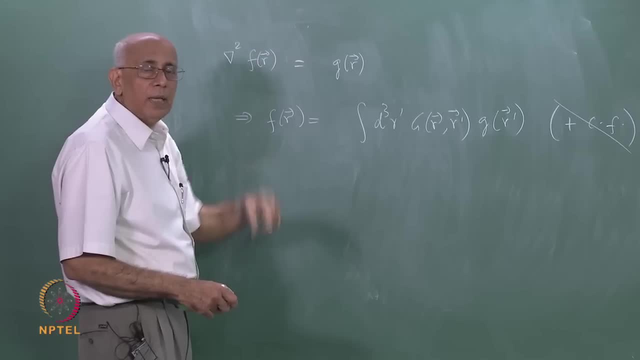 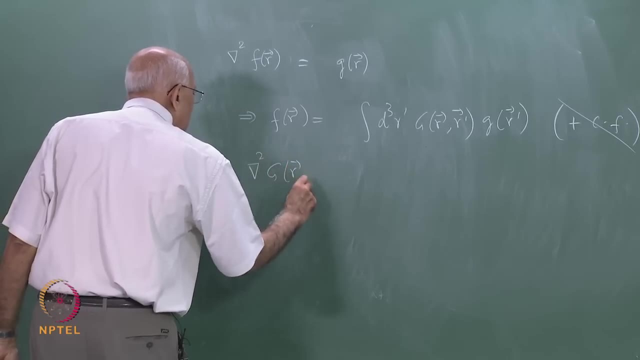 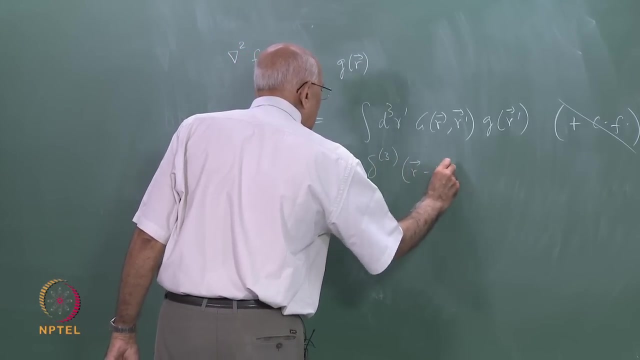 And what equation does this g satisfy? It satisfies the same equation as here, with a delta function on the right hand side. So you have del. square g of r- r prime is equal to a delta function, a three dimensional delta function of r minus r prime, in this case. 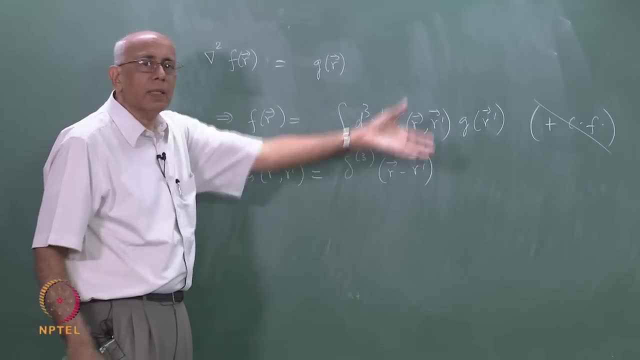 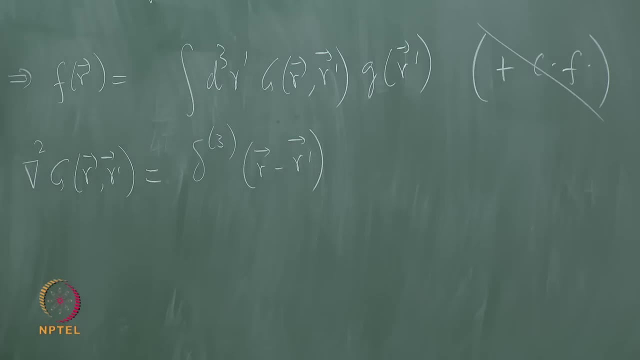 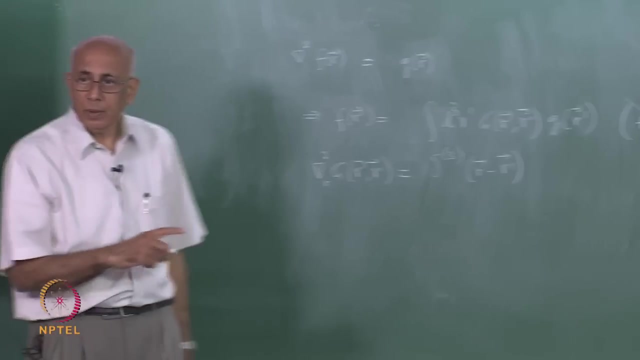 I need to solve this equation, put the solution back in here and then that is it. that is the particular integral. Now, just to remind myself that the derivative or del square is with respect to r. Let me just put an r here to show that it is with respect. 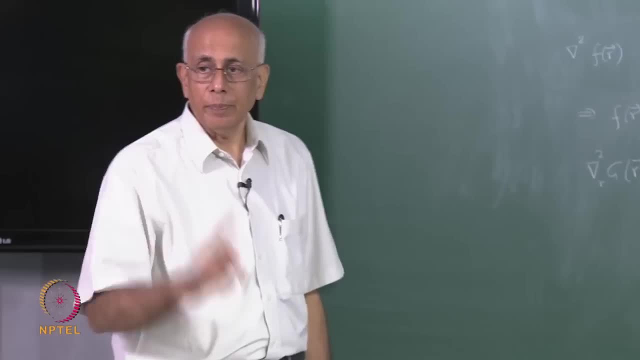 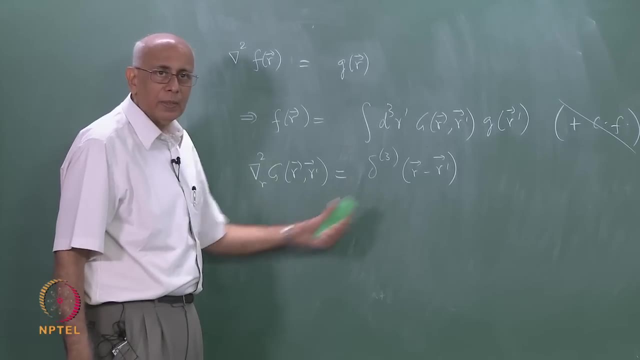 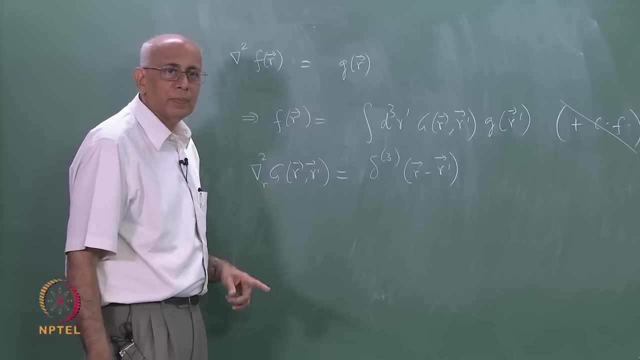 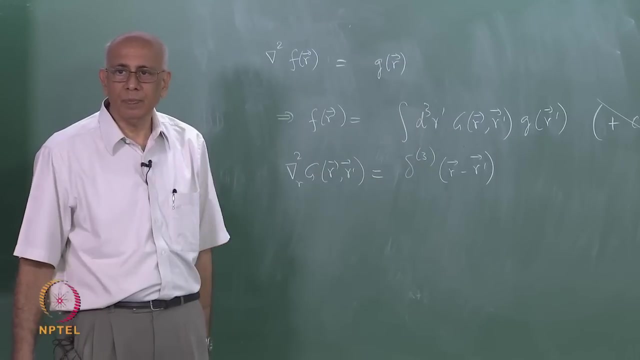 to the variable r, the vector r rather than r r prime. Now I assert that this equation here implies immediately that this g is a function of r minus r prime and not r alone. And there is not do. that is because the right hand side is a function of r minus r prime. 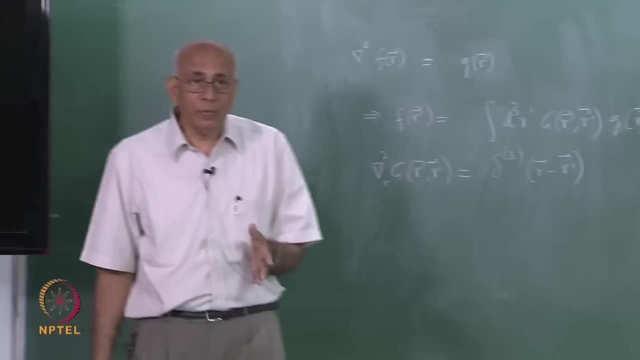 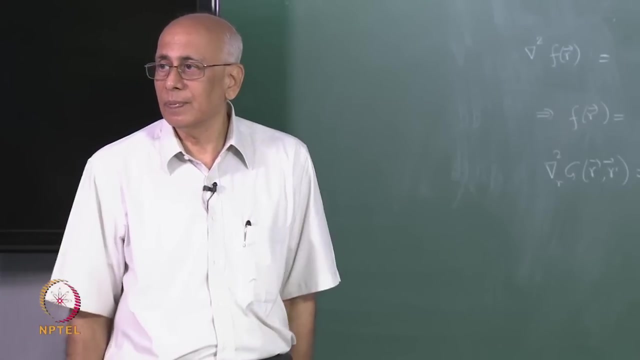 del square del itself. the derivative with respect to r is the same as the derivative with respect to r minus r prime for every fixed r prime is just a shift. Are these two statements enough to say that the solution will also be a function of only r minus r? 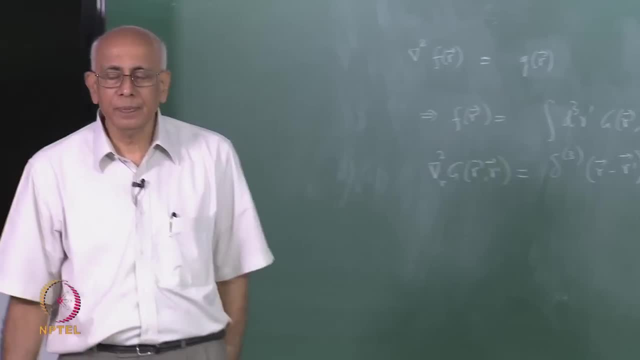 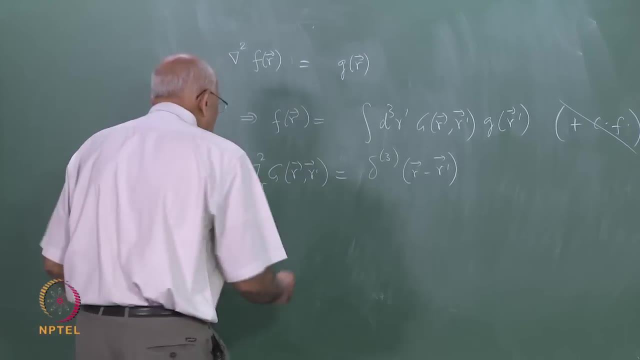 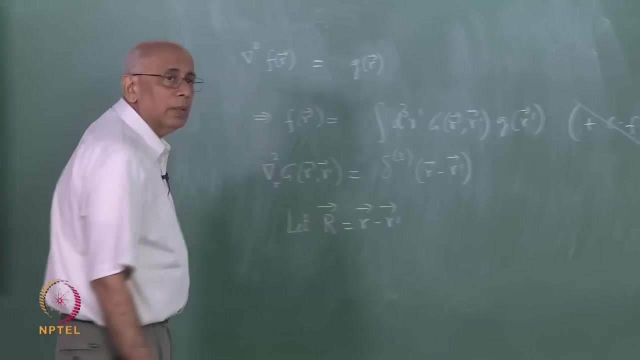 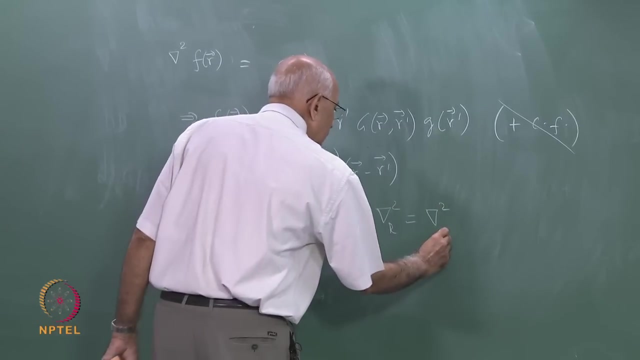 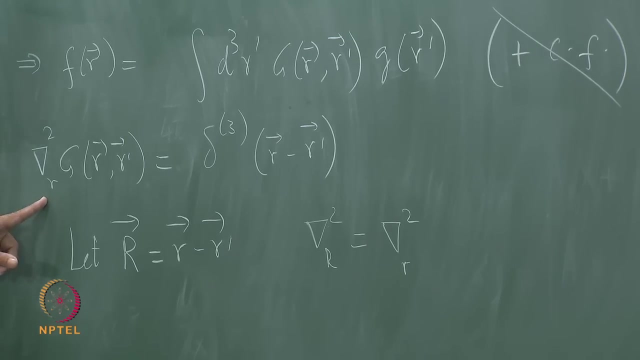 prime. are these enough? del square is invariant, So if I put r equal to r minus r prime- So let this be true- then my statement is: del r square is the same as del r square is just a shift. So this guy could be written del capital r. this is: 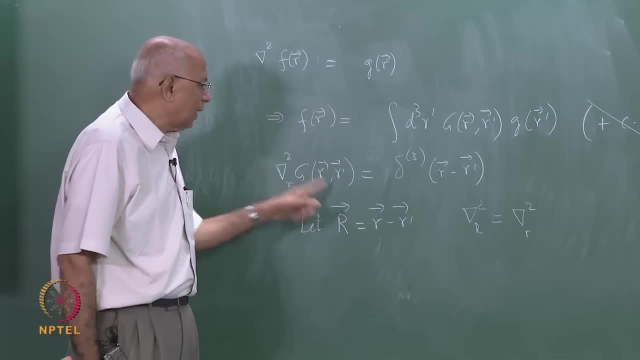 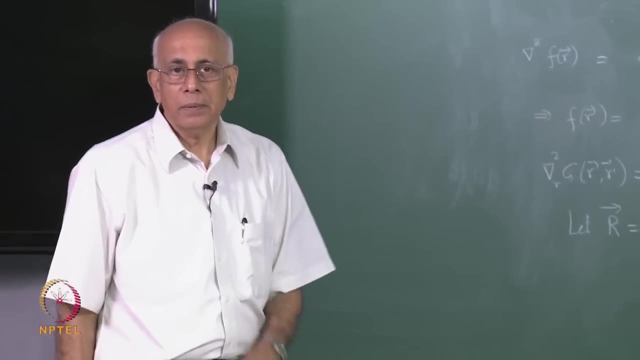 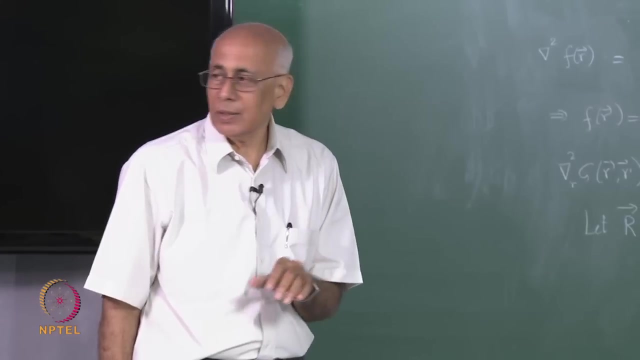 delta three of capital r vector. So can I now assert that this also is a function of capital r vector? can I do that In the think of the example we looked at a little earlier: d, two f over d x. two equal to the right hand side was again a delta of x. 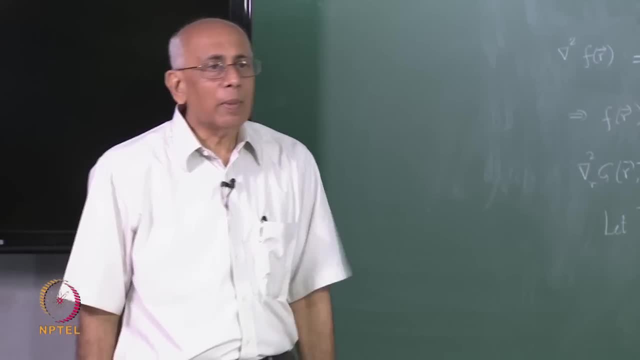 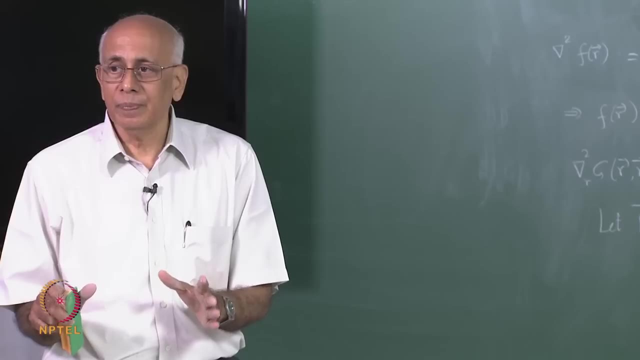 minus x prime for the derivative, second derivative operator. But that green function did not turn out to be within work it out fully. but it is not a function of x minus x prime. why not? the d two over d x two was also d two over d x minus x prime. 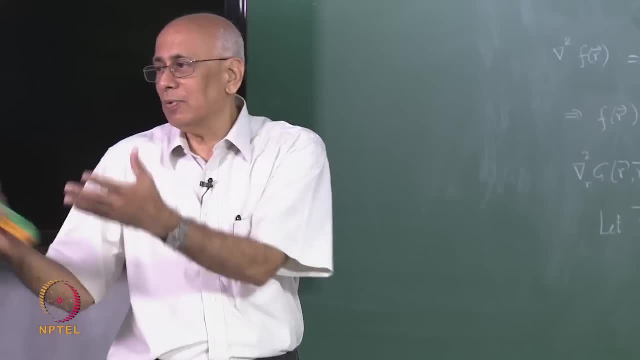 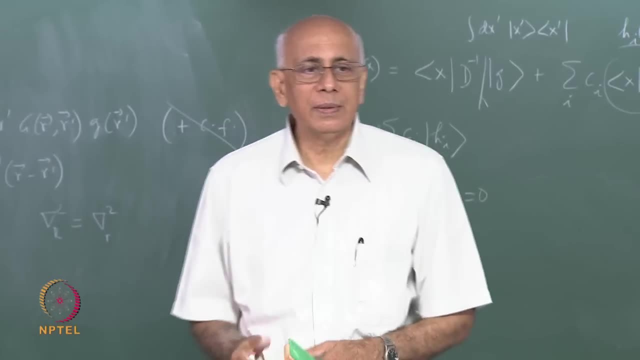 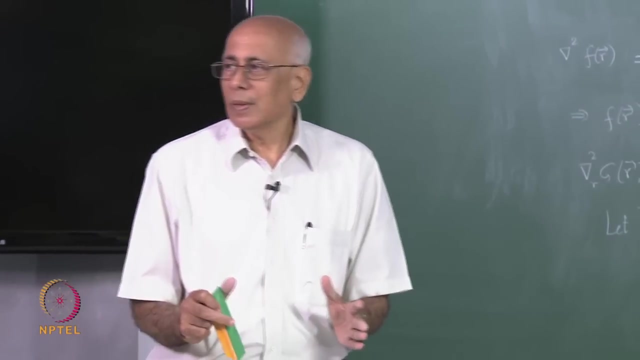 The second derivative, the delta of x minus x prime, function of x minus x prime. and yet the green function did not turn out to be a function of x minus x prime. what happened? Yeah, finite boundaries. the boundary condition broke this translation variance. the boundary condition broke it. So you cannot shift arbitrarily because the finite boundaries in this 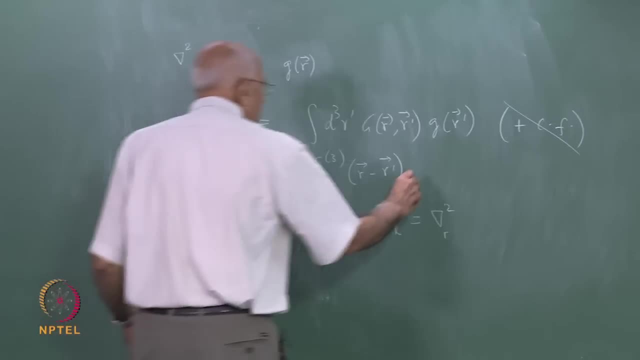 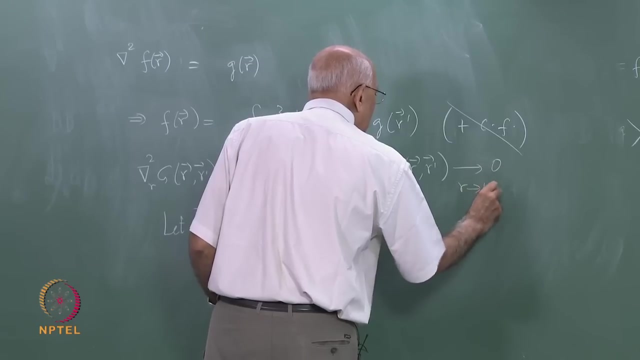 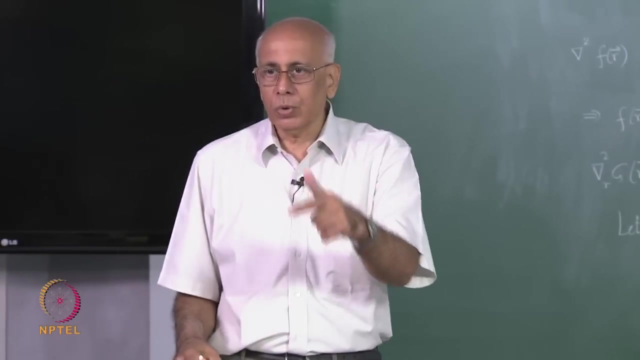 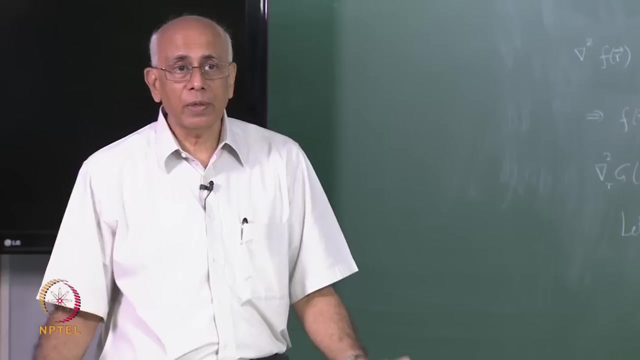 problem. However, we are asking for a solution. As this vector goes to infinity, we are asking for something which goes to 0 right. So as r goes to infinity, r minus r prime also goes to infinity for every fixed r prime. So in: 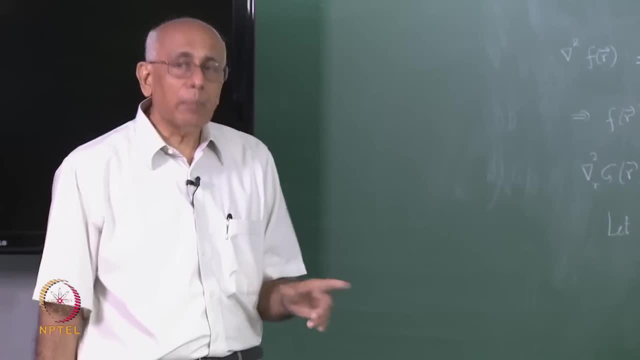 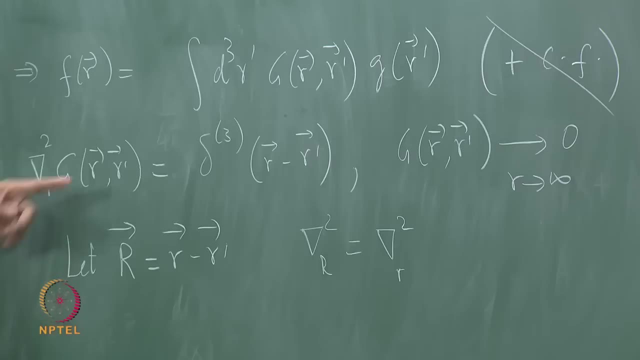 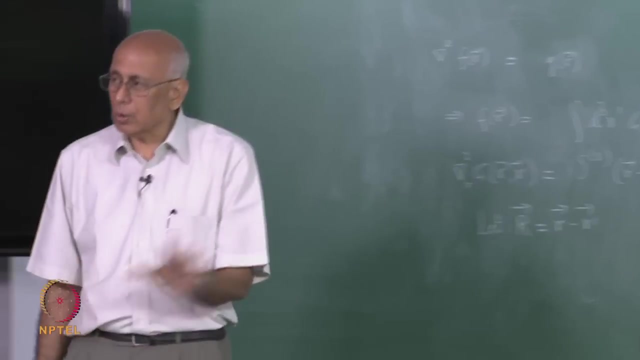 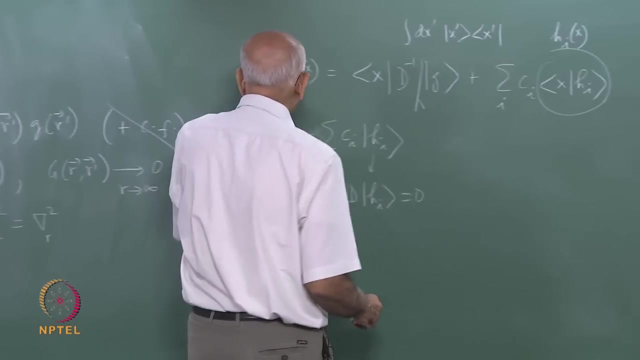 this problem with these natural boundary conditions. the boundary condition is also translation invariant. This translation invariant, the inhomogeneous term- is translation invariant, and so is the boundary condition. So we can assert, therefore, that the solution is also translation invariant. So this will imply now that the equation we have to solve, So we have to- 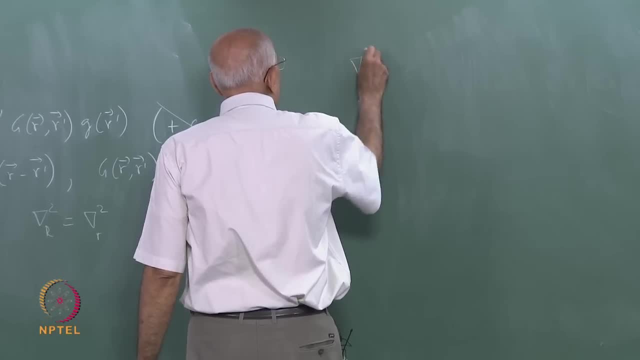 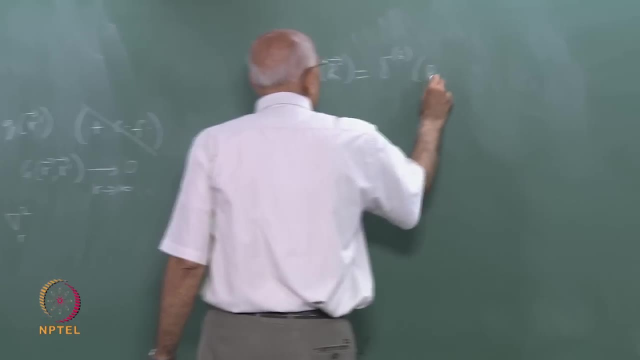 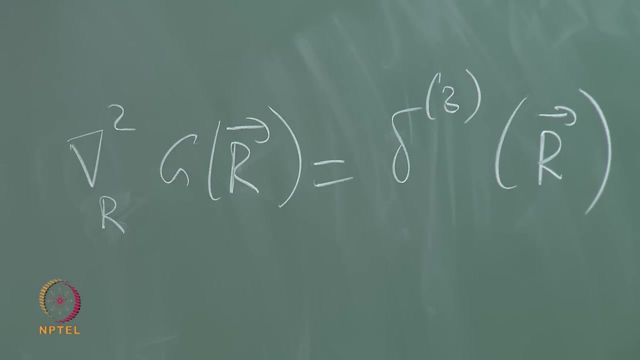 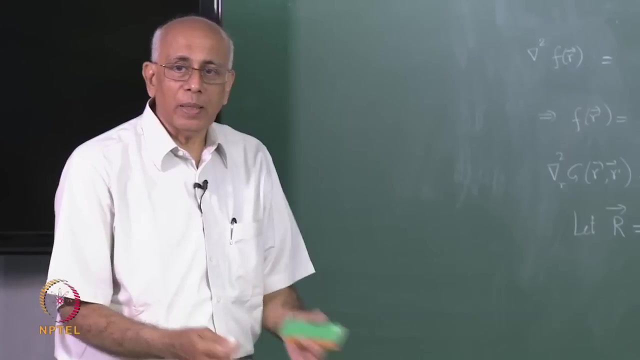 be careful, therefore. So the equation we have to solve is del r square g of r, equal to delta three. That is the equation we have to solve. What should we do? We should do something which converts this del square into a multiplication, and the obvious thing to do is to do the Fourier. 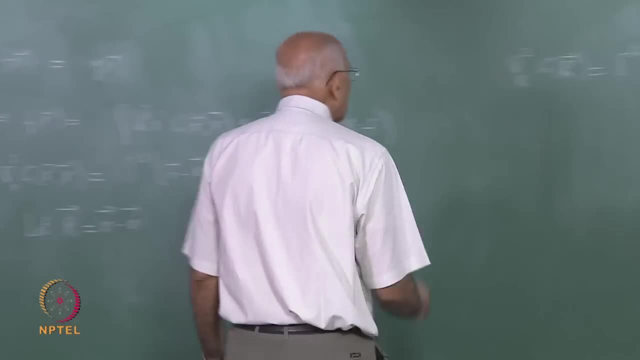 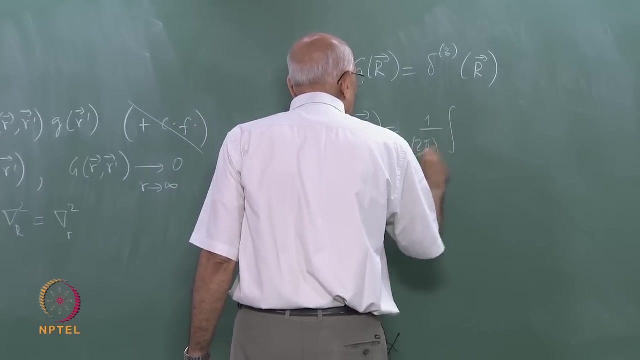 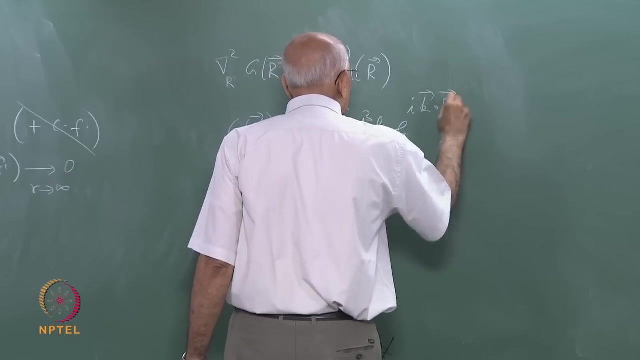 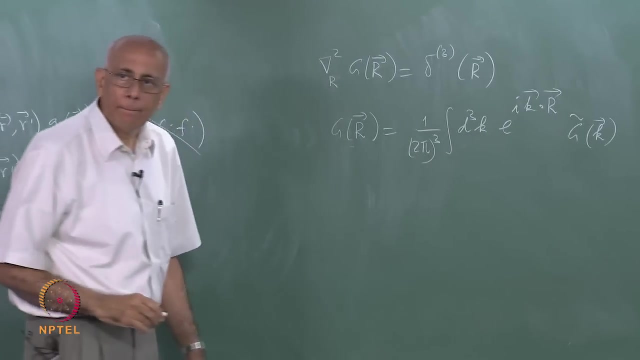 transform immediately. So let us define a Fourier transform. g of r, equal to it is in three dimensions: 2 pi cubed d, three k e to the power, i k dot r, g, tilde of k, And of course this is a inverse. 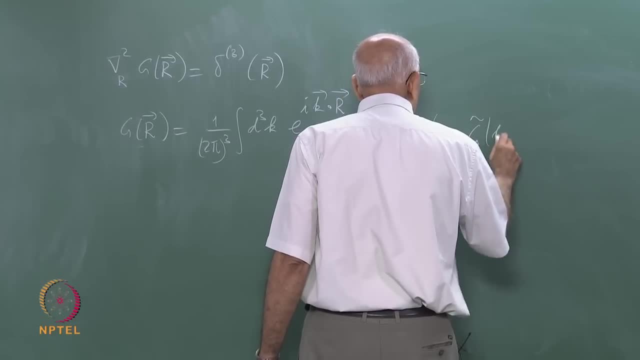 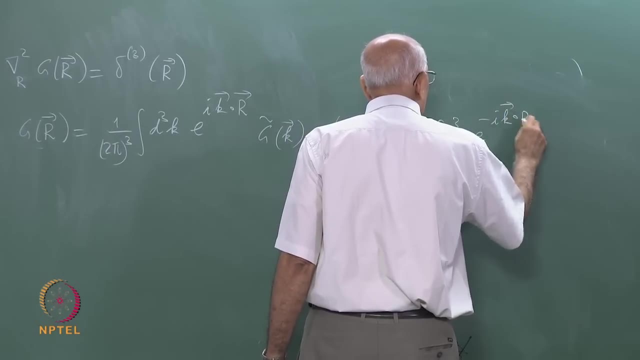 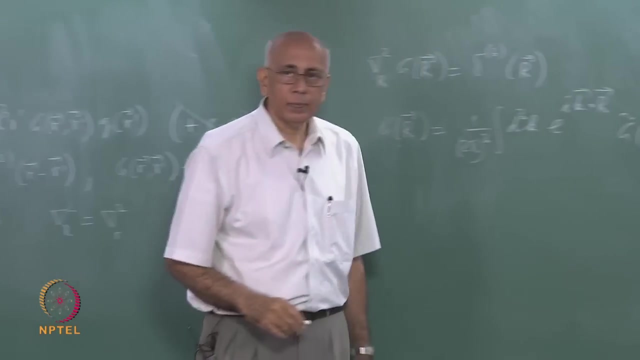 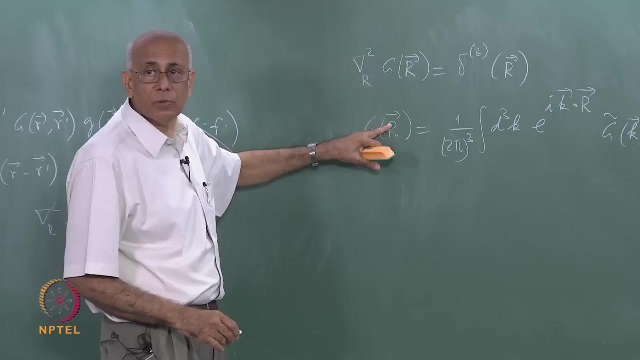 relation. this will also imply that g tilde of k equal to d, three r, e to the minus i k r, and let us put that in here. Let us substitute this representation for g in here. and the del r does not act on that, it acts only on: 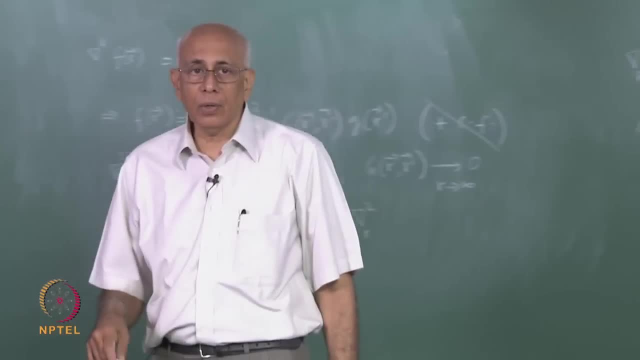 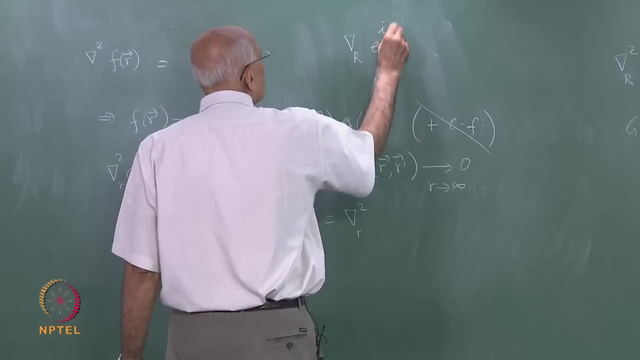 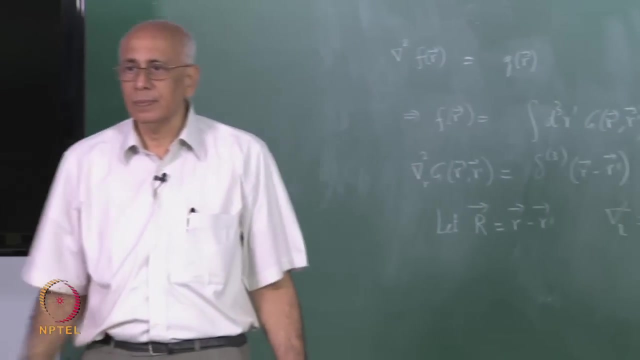 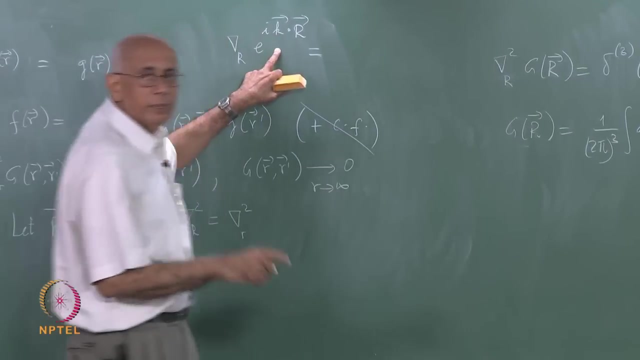 this. Now, what is del do when it acts on the scalar e to the i k dot r? What does that do? It just brings down an i k vector. all it does is bring down an i k vector. This is a plane wave. this guy is represents a plane wave, the. 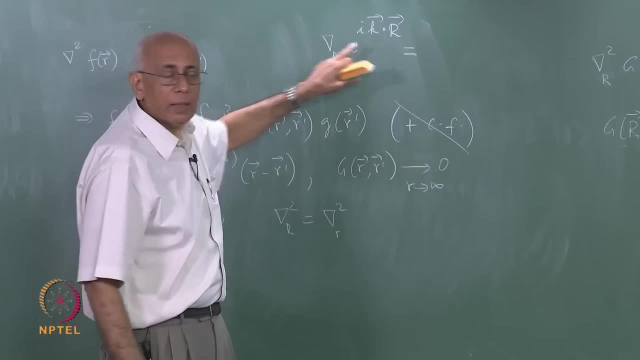 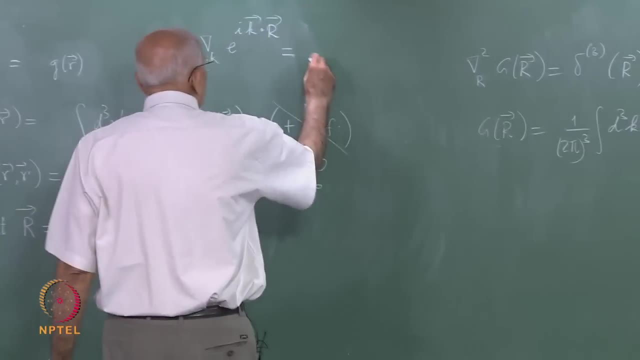 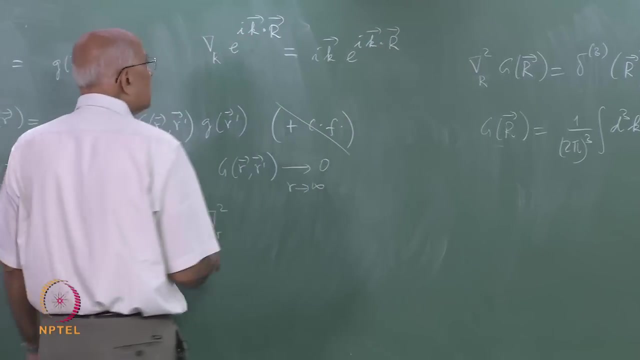 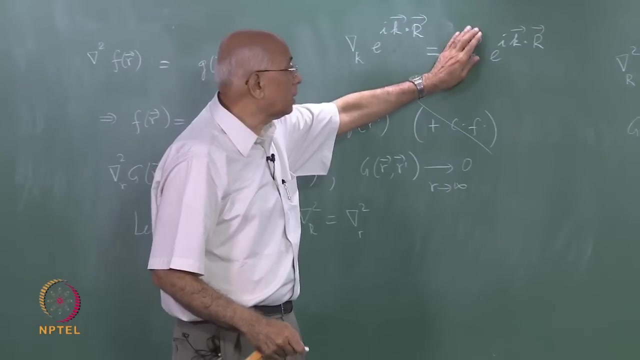 normal to the wave a plane is the k direction and the del always acts, is always in the direction of maximum rate of increase. So this is i k. So what is del square, del dot, this guy? So we got to do the divergence of this, but this is not dependent. 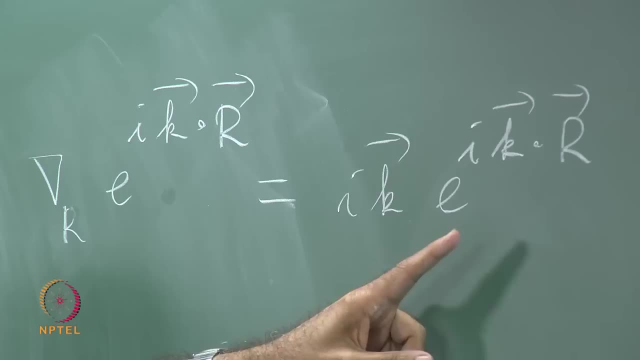 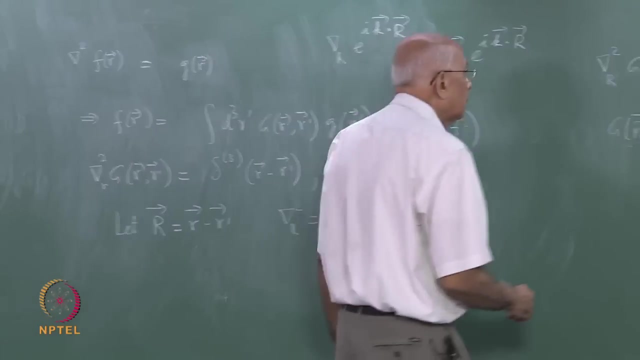 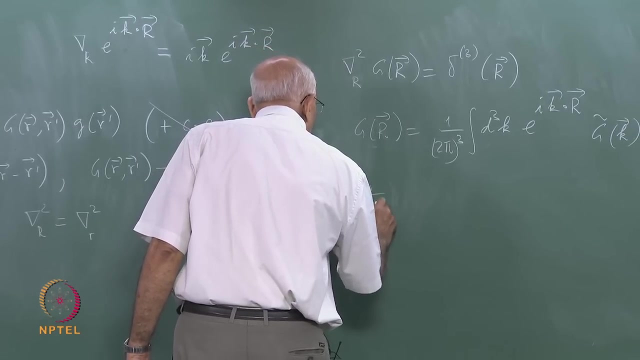 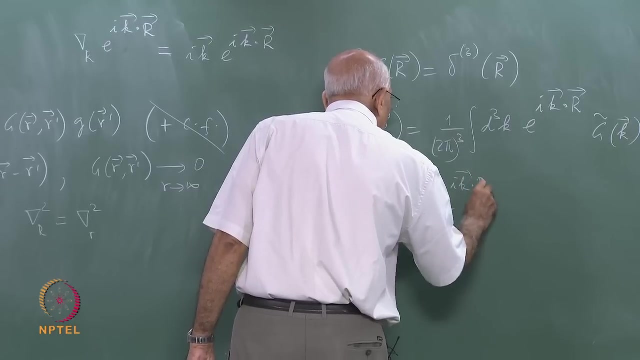 on r and get only the divergence, only the gradient of this once again. So it says del square is minus or whatever it is. So let us put that in right away. So this says 1 over 2 pi whole cube integral d, 3 k e to the i k dot r minus k square d. 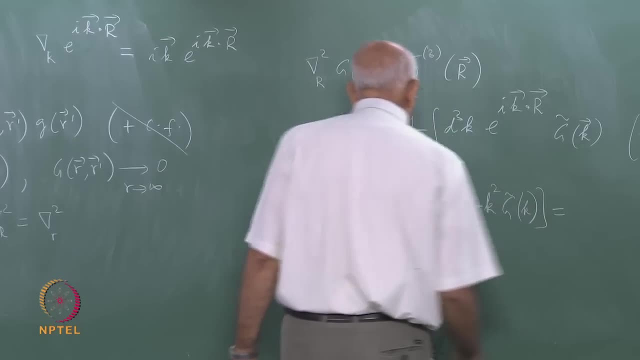 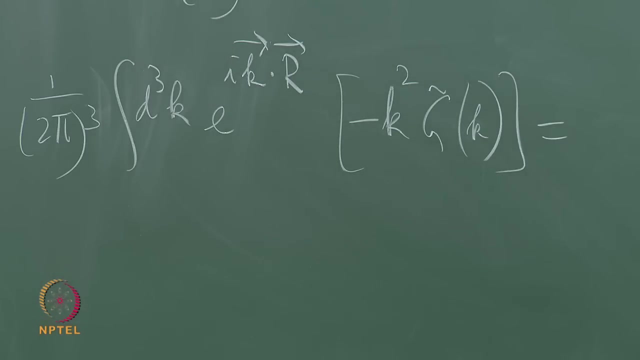 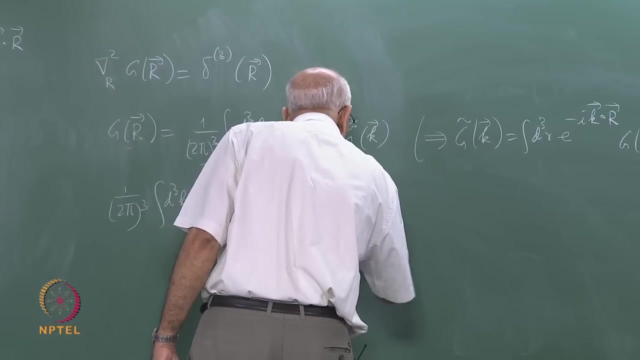 tilde of k is equal to, on the right hand side, the delta function. but we can write the delta function itself in terms of this exponential right. the delta function Fourier transform is just one, So you can write this as 1 over 2 pi whole cubed integral d, 3, k. 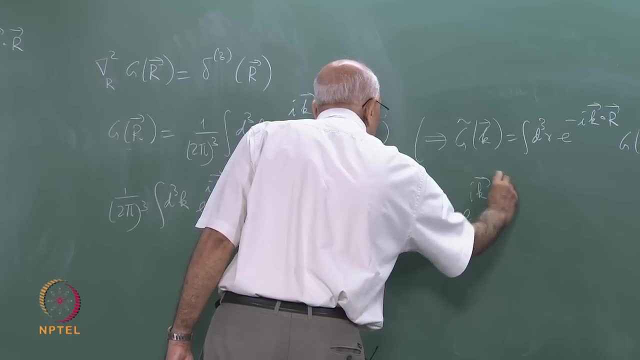 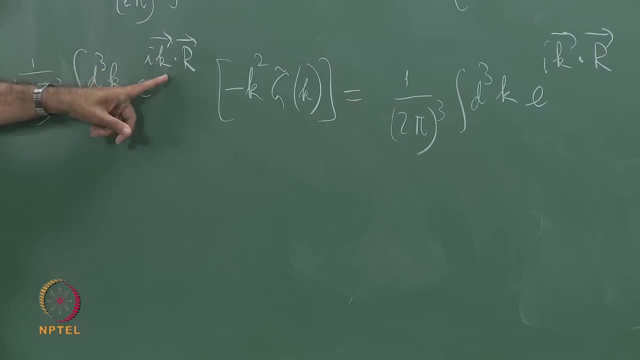 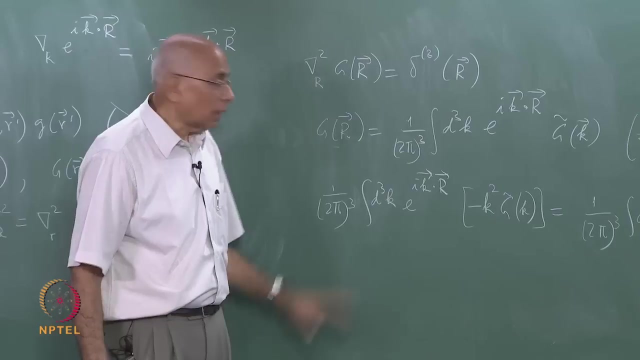 e to the i, k, dot r, And this forms a complete set of states for all k integrated over k, it forms a complete set of states in the r space, and you are equating these two ways. So, component by component, they must be equal. 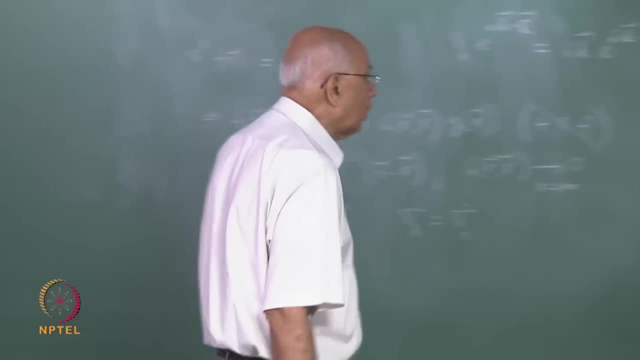 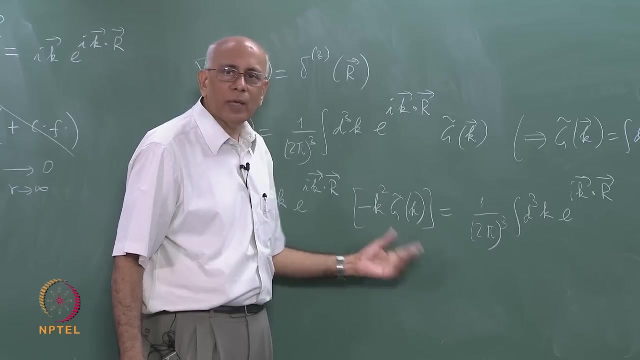 when you equate two vectors, they are equal component by component. So the coefficient of each i to the i k dot r on the two sides must be equal, which says minus k square g, tilde of k must be equal to unity. So you got g. 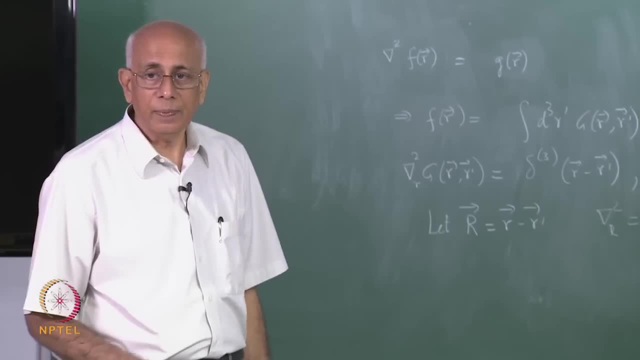 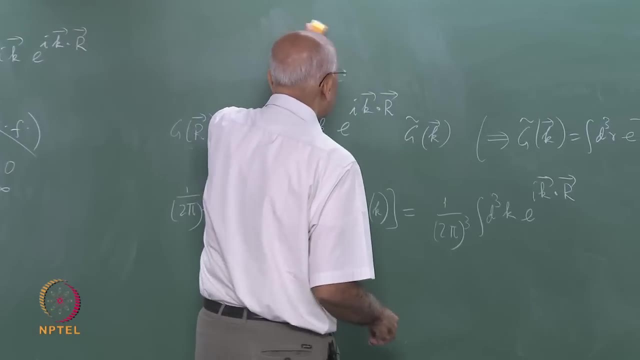 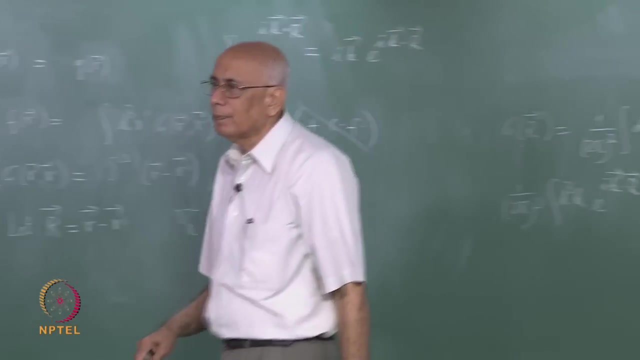 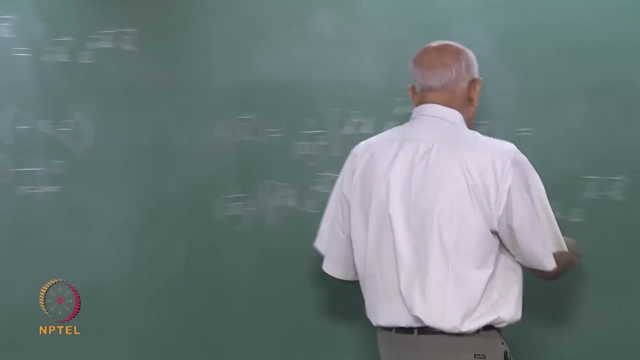 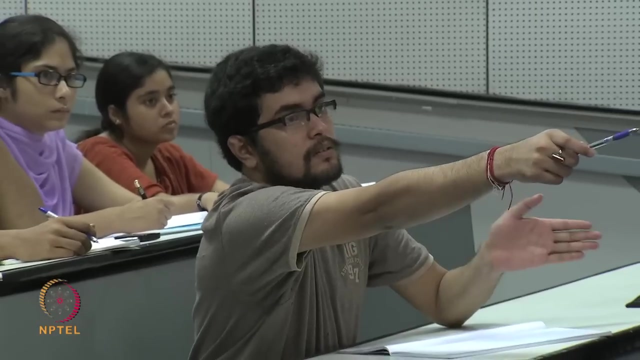 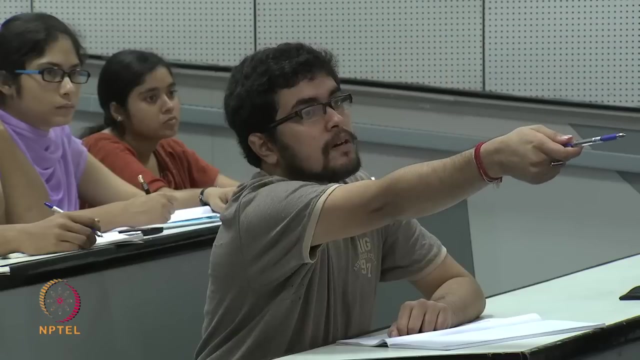 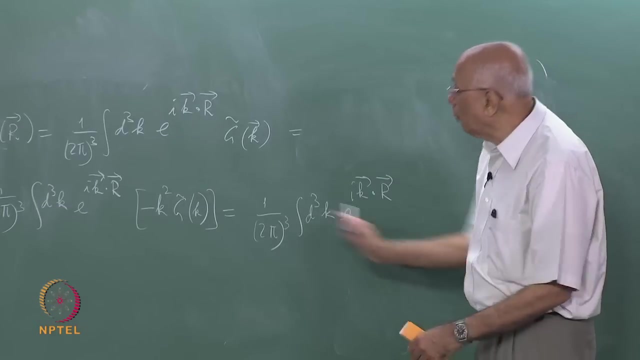 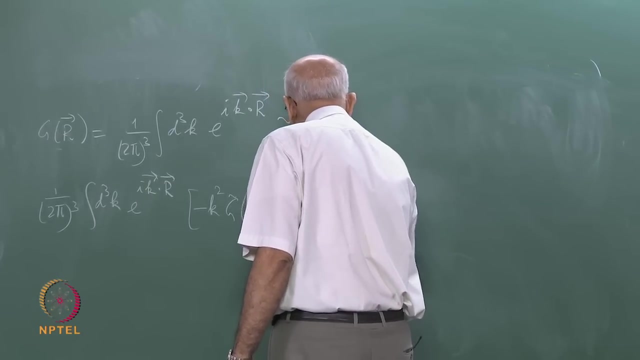 tilde of k is minus 1 over k square. that is it so immediately says. I wrote: this is the delta function. this is the three dimensional delta function. So if I move this to the left hand side, it says this: minus 1 is equal to 0.. So it says a. 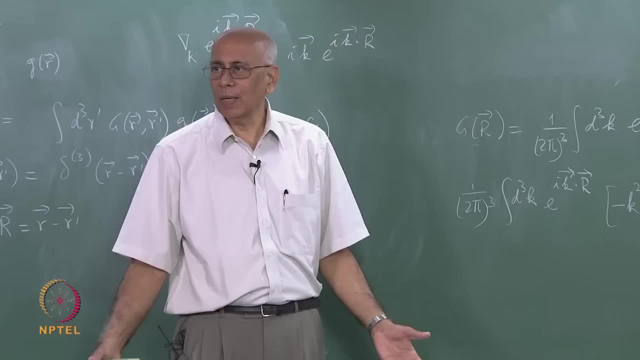 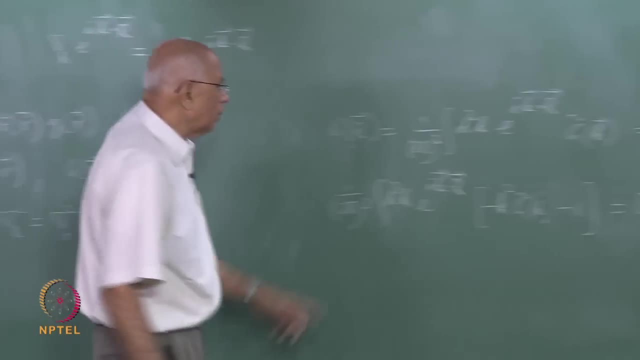 certain vector, certain function is 0, identically. and when is a vector 0, when every component is 0. And what are the unit vectors in this problem? e to the i, k dot r. So this is the total vector and this is the function space. they are the unit vectors and for 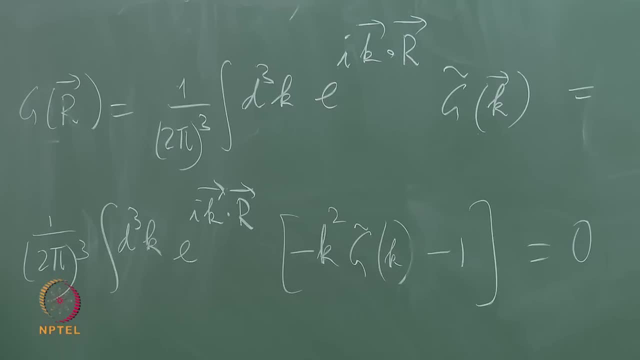 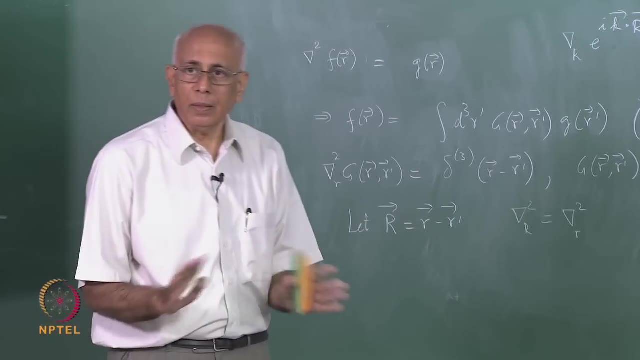 every k. this quantity must be 0, that says g tilde of k is minus 1 over k square. So the argument is completely rigorous but it has to go. you have to go through it. The reason you can equate Fourier coefficients is because 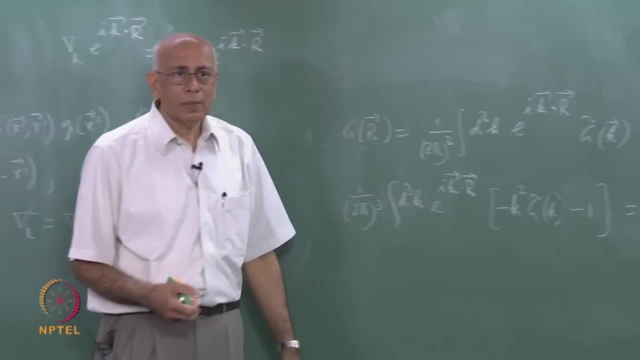 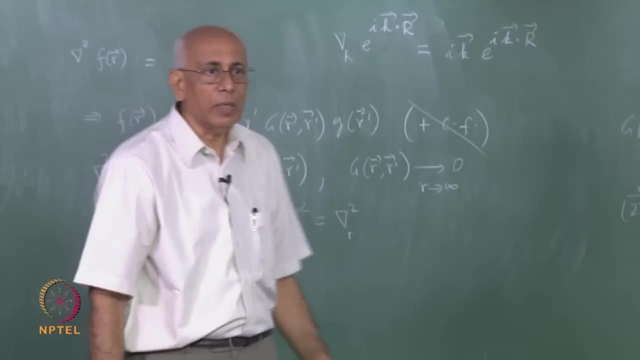 these things form a complete set of states And therefore you can bring everything to the left hand side and say a certain vector is 0, which means every component is 0. So 0. So each Fourier component must be 0. And therefore, once I put that in here, this is: 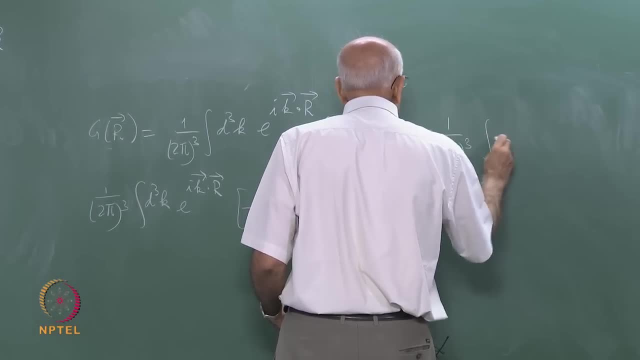 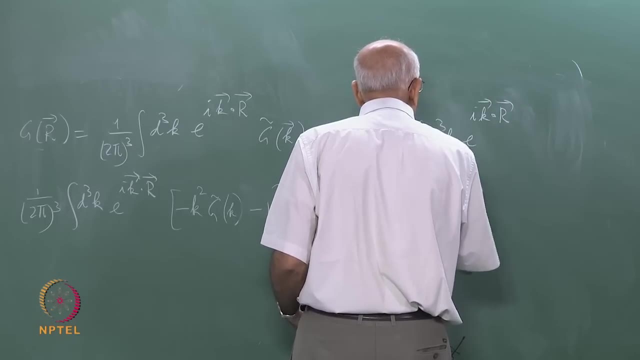 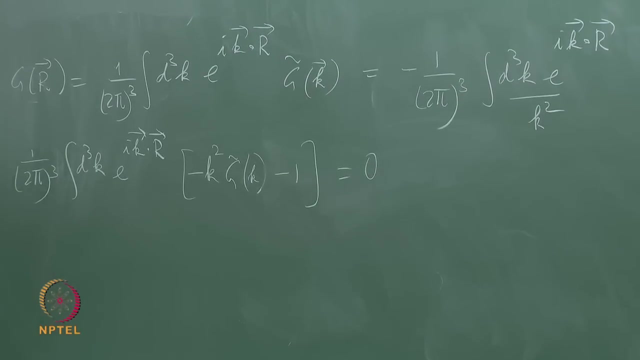 minus 1 over 2 pi 4 cube. integral d: 3 k e to the i k dot r over k square, that is g of r. If I can evaluate that integral, then I got an expression for g of r. I put that back in g of r. 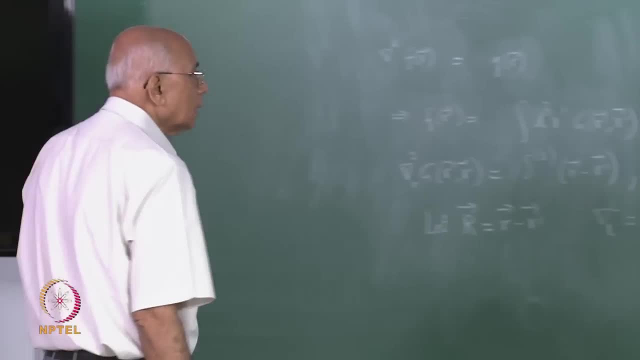 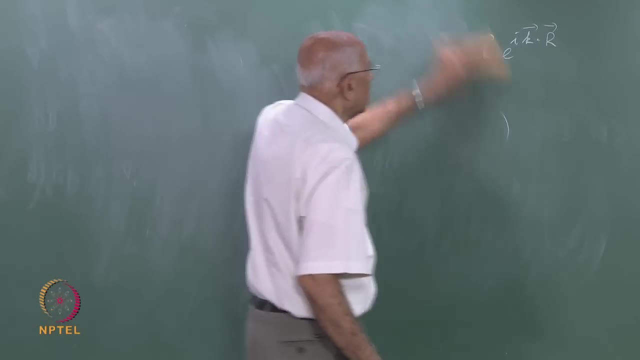 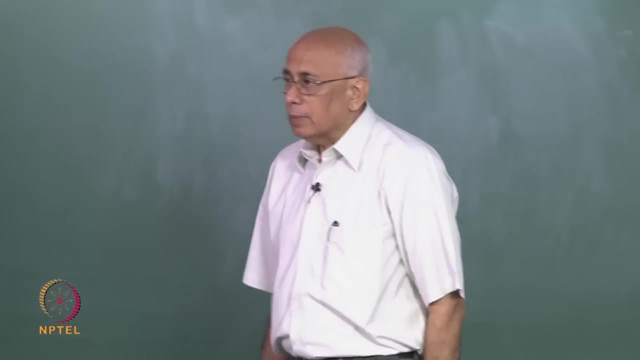 comma, r, prime, and that is it that gives me the fundamental green function. So let us see how to do this integral. what would you do to tackle such an integral If you took an arbitrary coordinate system? you are in deep trouble because this means k vector point somewhere and you have to integrate over all. 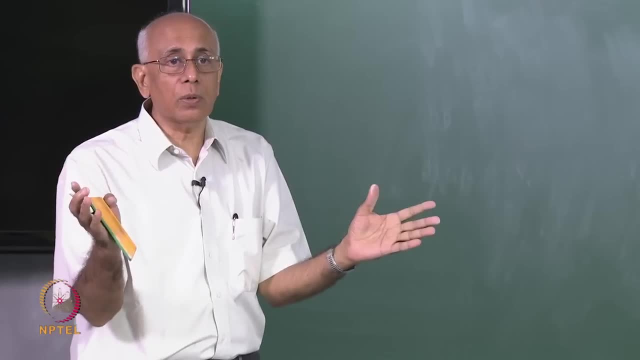 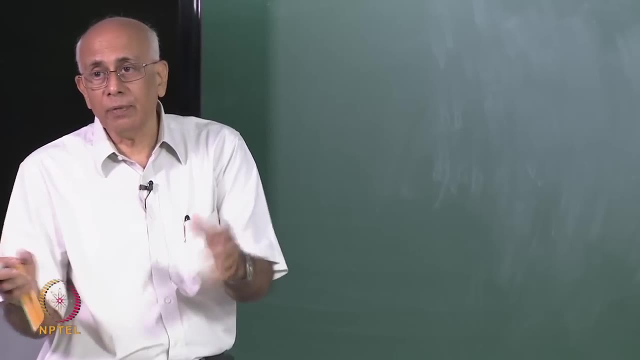 directions in k, the r vector point. somewhere else you have to integrate over all directions in k, the r vector point. somewhere else you got to integrate over all the angle between the two, because e to the i k dot r as e to the i modulus k, modulus r, the cosine of the angle between them, And that is a big nuisance. 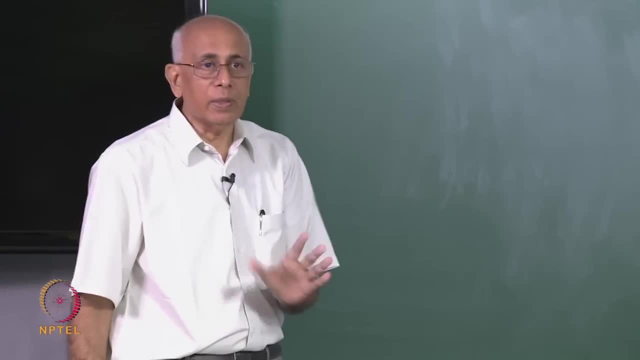 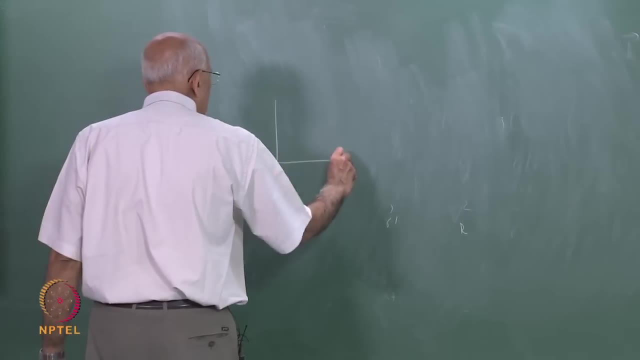 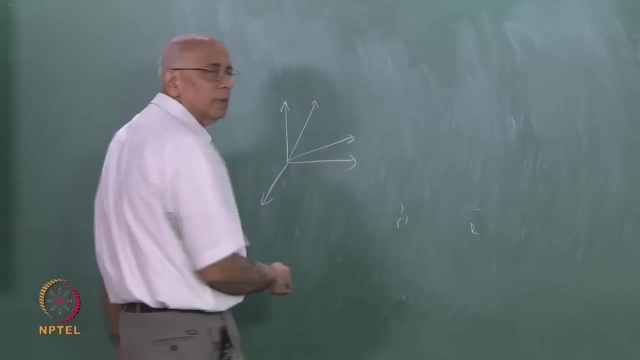 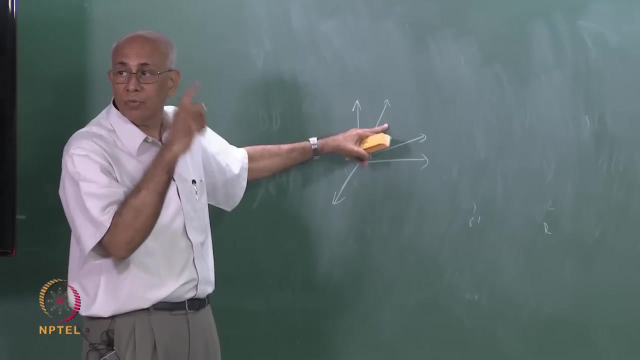 that is a terrible nuisance, is not trivial to do this integral at all if you are going to do it the hard way, Because if you take two arbitrary vectors, if you took some vector like this and some other vector like that, this is got some polar coordinates r theta phi, say, and this is got r prime theta, prime phi, prime, etcetera. 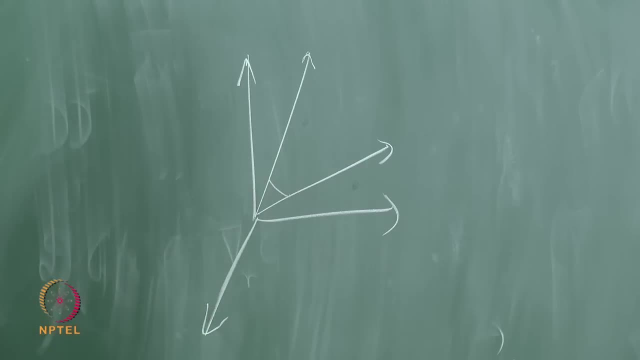 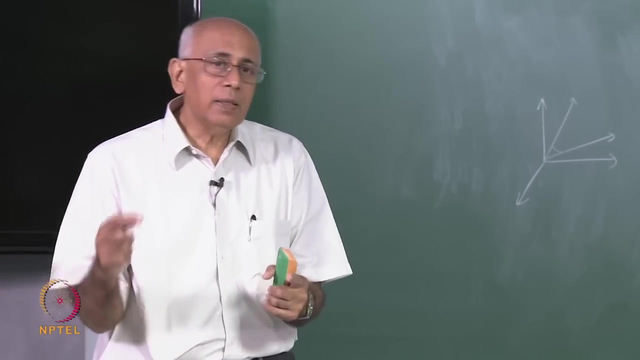 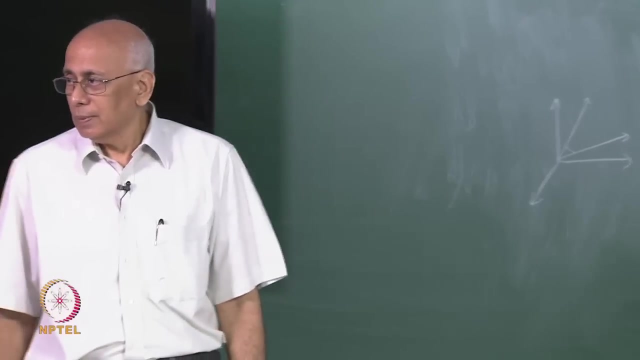 We are asking for the angle between these two guys, the dihedral angle between these two vectors. you can rewrite that. you can write this angle in terms of the polar coordinates, a polar angles for each individual vector. It is called the law of signs or some such. 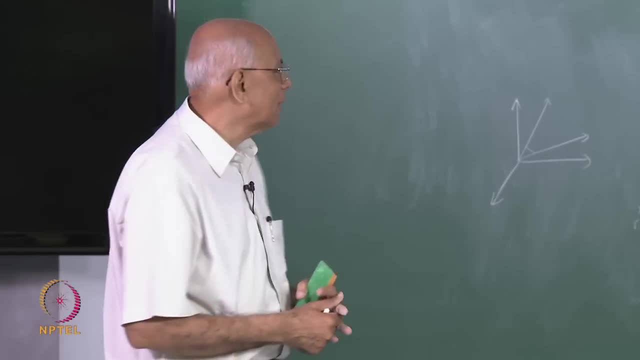 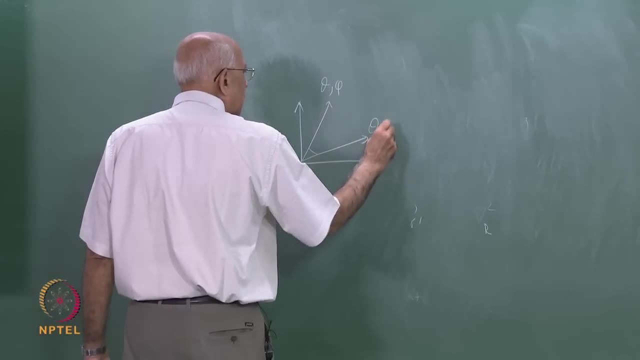 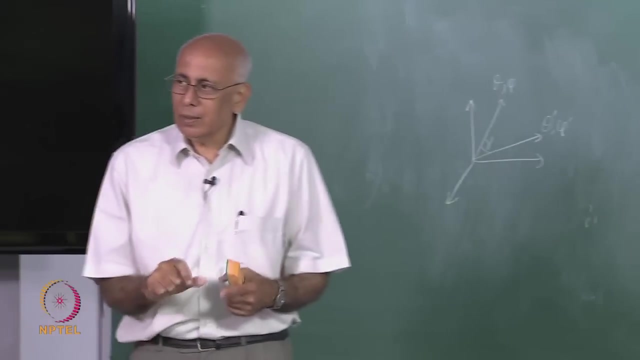 thing, it is standard problem. I do not know if that is learned by people, but if the coordinates here are theta, phi and the polar coordinates here are theta, prime, phi, prime, and this angle is gamma, then there is a relation which is essentially the addition theorem for the Legendre function of order. 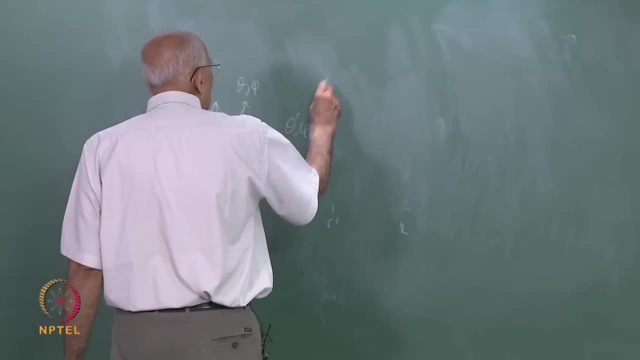 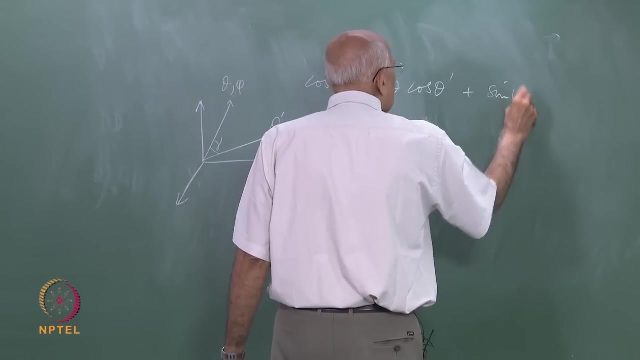 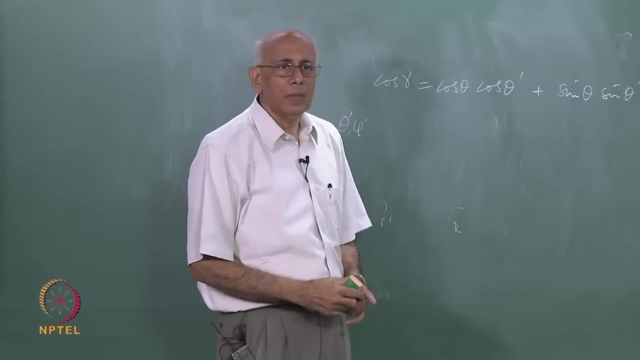 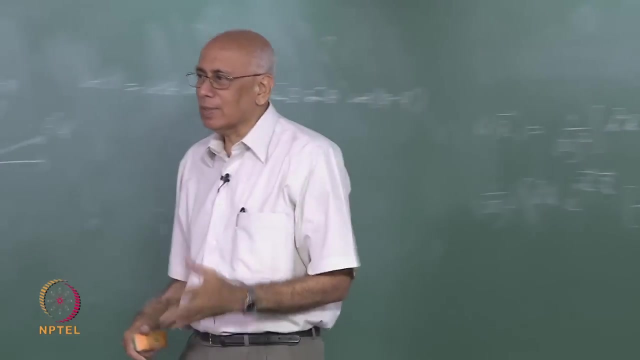 one. So it says something like cos gamma equal to cos theta, cos theta prime plus sin theta, sin theta prime, cos phi minus phi prime. So you have to put that in here and then integrate over theta prime and phi prime, which is a terrible job. it is horrible. So that is not. 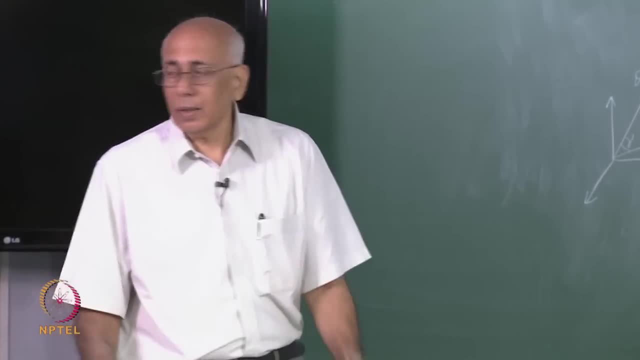 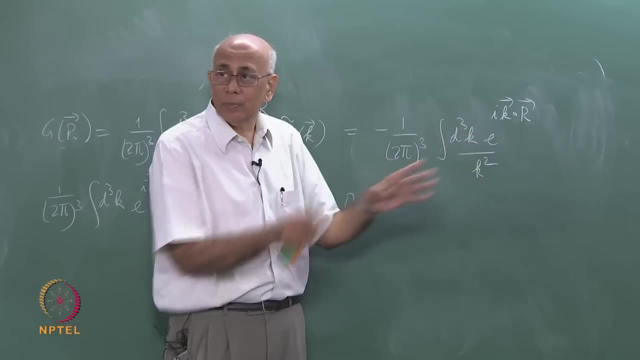 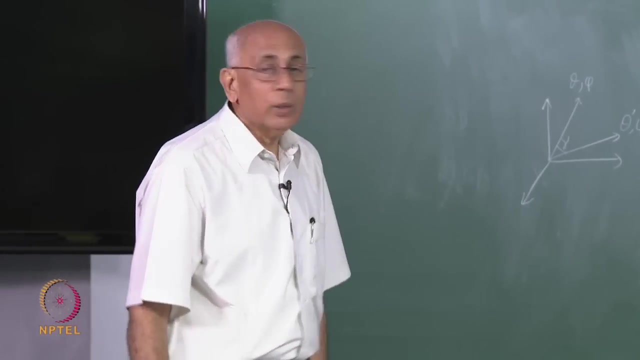 the way to do it. you could ask: can I do it in Cartesian coordinates? well, you could in general, except that you have this factor sitting here. otherwise this itself will be a product. So you could do this in Cartesian coordinates, but doing it with this k square is again a big problem. So what should we? 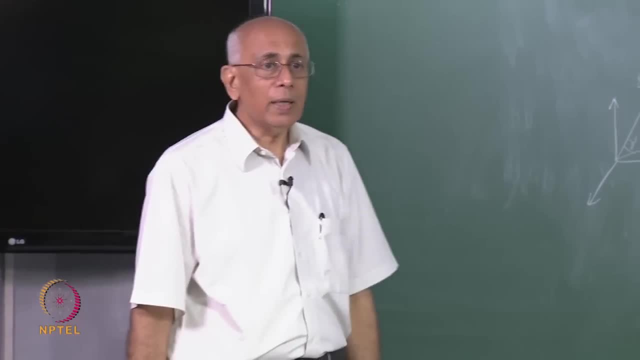 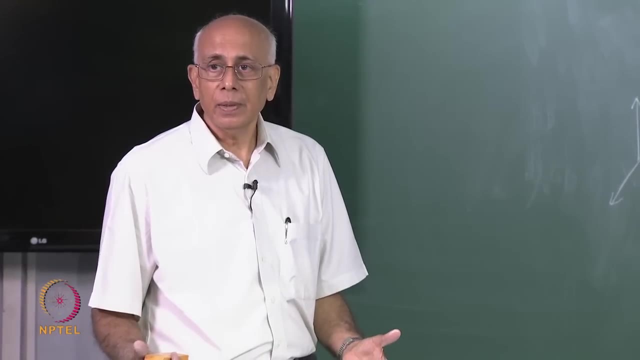 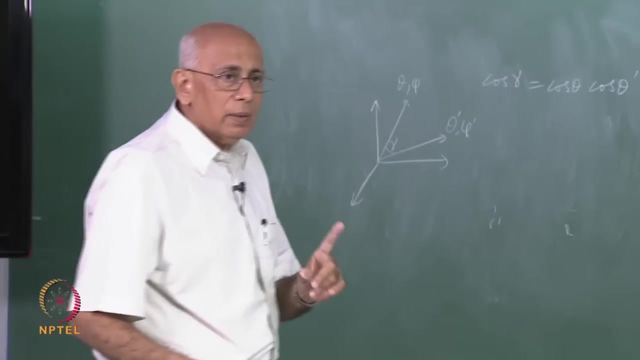 do. we should clearly look at some invariance of this quantity here. this g of r, it is a scalar in the fact that it is a scalar means it is invariant under rotations. So you could actually choose your coordinate system as you please. you can choose the polar axis of 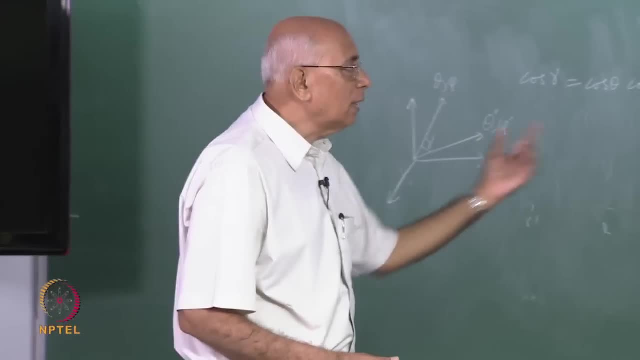 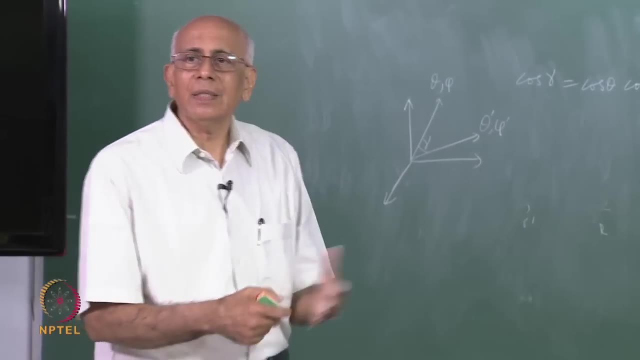 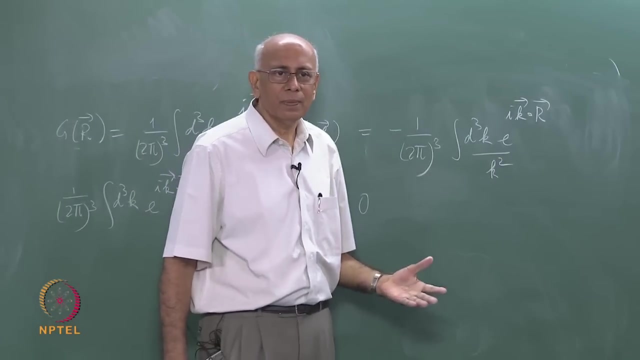 your coordinate system as you please And given any other choice. you can bring it to this choice by a change of variables in the k space. Now, what is this? what is the vector sticking that sticking out? k is integrated over. So what vector is sticking out? r vector. So let me choose the polar. 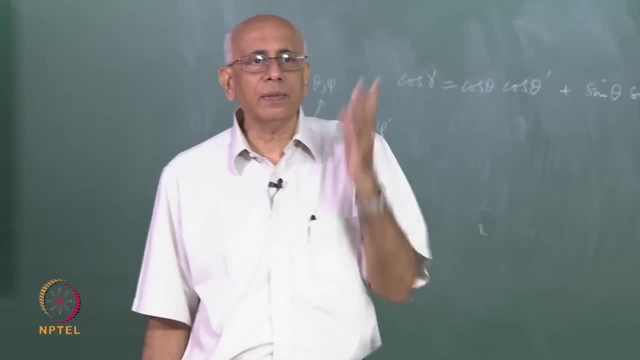 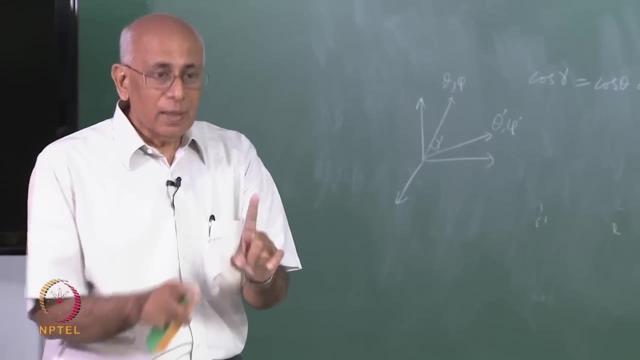 axis in k space along this vector r. you can do that, you can always do that. So once I do that, Then the polar angle of k is just cost theta, there just a theta, and E to the i k dot r becomes. 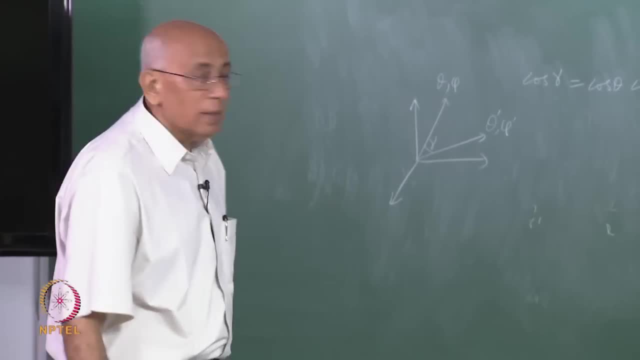 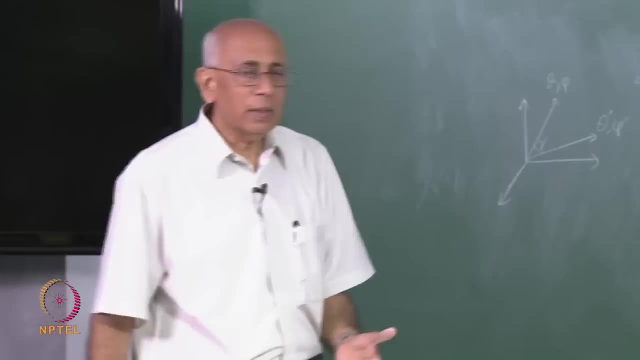 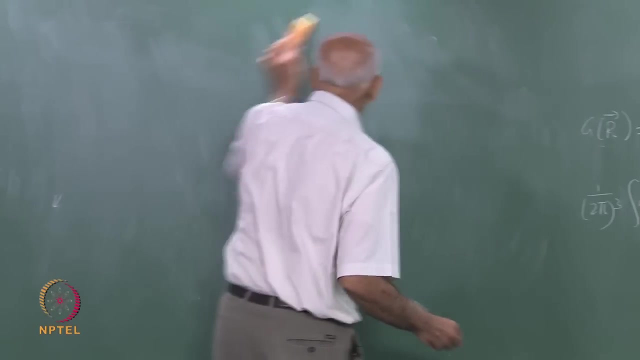 E to the i k r causta is that five dependence. So I can integrate of five what is the integral of five. give you gives your two pi. So this immediately means that you can, in case space, choose this access along the direction of. 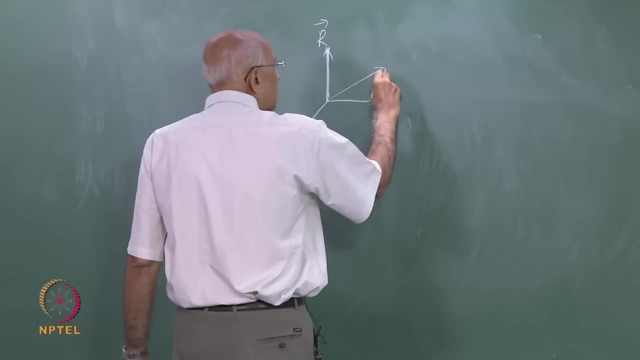 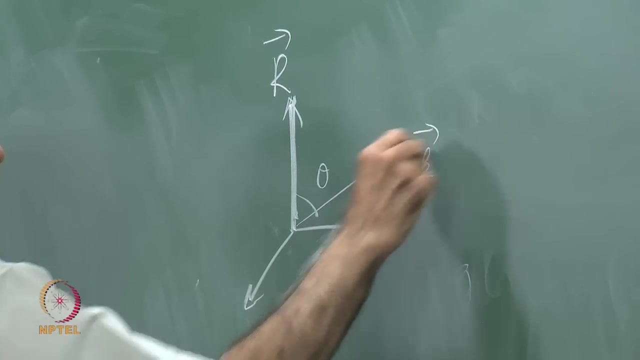 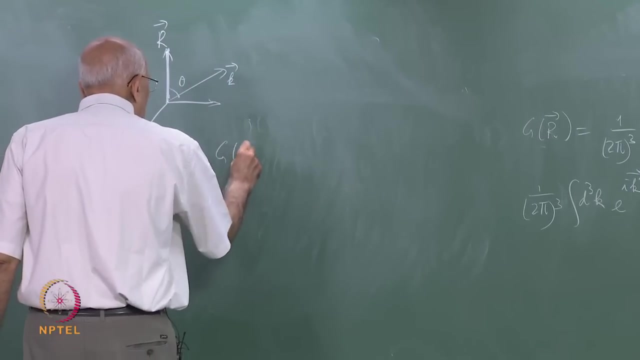 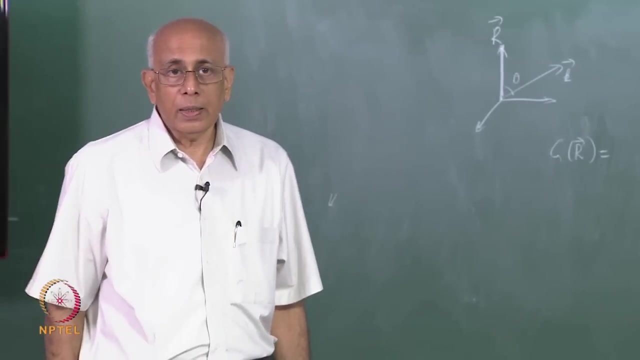 of r, And then k is integrated over all directions, but this angle is theta here and this is the typical k. So this integral becomes g of r, equal to. by the way, I said that this function is a scalar, So I really expected not to depend on the direction of r either. it should. 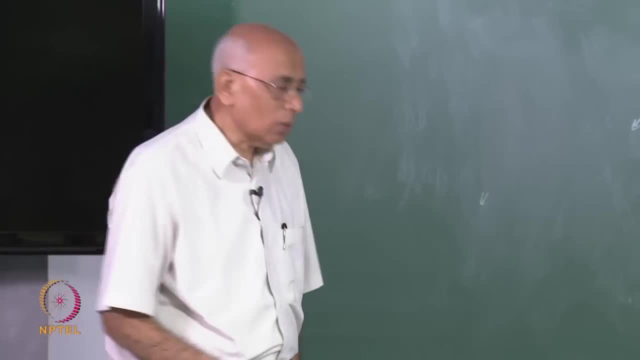 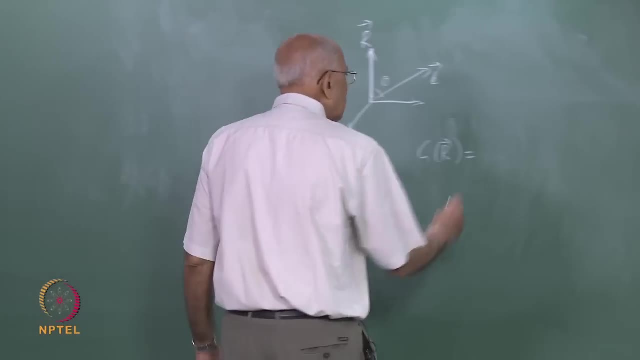 finally end up depending only on the magnitude of this r right, So I could write g of capital R without the vector sign, but we will see that really comes out or not. So this is equal to minus 1 over 2 pi whole cube integral. 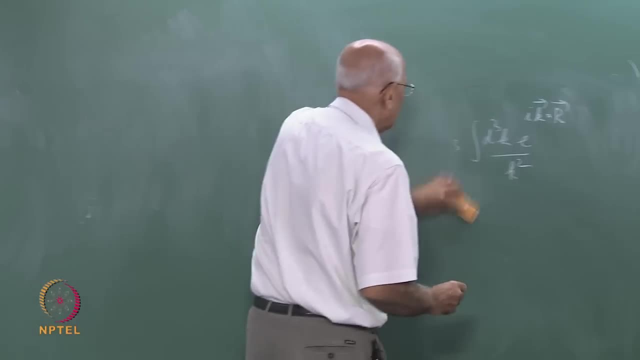 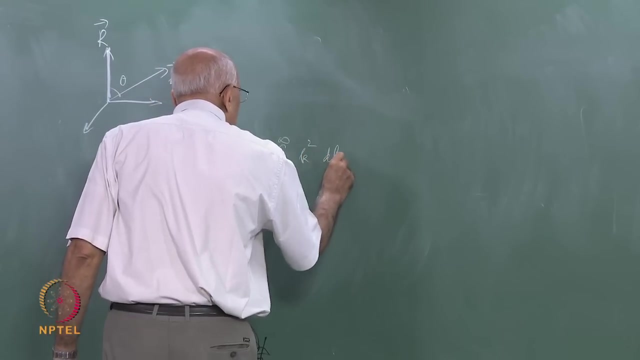 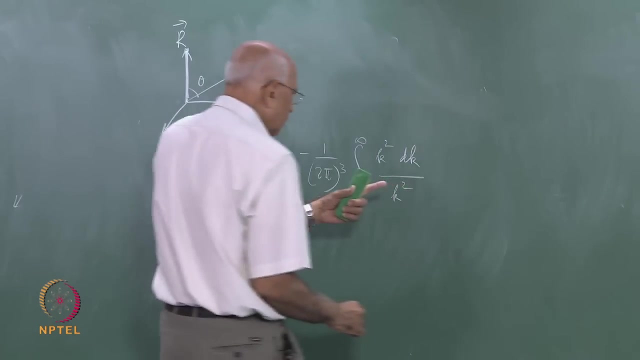 0 to infinity, k square, d, k. but there is a k square in the denominator, which obligingly cancels out. And then there is a 2 pi from the pi integral, So this becomes a 2 pi square and I have 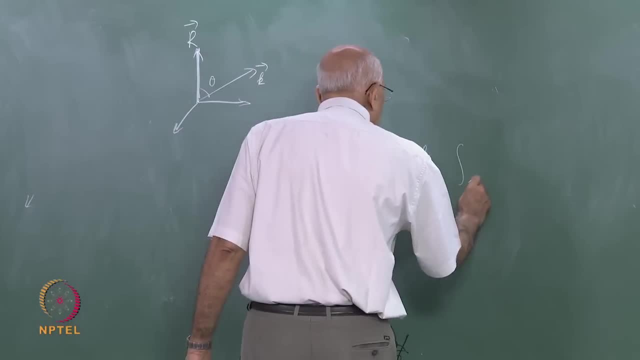 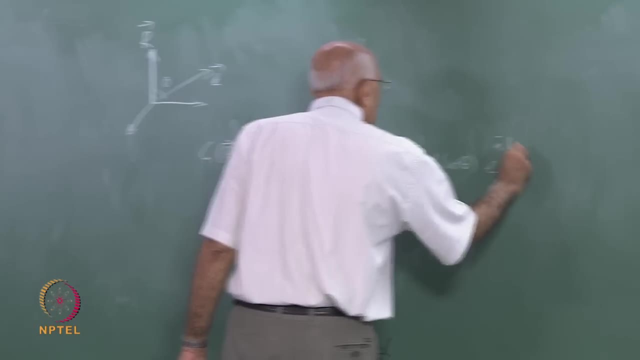 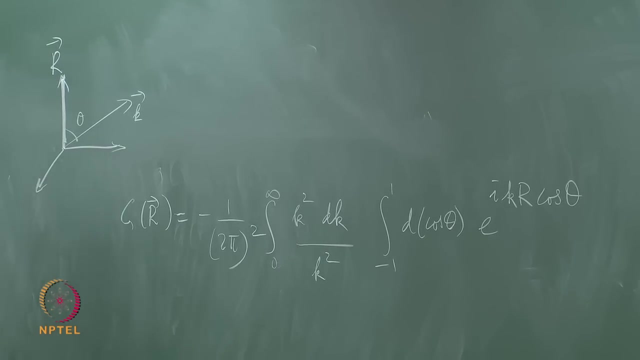 done the pi integral on the pi integral now and then I have an integral over the theta which is minus 1 to 1 d cos theta, e to the i k r cos theta. I change variable to cos theta is running from minus 1 to 1.. 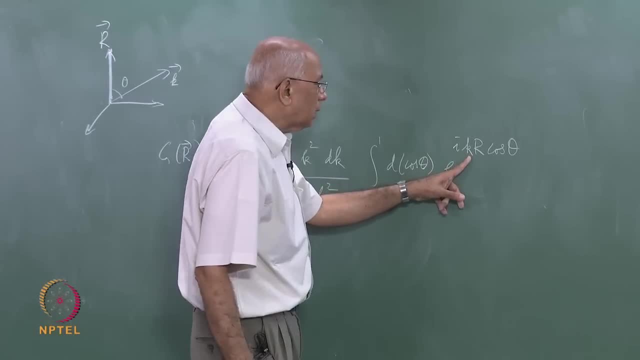 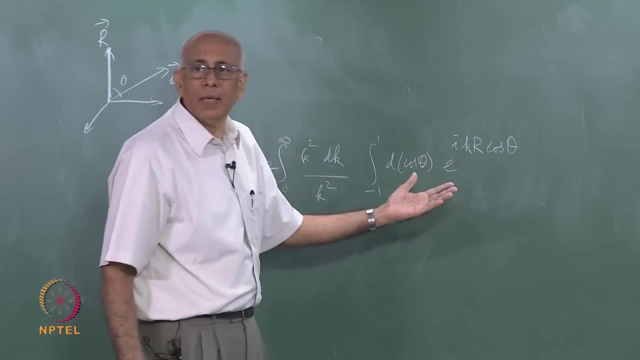 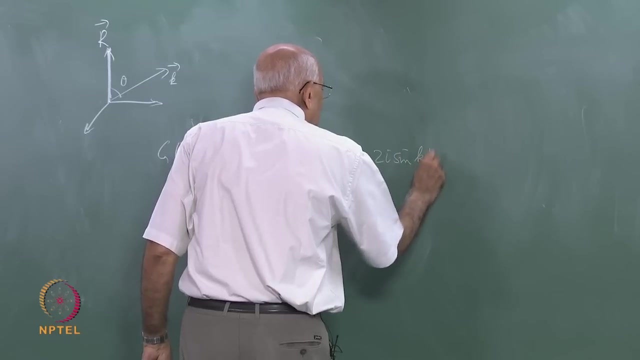 So this thing gives you e to the i k r minus, e to the minus i k r over i k? r, But the numerator is 2 i sin k r. So I get rid of this and write this words: 2 i sin k r. 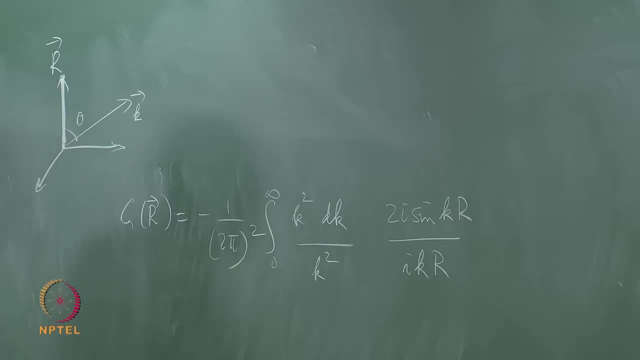 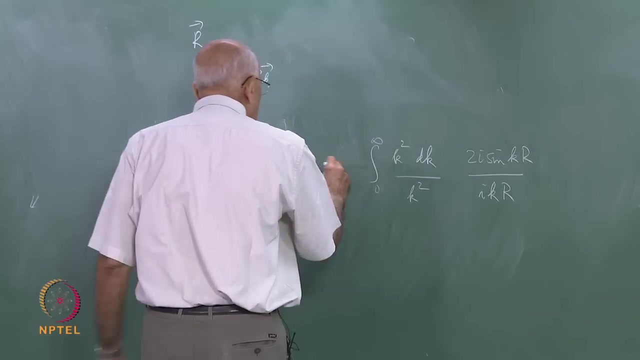 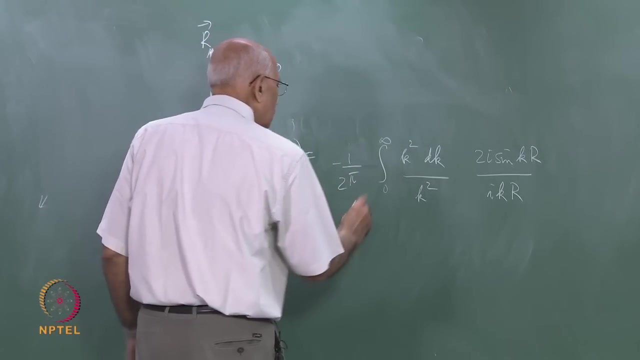 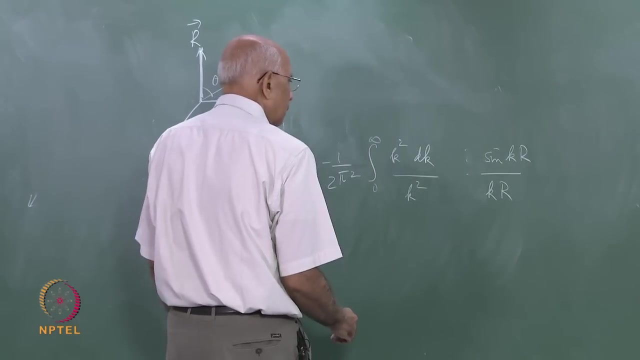 over i k? r. So this is 4 pi square. let us make it a minus 1 over… 4 pi and there is a 2.. So there is a 2 pi square. the 2 cancels the i cancels by the. 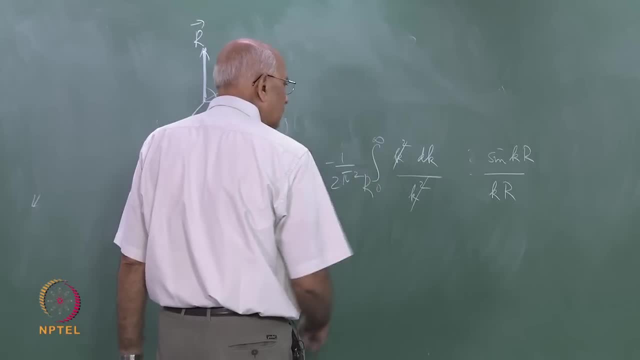 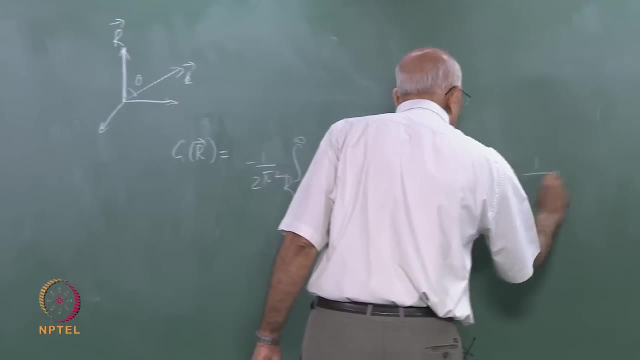 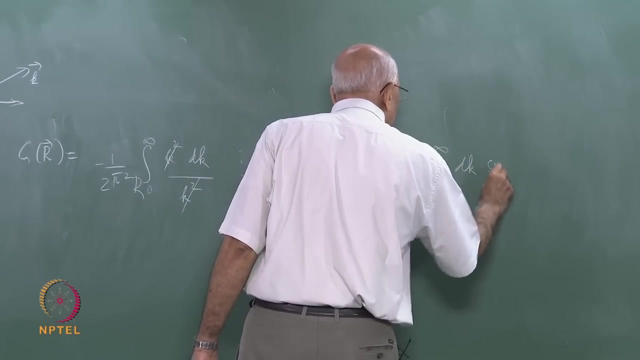 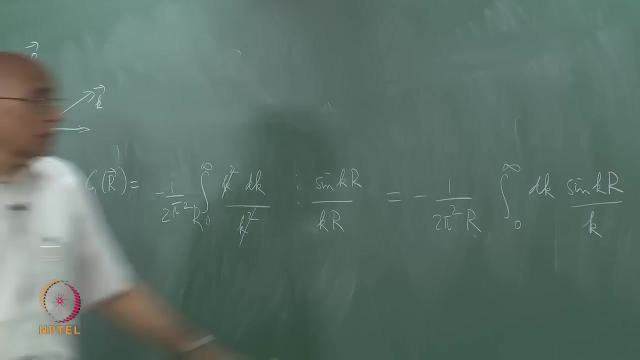 way the k square cancels, the r comes out and you have d k sin k r over k. So this is equal to minus 1 over 2. pi square capital r integral 0 to infinity. d k sin k r over k. that is it, but this is the directly integral capital. 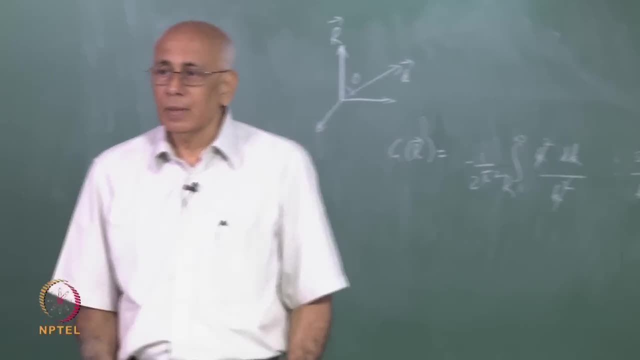 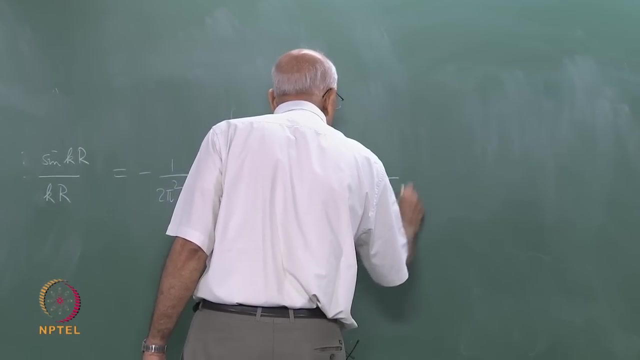 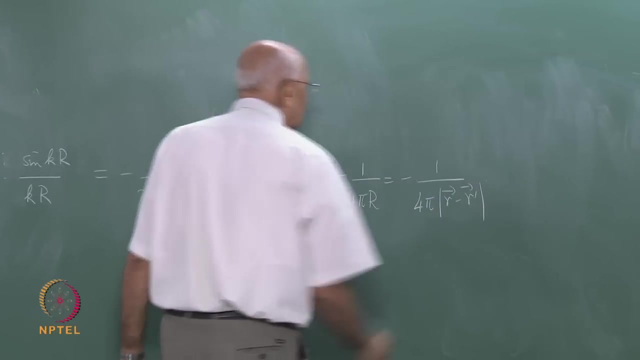 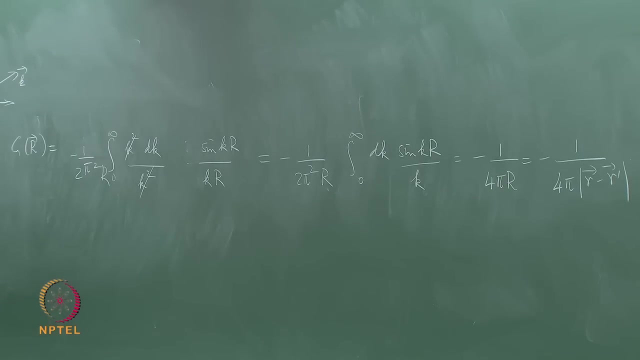 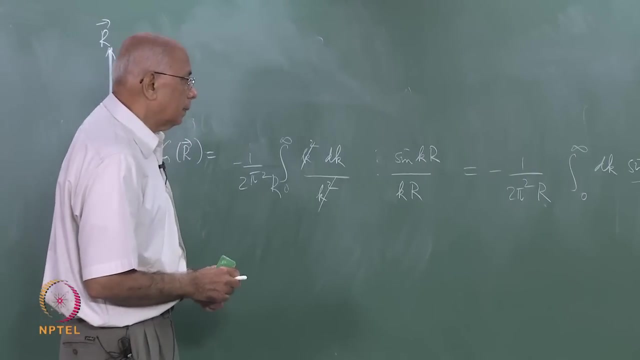 r is positive. So what is the value of this integral pi over 2.. So this gives you: 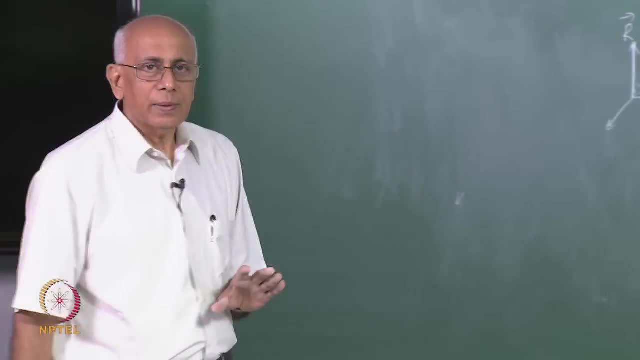 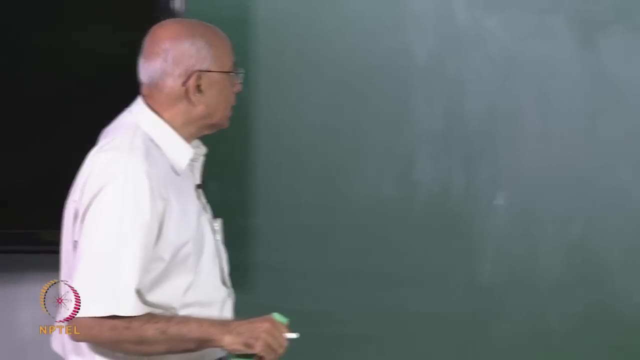 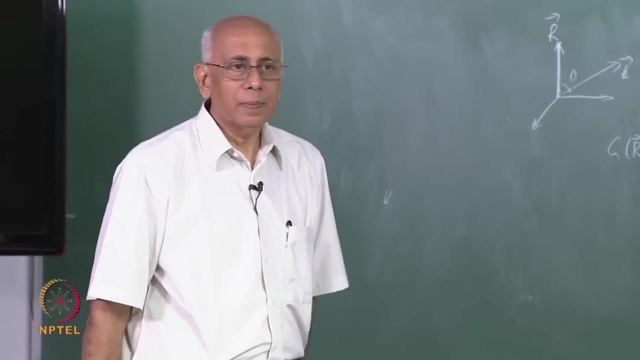 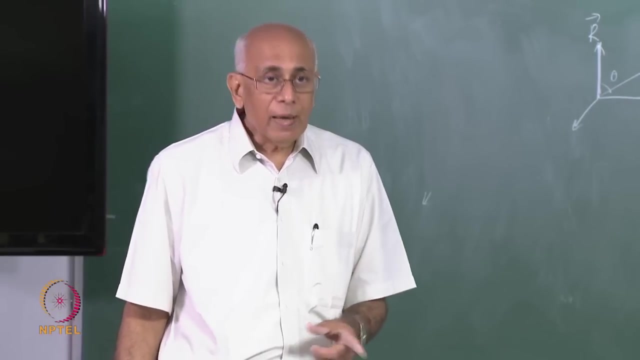 accident. Coulomb's law is directly a consequence of the fact that the operator is del square. So very often you see the statement that the green function for del square is just the Coulomb potential. In fact, you could define the Coulomb potential in an. 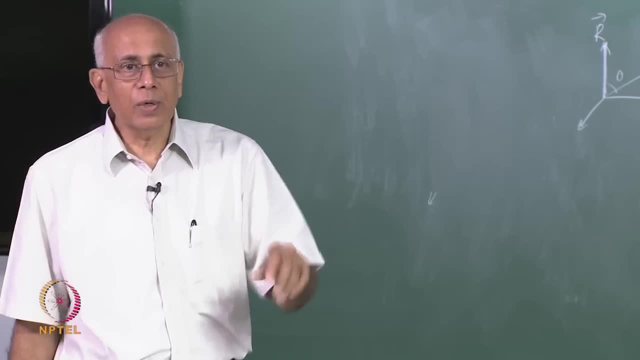 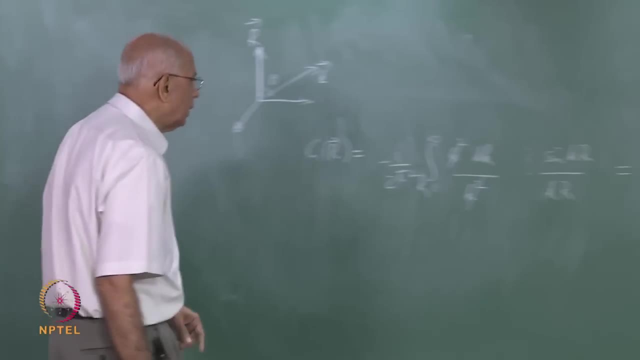 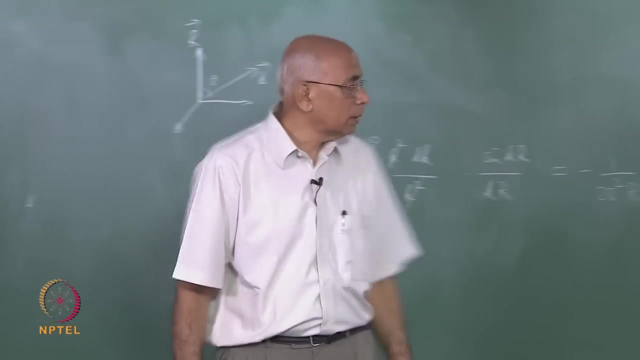 arbitrary number of dimensions, as the inverse Fourier transform of 1 over k square or as the green function, free green function- of the del square operator. We will do that very shortly, but I want you to see how this 1 over r minus r prime modulus has emerged. 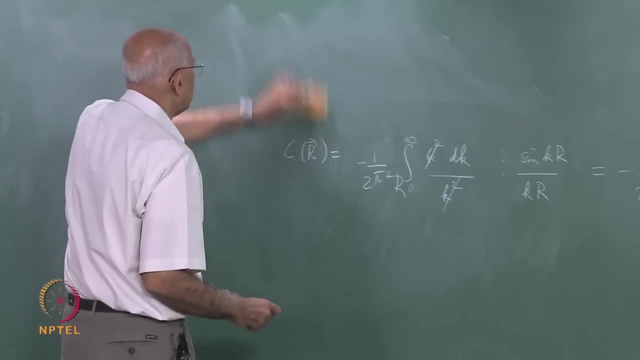 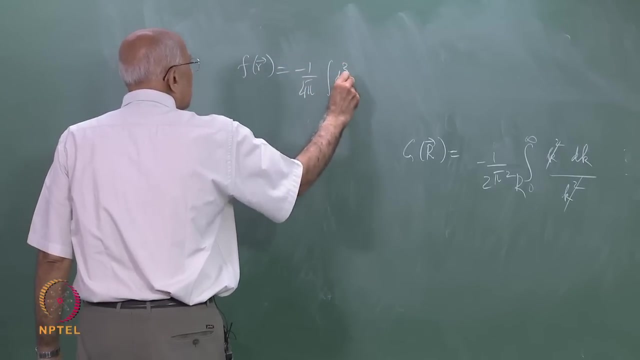 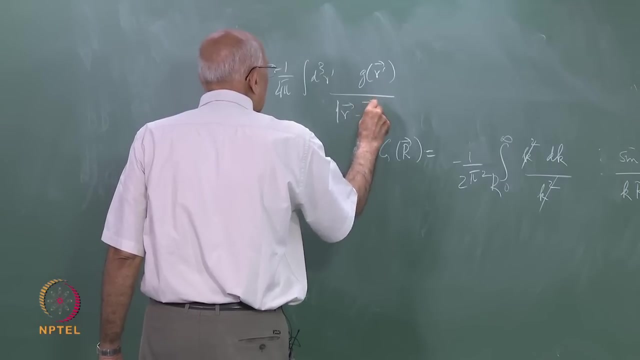 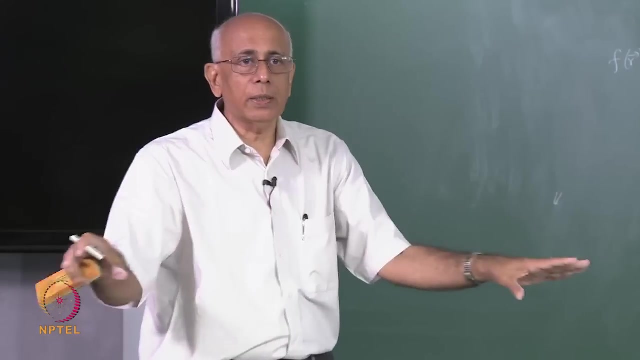 And rest of course. the rest of course follows Now. you can write: f of r equal to minus 1 over 4 pi. integral d 3 r prime. g of r prime over mod r minus r prime. Plus of course the complementary function. but I took the boundary condition that this: 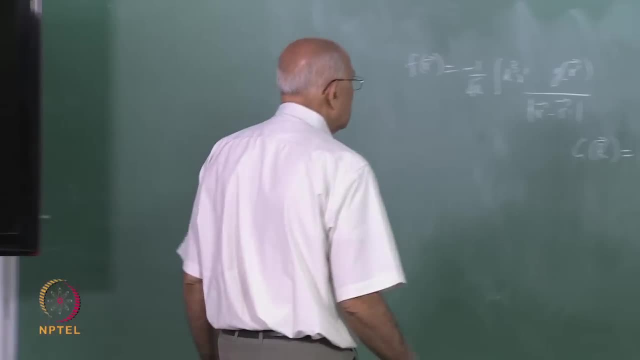 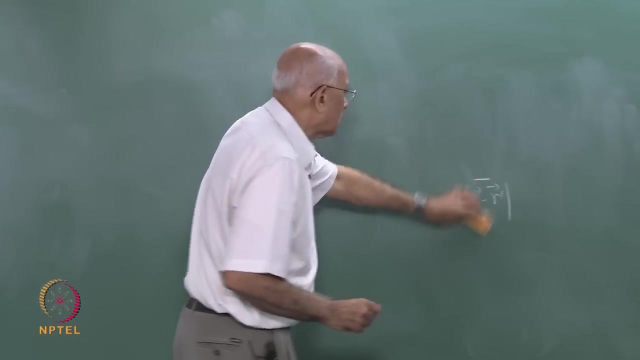 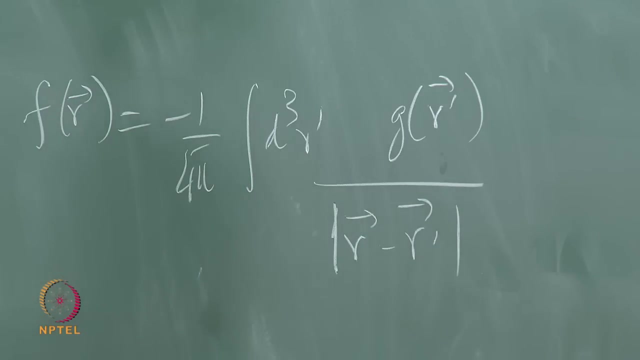 went to 0 at infinity, and then this is the solution. Now, of course, you can look at various special cases. You could ask what happens if this is a function only of magnitude, If it is a charge density, for example. what happens if it is a spherically symmetrical? 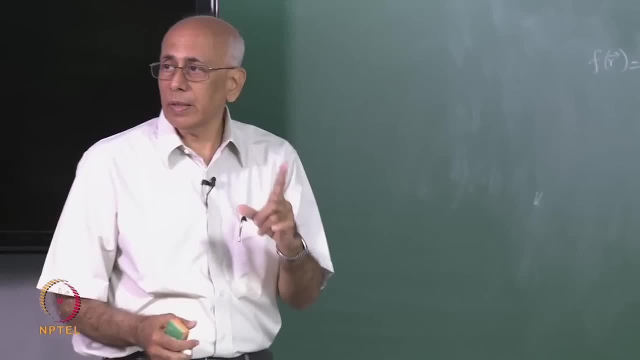 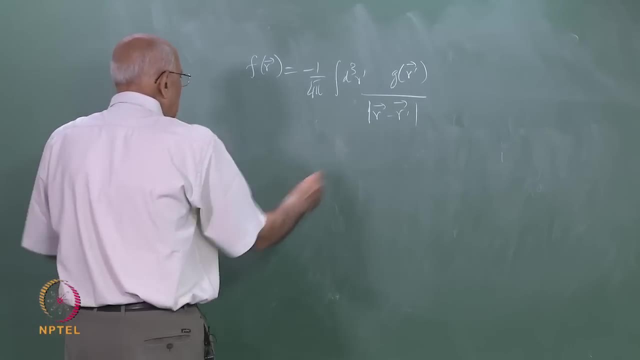 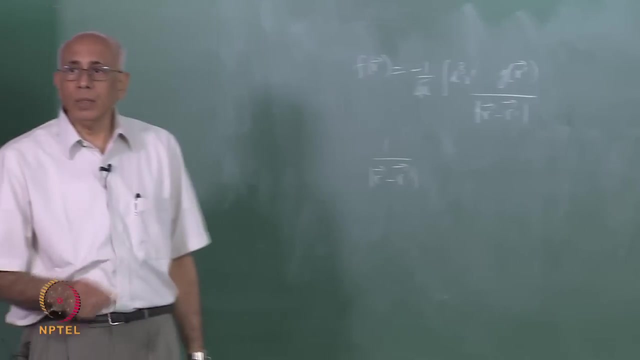 charge density. So it depends only on the vector, the magnitude of the vector, r prime, and so on. All these cases can be looked at and all of you, I am sure, familiar with the fact that this quantity here, 1 over mod r minus r prime, is called the colon colon, for obvious reasons. 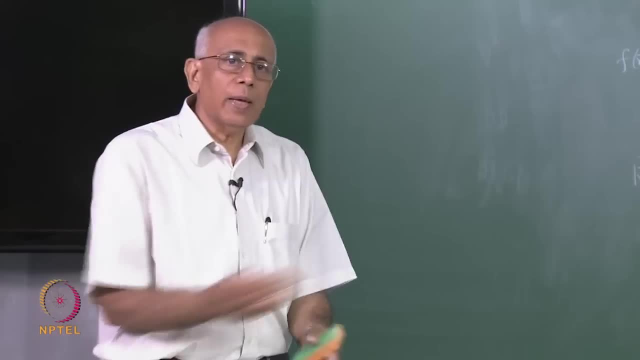 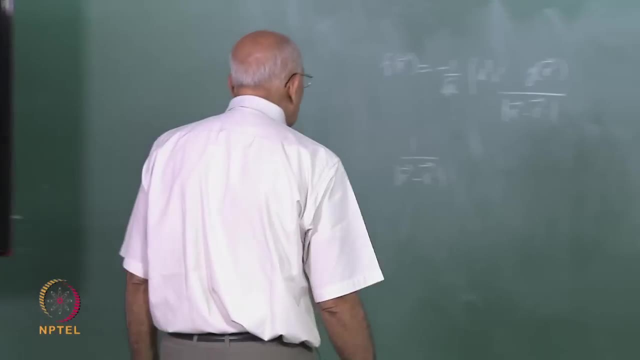 and you normally, when you do these multiple expansions, you expand this guy in powers of r over r prime or something like that. And what is that series look like? Well, there is a famous series which goes like: summation l equal to 1 over k square, and then you can: